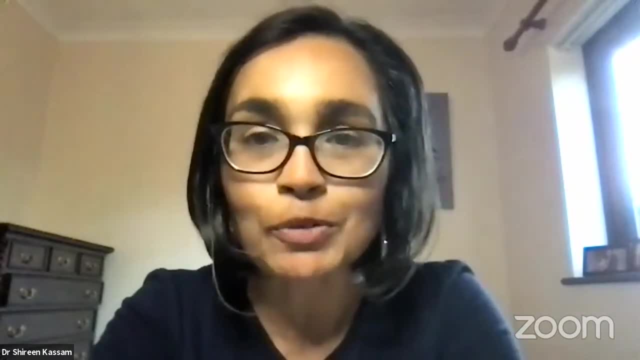 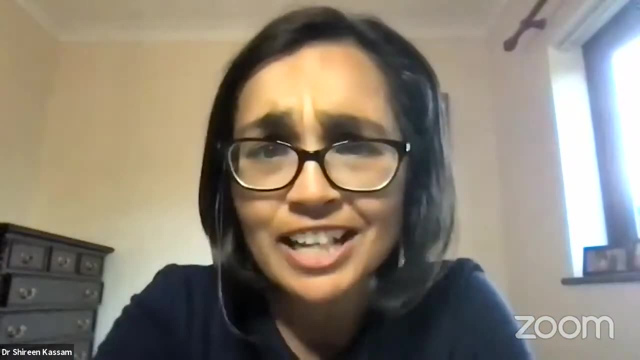 and it includes malignant conditions and non-malignant conditions, So inherited things like sickle cell anemia And then, as I say, all the way through to the blood, And then kind of the dull everyday things as well, like anemia and low or high blood. 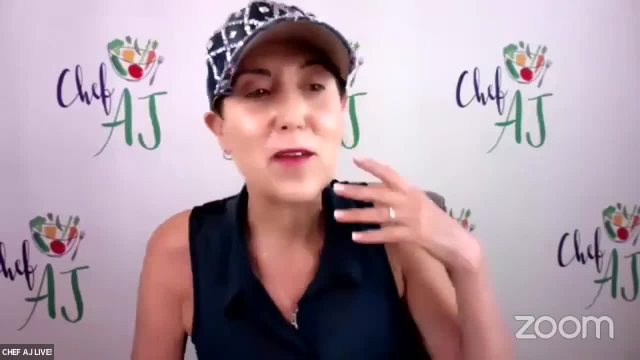 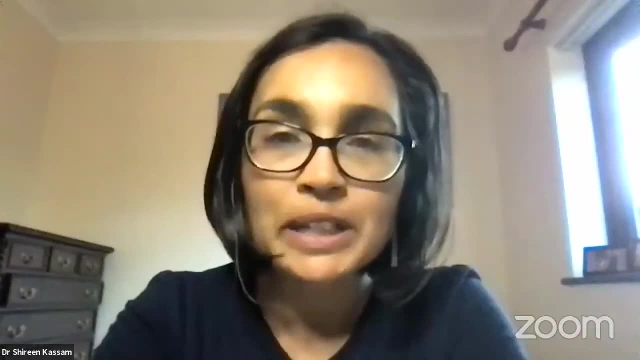 counts Right. So generally it's not like an eye doctor that you just kind of see regularly. You probably have to have a condition to see you. Hopefully we won't need to see you. Yes, it's a hospital-based specialty that requires a referral, But we sort of have our fingers in lots of different specialties because the blood system sort of gets affected by so many underlying conditions like even pregnancy And children in cancers and other conditions. Would you see all ages of patients then I personally only see adults. But yeah, I could have chosen on my training to become sort of more. 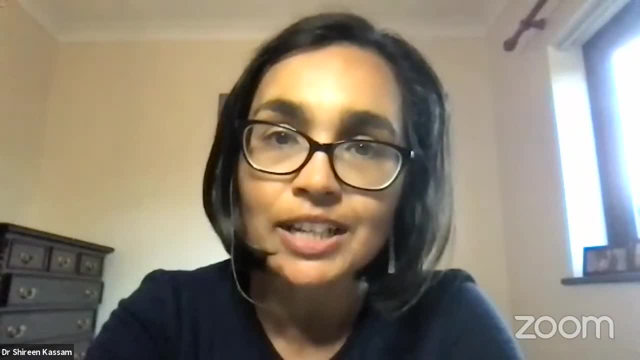 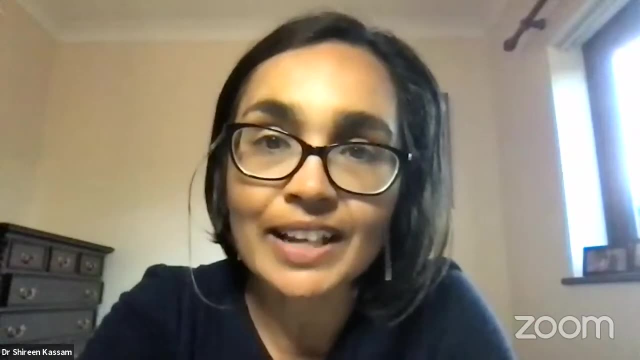 pediatric-based, but I'm an adult hematologist. I'm guessing that you even see cancers then. Yes, So my personal specialty is lymphoma, which is a cancer of the lymphatic system. So, yeah, Wow, Do you ever tell your patients, hey, consider a plant-based diet? This could help you. 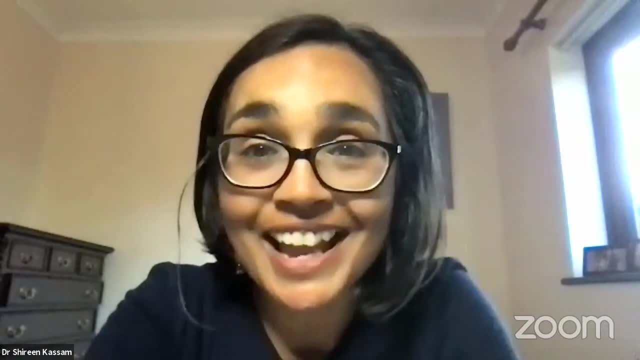 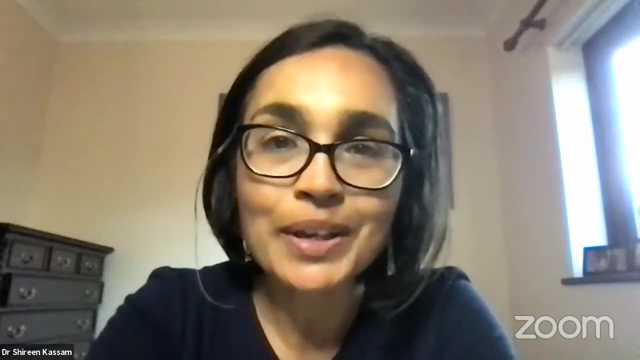 Yeah, for sure, I mean. the one question that everyone asks me is: you know what can I do, doc? What should I eat? What about supplements? You know. so you do get the opportunity to discuss with most patients And, like all your guests say, you know, you meet the patient where they are. 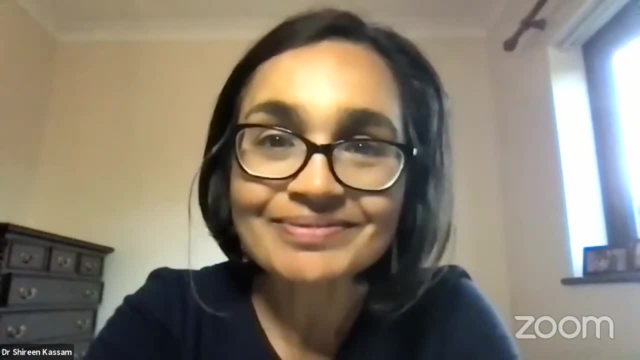 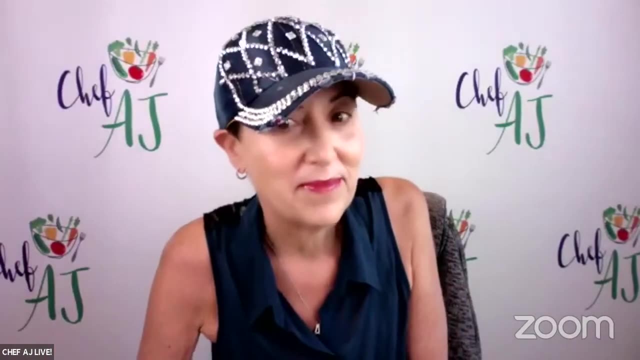 and help them transition to more healthy eating, as best you can. But if they have cancer, I mean, I agree with meeting people where they are, but when they're that sick, is there a way to get them to go further faster? It's hard, isn't it, Because you know you're giving somebody a life-altering diagnosis. 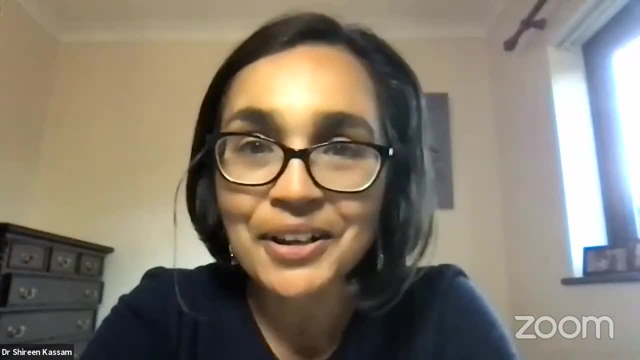 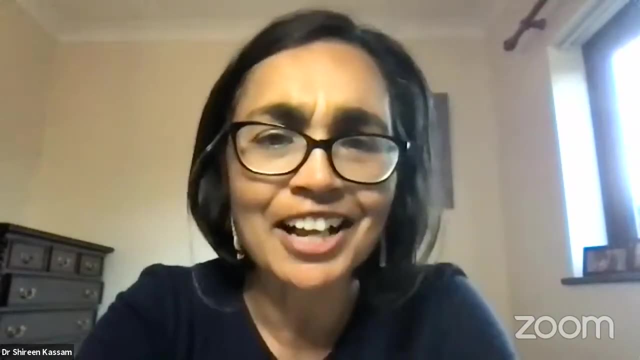 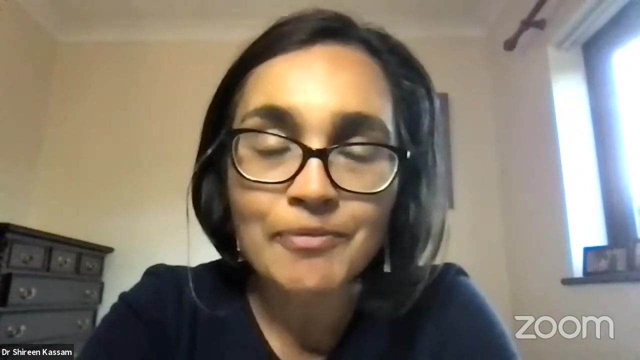 you're talking about chemotherapy. you're talking about, you know, changing their life and stopping work and financial insecurity. There's so many things to cover, So you really do need to have a person sort of centered approach. But yeah, everyone is up for talking. 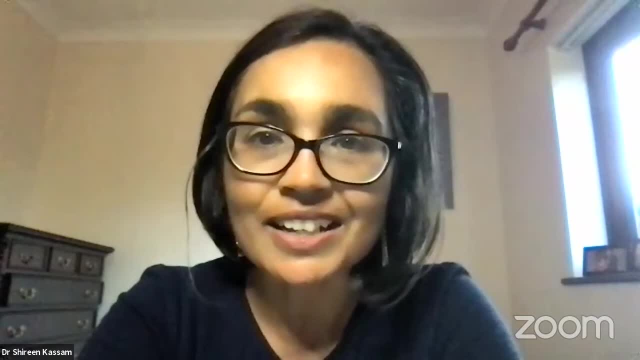 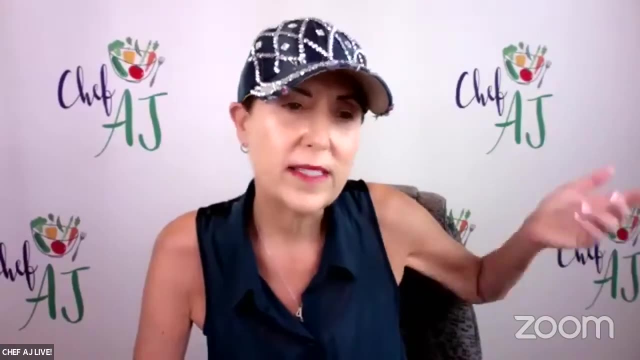 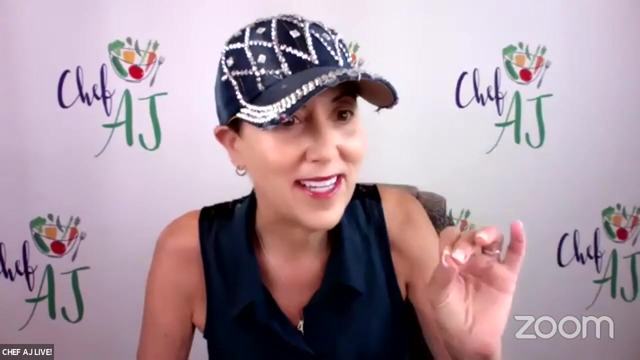 about diet interventions and exercise and other lifestyle interventions. I have known so many people that not necessarily family members but just people like acquaintances, co-workers throughout the year- That have had various cancers And they've said their doctor said diet has nothing to do with it. You're sick, eat whatever you want. 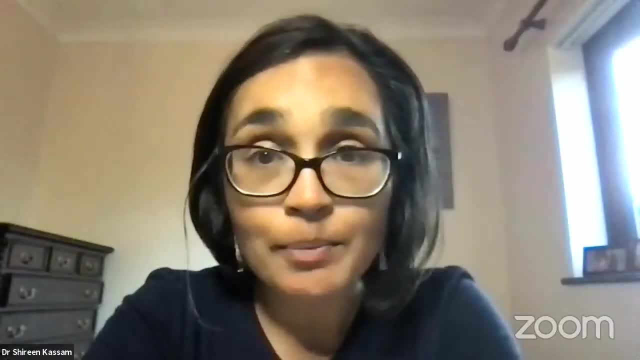 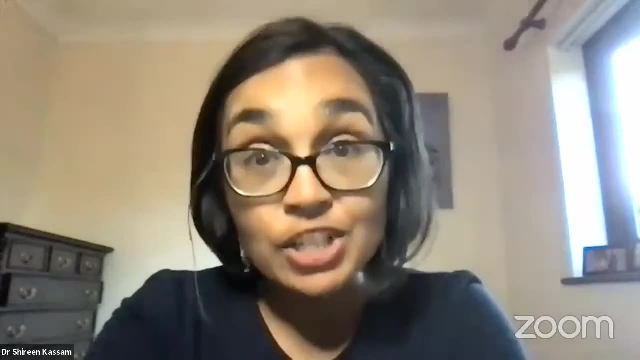 Yeah Well, it's a tough one. So you know, for example, in my specialty with lymphoma, it's not really related to diet and lifestyle per se, but the issue I face is a lot of my patients come to me, you know, middle or older age with all the other comorbidities that we're 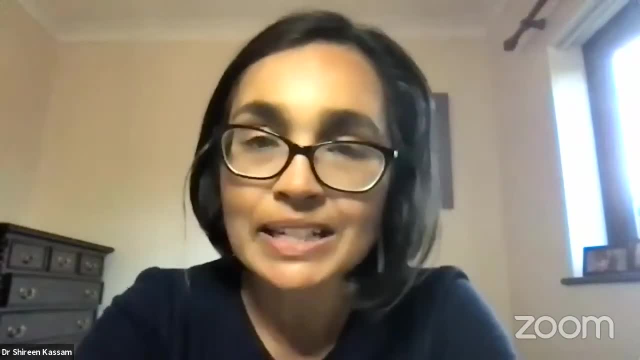 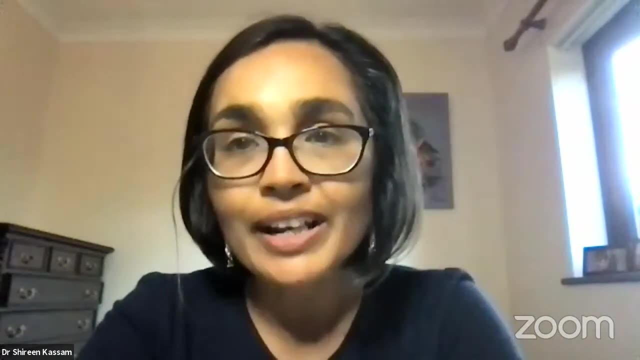 so used to seeing in primary practice. you know the high blood pressure, the diabetes, et cetera that really it really does make my life a little bit difficult. You know you're more at risk of the side effects and you know we're worrying then about long-term side effects of the treatments we give. 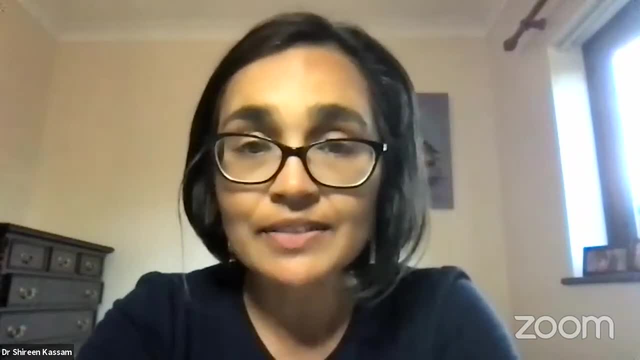 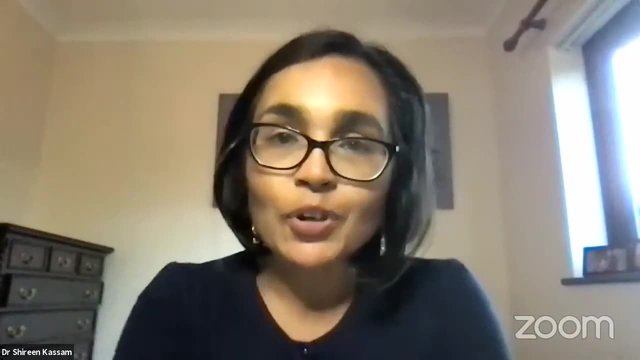 as cancer doctors, which obviously affect the heart and increase the risk of second cancer. So it is hugely relevant. But you know we come back to the same point that many of your guests will have made about our, you know, very, super, super specialized interest. You know we don't 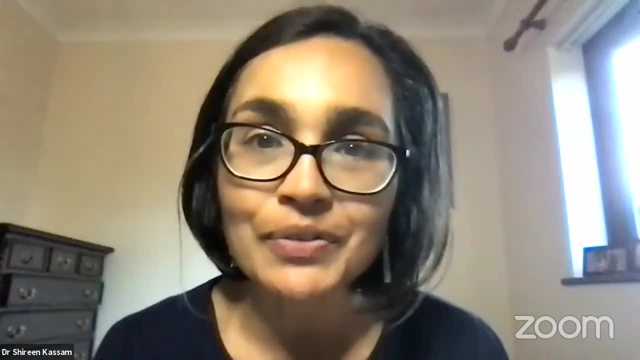 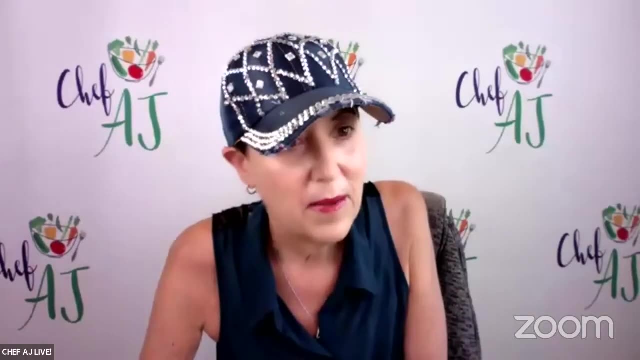 necessarily see the whole picture, but I think this explosion of sort of lifestyle medicine physicians, I think is a really big part of the problem And I think that's a big part of the and professionals is hopefully helping to change that. When did you first discover the plant-based? 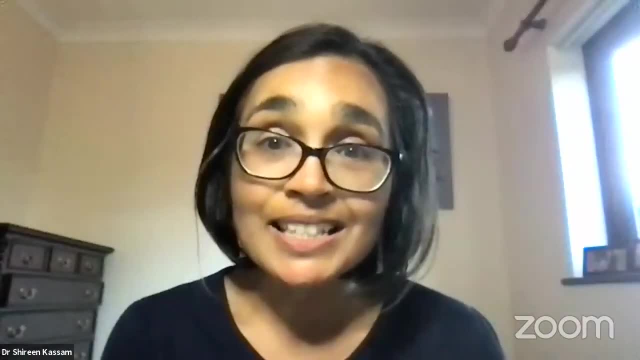 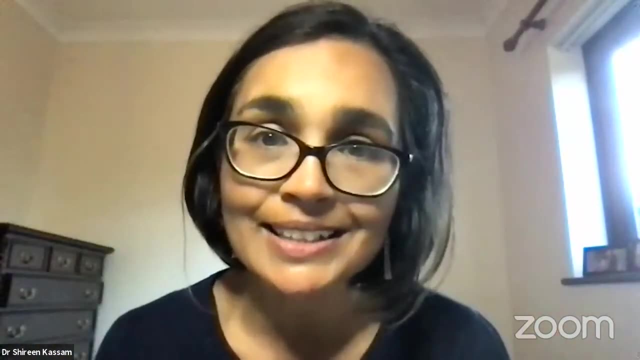 diet and transition to one yourself. Back in 2013,, I became vegan- for the animals predominantly. I'd been vegetarian since 2001, but suddenly realized that clearly, eating eggs and dairy was no longer aligned with my ethical or moral beliefs. And then, you know, I started looking into, you know. 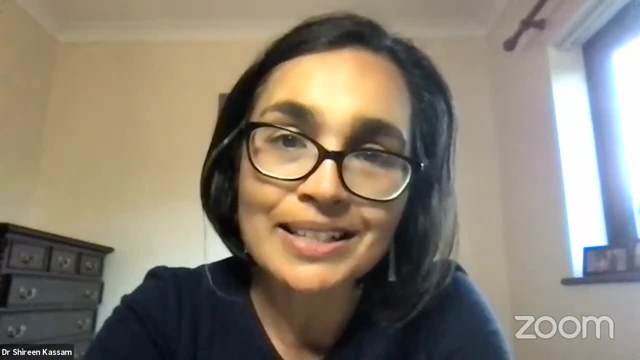 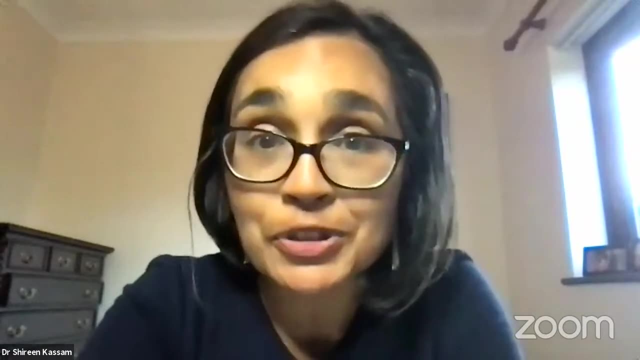 what should I eat? How should I be healthy? And came across all this amazing information about the potential health benefits of being on a plant-based diet and spent a good sort of three, four years educating myself, mainly out of, you know, the education coming out of the US. 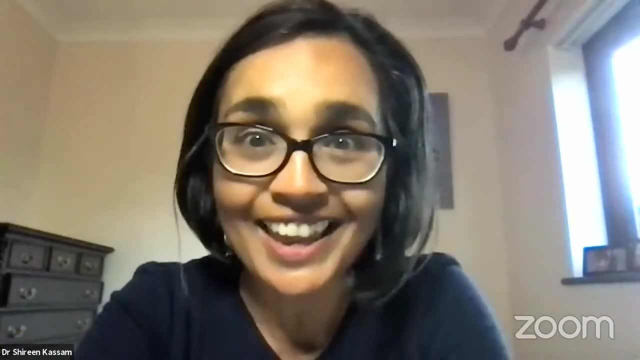 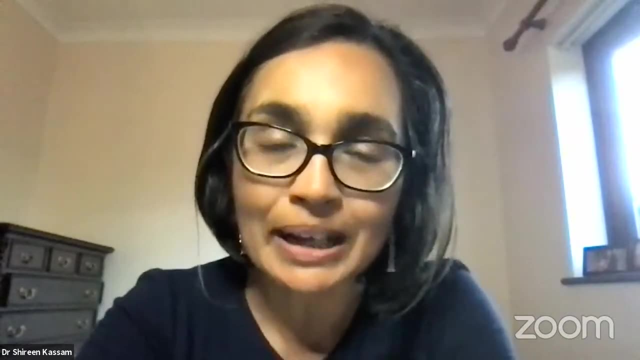 and then realized: well, what's happening in the UK? There's nothing here, There's no big organization really teaching people how to adopt a healthy, plant-based diet. So that sort of started my journey back in 2017, 2018 to create an organization that would do that. Tell us about. 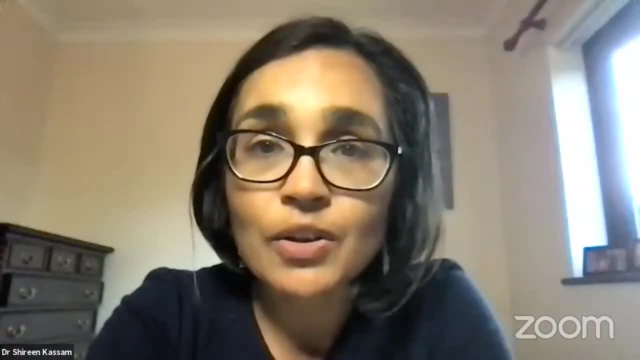 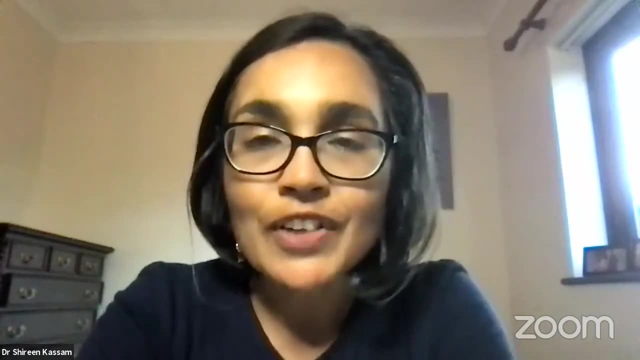 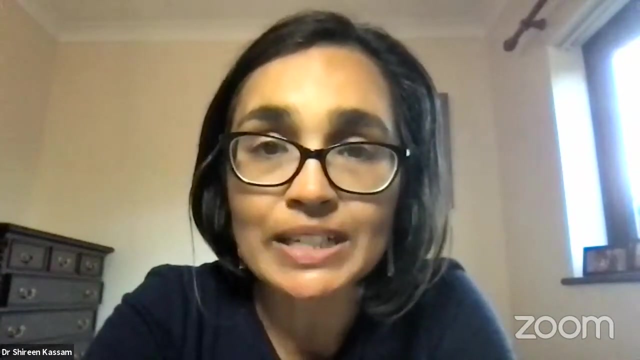 that organization. Yeah, thanks Thanks, Chef AJ. So I created Plant-Based Health Professionals UK in 2018.. And we sort of tested the water sort of earlier in the year. We launched our first conference on plant-based nutrition aimed at healthcare professionals in March 2018.. And that drew, you know, over 200 people. It was. 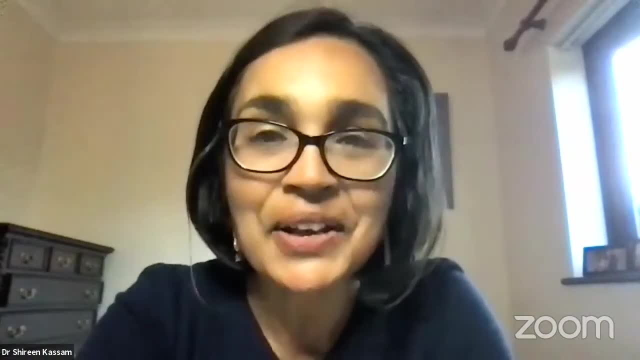 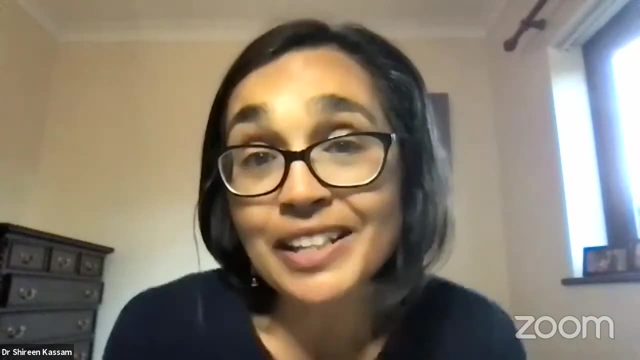 a sellout And I thought: well, you know people are really interested in this. So once the conference was over, you know it made some good connections. We set up a community interest company That's really gone from strength to strength really due to the hard work of all our wonderful 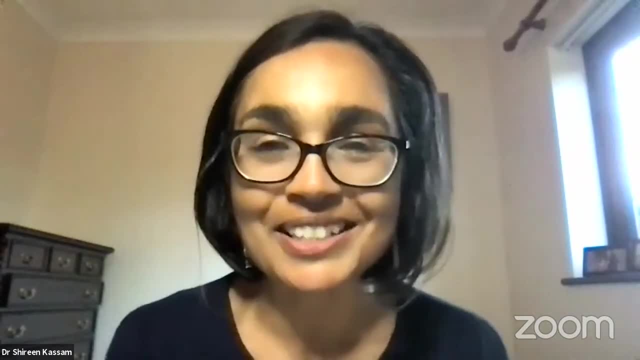 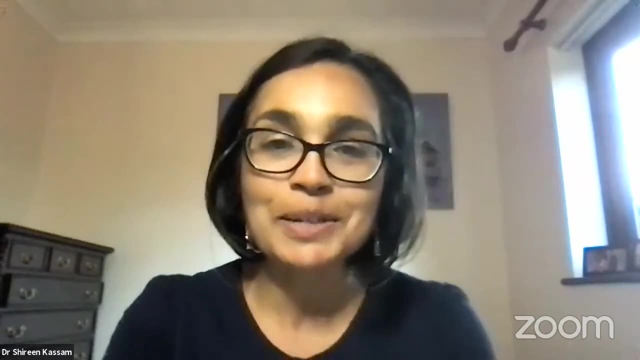 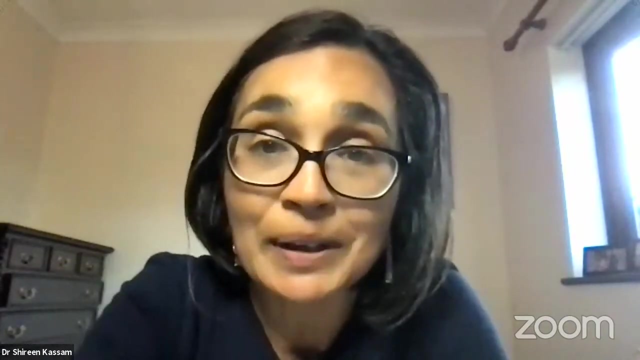 team members that I hope you get to meet at some point to as well. So we basically modeled ourselves on PCRM because they're such an amazing organization. So we were just wanted to bring all of that education advocacy to the UK And so hopefully we've started our journey but got. 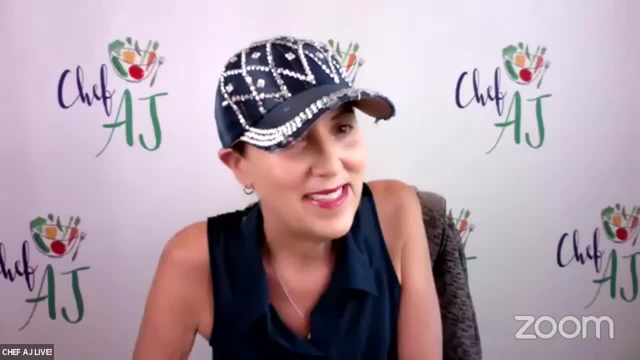 several decades on which to catch up on. I love that. the PCRM of the UK. How many team members do you have, And are there any that you've worked with? I think there's a lot of people that I've heard of. Are they of different specialties? 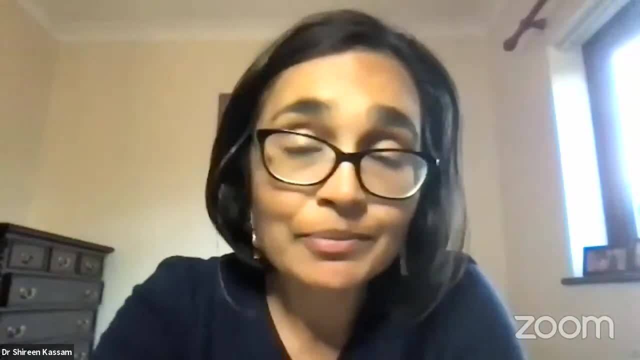 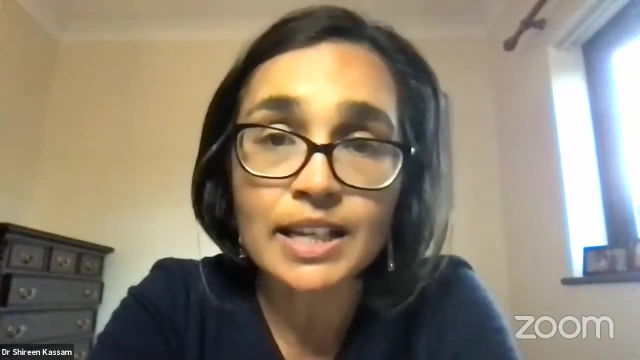 Yes, absolutely So. we're multidisciplinary. You know, we have a membership organization that include everyone from general public to any healthcare professionals, specialties and nurses and dietitians, nutritionists and, of course, doctors as well, And our core team. we're small. 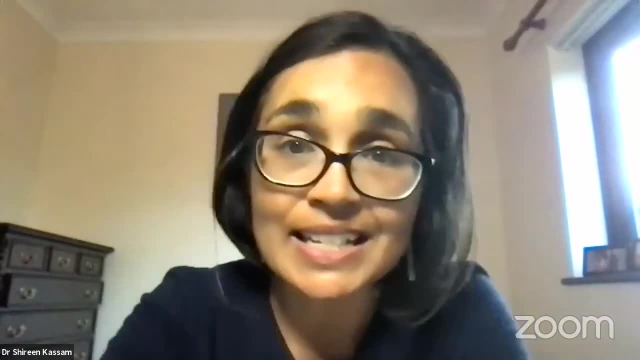 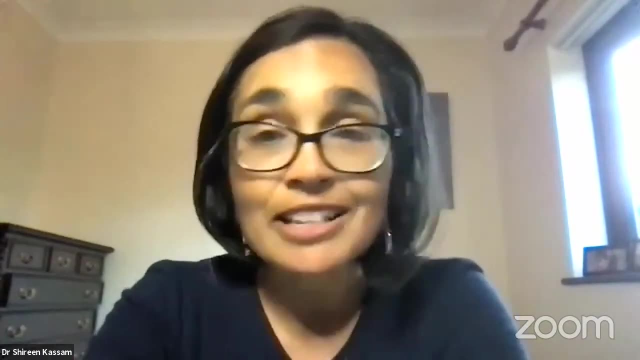 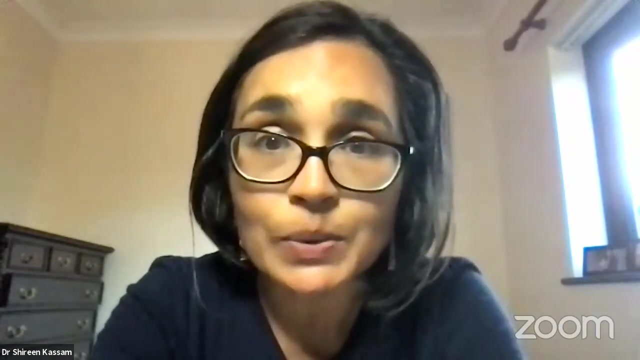 still, but we have Rohini Bajaykal, who's our communications lead and nutritionist and she runs our webinar program. We have Leila Dakin, who is our education lead, So she does works on the articles, all our sort of fact sheets that doctors can download, And she's created the 21 day plant. 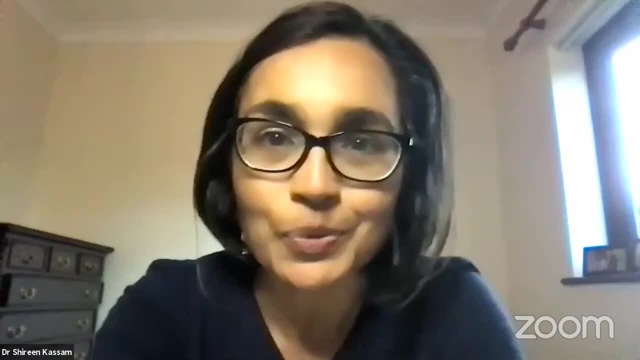 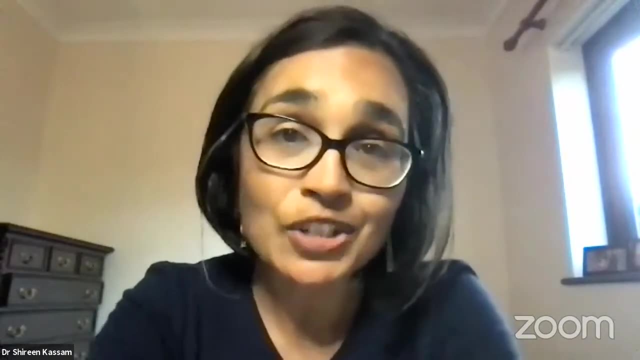 based health challenge, a bit like the PCRM, but sort of UK version with all the doses and concentrations of various nutrients that we recommend over here. And then we've got Laura Freeman, who's a GP and lifestyle medicine physician, who's created plant based health. 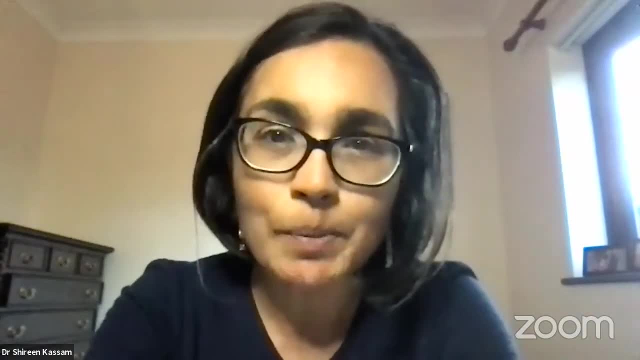 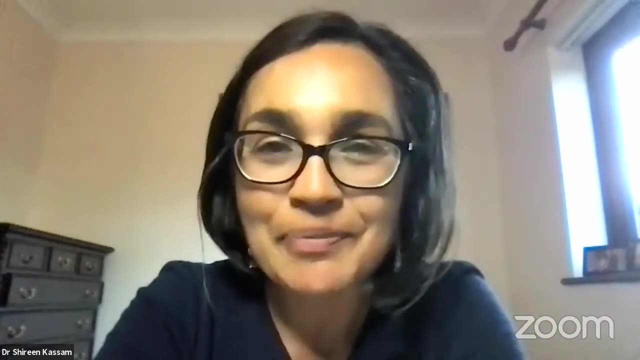 online, which is our sort of healthcare service. It's a bit like your plant based telehealth in the US, And we sort of nicked their idea- with permission, of course- And it's an online service where people can book an appointment with a plant based professional. 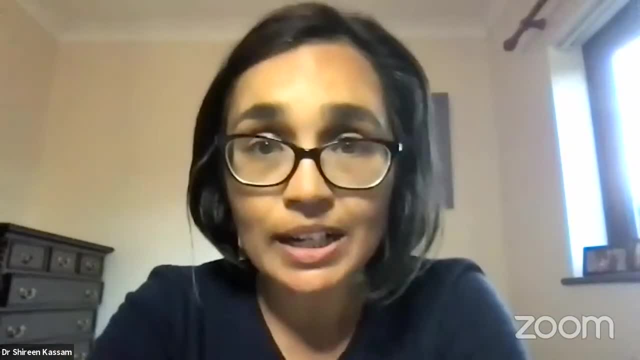 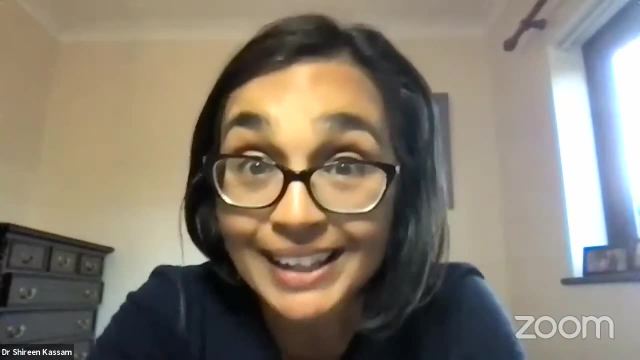 whether it's a doctor, a nutritionist, dietitian and you know- have a more holistic approach to their healthcare, should it be for reverse and type two diabetes, surviving cancer, those sort of things. And we've got Hayley Tate, who's a chef and an author and a GP, And she's bringing 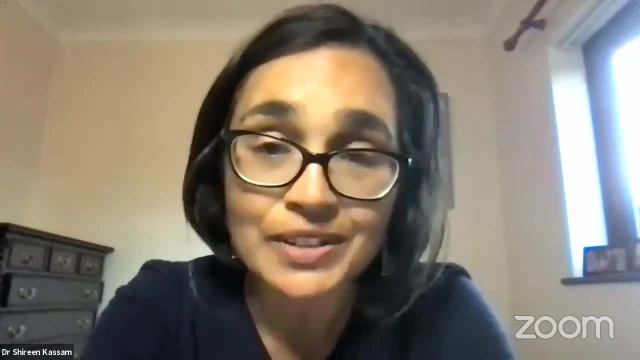 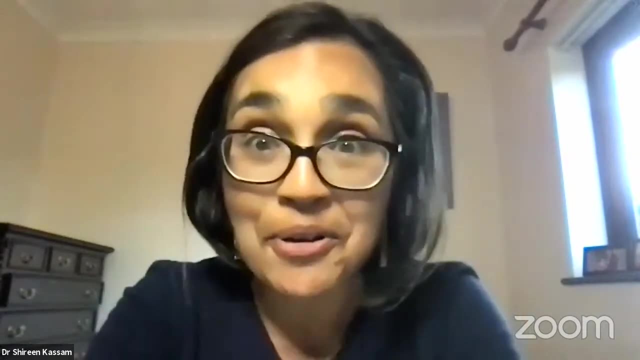 our cooking to the climate course, hopefully to medical students. So we've got some medical schools signed up to to that for the coming academic year And, yeah, we can go on and on. lots of little projects and amazing team members and our ambassadors you've met already, So you've. 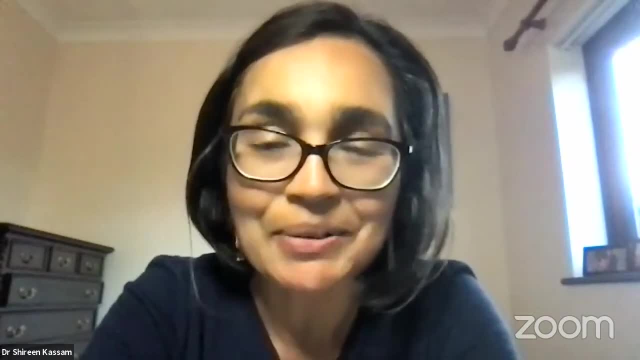 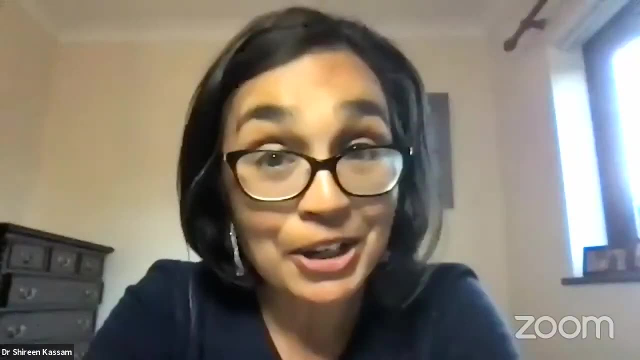 met Gemma Newman and Alan Desmond, who've been working with us for a while too. Well, it sounds like you have enough people for me to do a week devoted just to your organization. You really could actually So, if you're up for it. 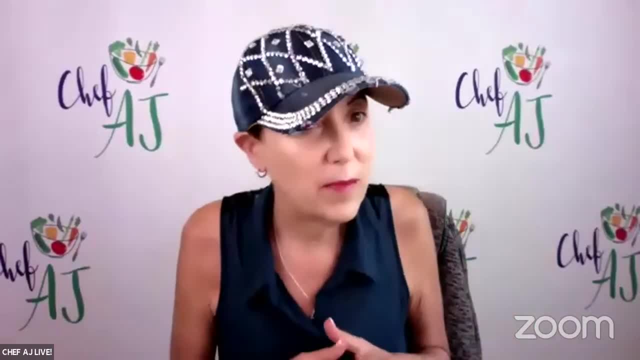 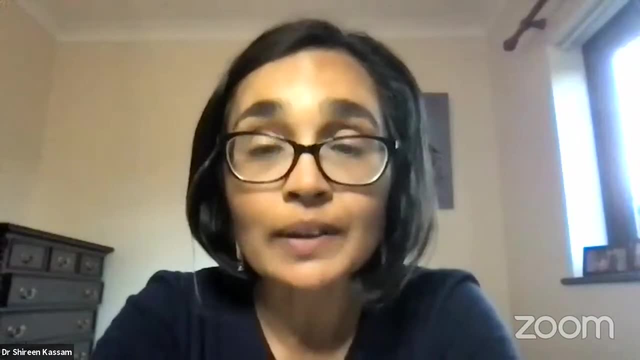 You could co host it with me. So are most of the people that find out about your organization or join in. Are they living in the UK Or are you more global? Yeah, well, we. this year we seem to have become more global, And I think you know. the one of the good things of the pandemic is that we have 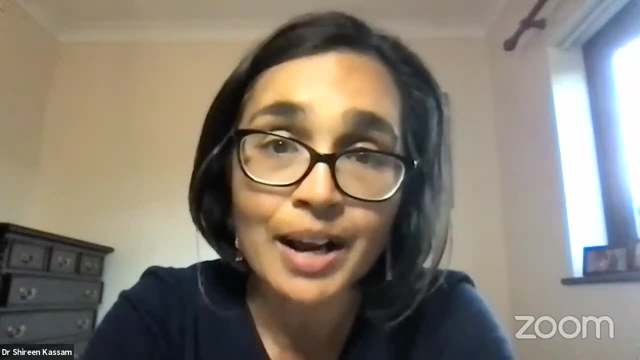 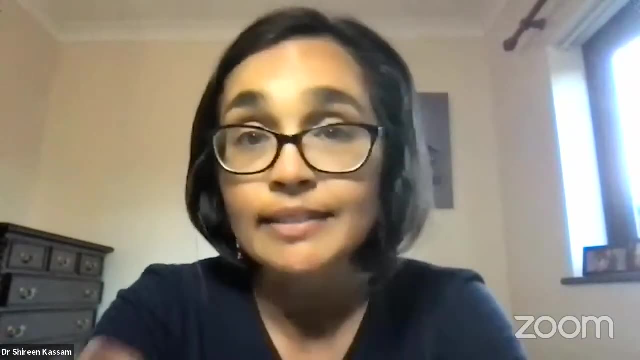 been able to connect a bit more on online and our webinar program, which is free at CPD accredited- it's accredited by the ACLM, So people with a lifestyle medicine certificate can get more CPD from that. So we have had more international members for sure. So we've got some from the US. 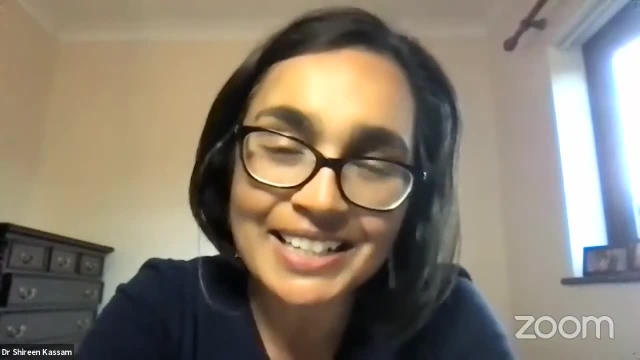 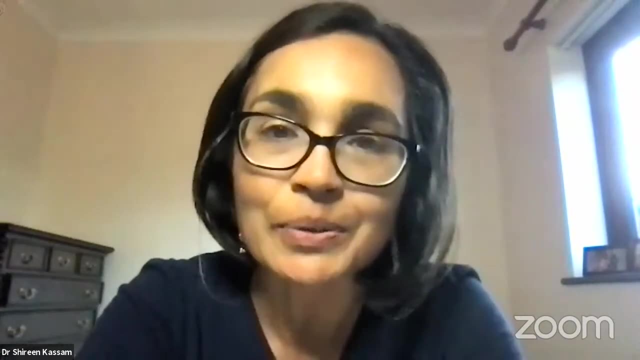 and Australia, And I have spent time over the last two, three years connecting with sort of the counterparts and the different organizations around the world, like Doctors for Nutrition in Australia and obviously PCRM and what have you So. So yes, we have got international members. 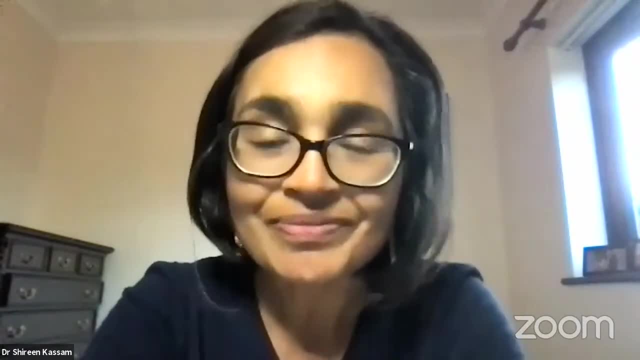 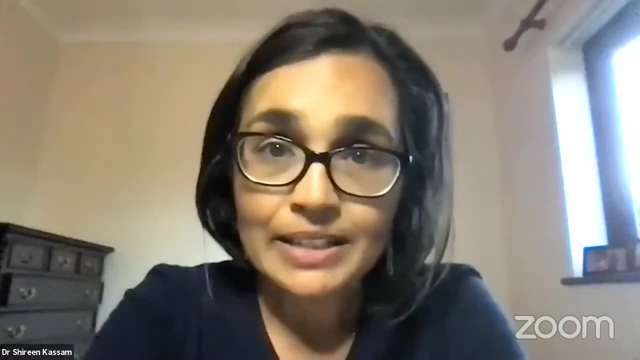 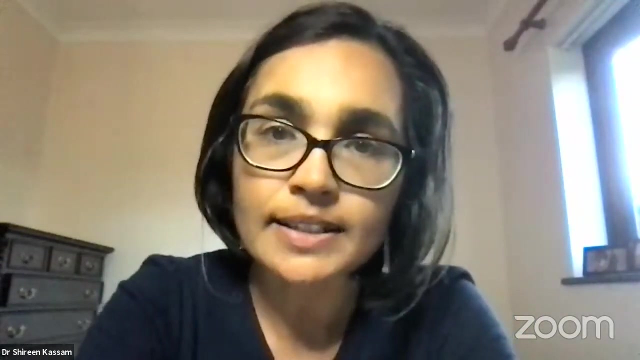 which is wonderful because you get different perspectives And the people have a consultation- if they're not in the UK- with the, with the professionals. Yes. So for plant based health online, it's available worldwide with our dietician and nutritionist- not necessarily with our doctors per se, because our licensing is slightly different. 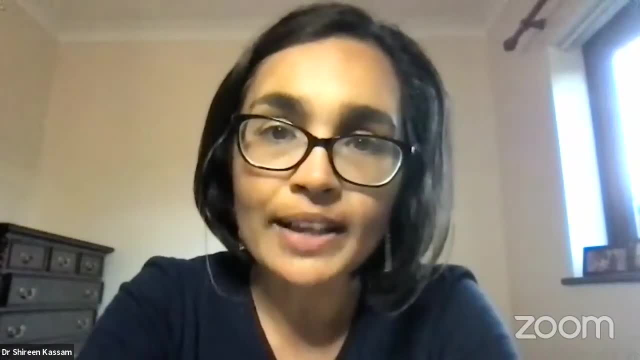 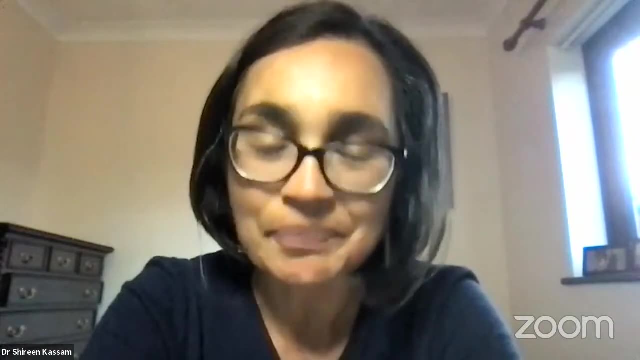 in that way, But- and we're not- we're not covering US and Canada, since that's so well covered by plant based telehealth, But otherwise, yeah, we're available globally. Wow, What about this course that you created? Tell us about. 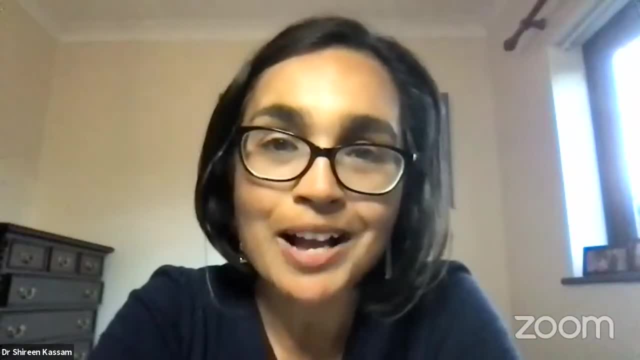 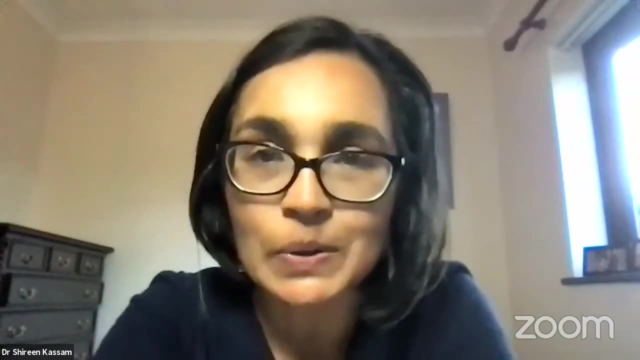 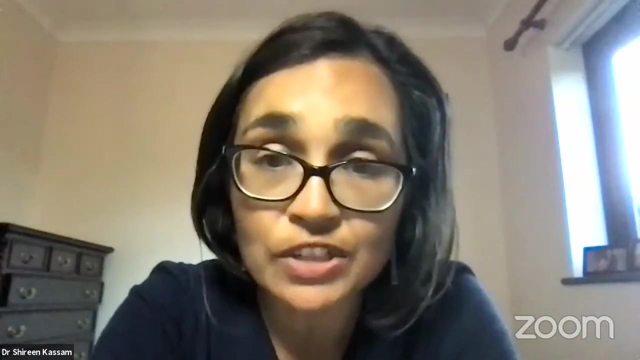 Yeah, so that that happened a couple of years ago. I've always tried to tell people sort of infiltrate the conventional systems and kind of get into universities and medical schools, and it was fortuitous really: a friend introduced me to the then Vice Chancellor of Winchester. 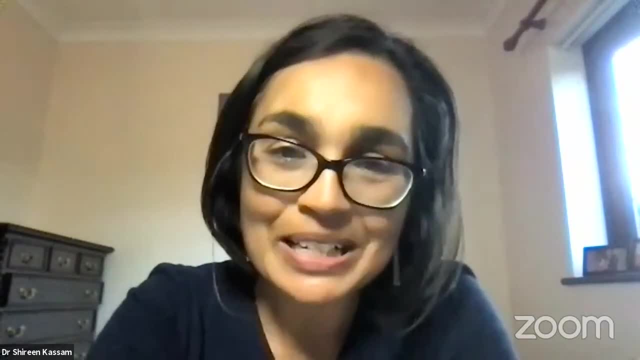 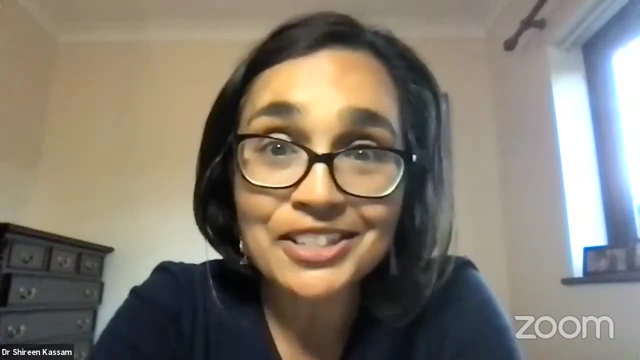 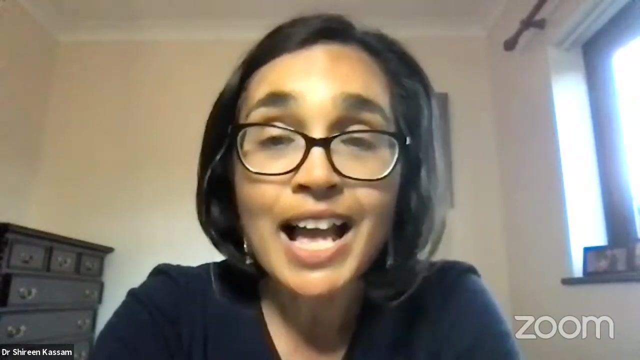 University who was vegan, And I went to meet her and I said: well, you know, you're creating a faculty of health and well-being at Winchester University, so you need to be teaching people about plant-based nutrition. nobody is doing it in the UK, certainly not one that's directed towards healthcare professionals, and there they 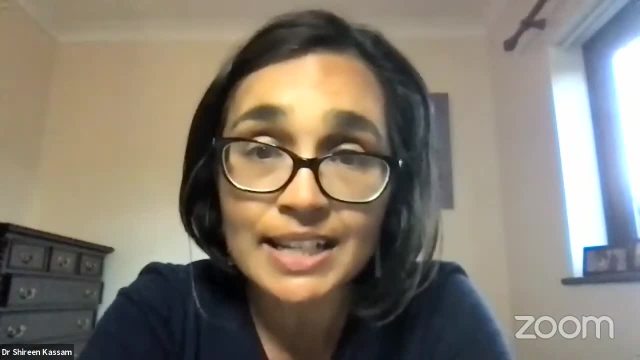 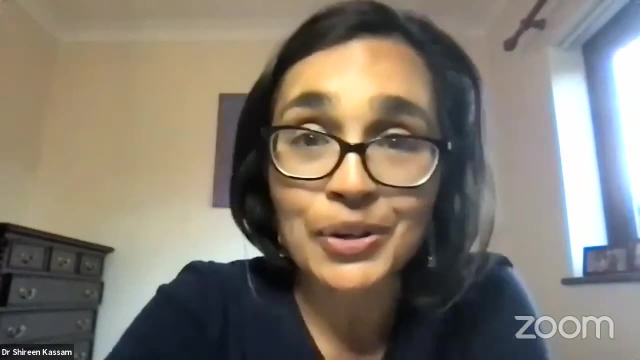 were, you know, going to start nursing and physiotherapy and dietetics as degree courses. so I didn't hear anything for a few months and then suddenly, you know, through the post, got an invitation to join the faculty and create a course. so I've been able to offer a plant-based 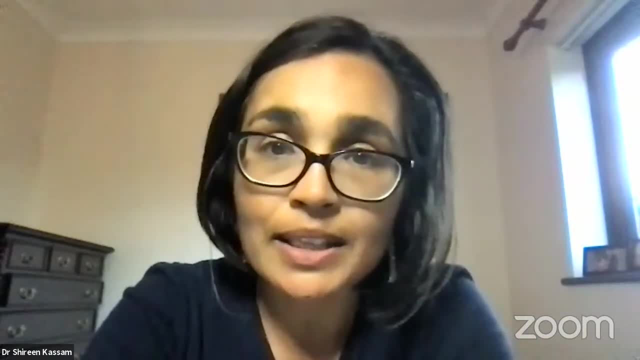 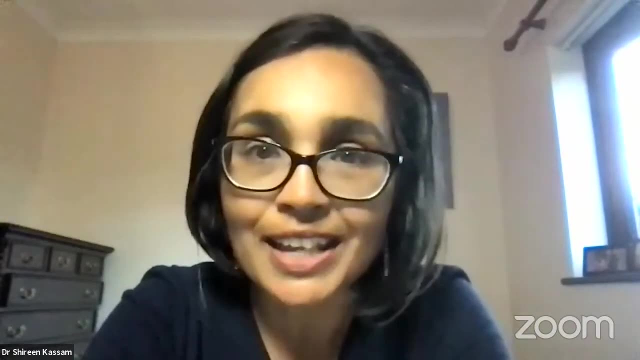 nutrition certification, which is again accredited by the Lifestyle Medicine Societies here in the UK and the US. and yeah, we've been running it for the last two and a half years now with my colleague, Leila Dakin and we've it's been a great success actually, lots of people coming through learning 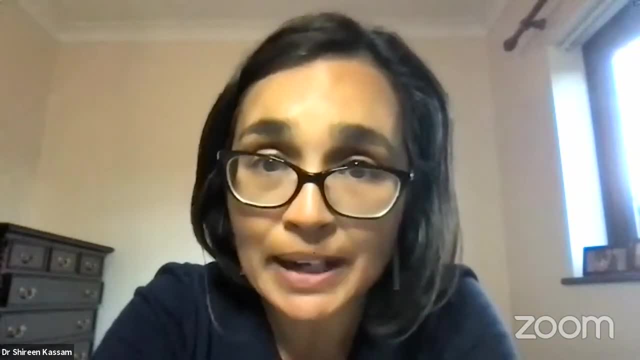 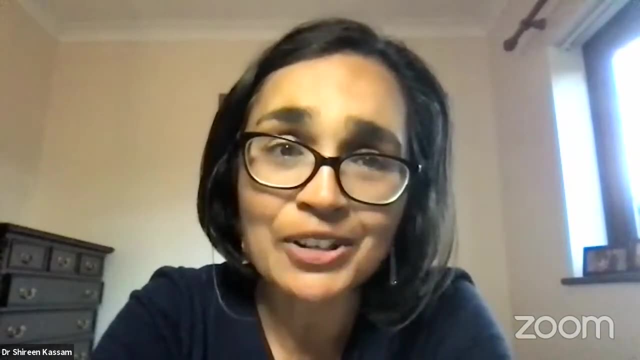 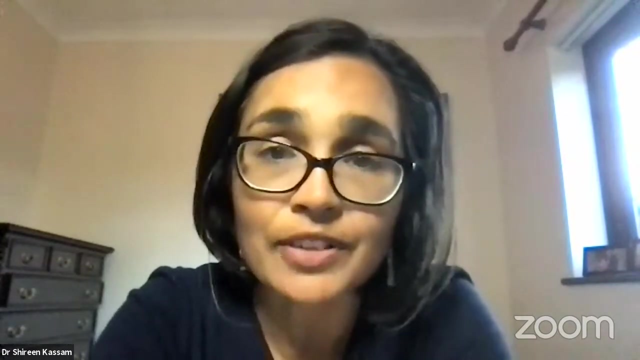 about plant-based nutrition and, you know, exceeded expectations really. I don't think Winchester University thought it was going to run it for more than a couple of sessions, so that's been really good to see and that really is available globally to everyone who's looking to sort of get extra CPD for their, for their. 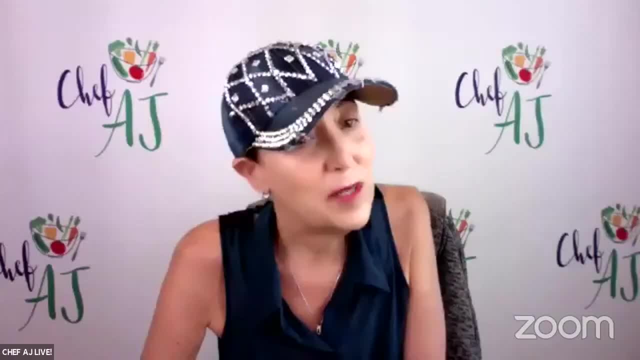 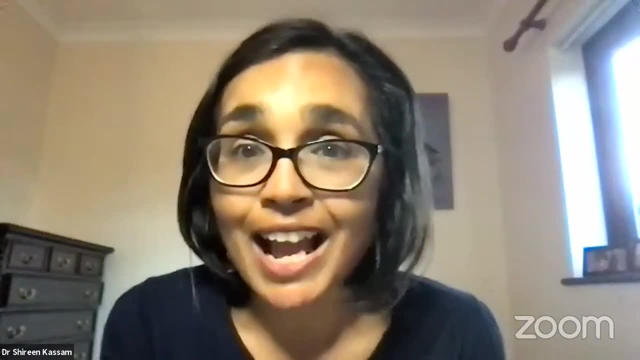 appraisals and careers and just general knowledge. Is it similar to the T Colin Campbell course? Yeah, so I mean I've done that course of you know, naturally when I was first starting out and it's wonderful, I guess, from what I remember, because it was quite a while ago, I guess mine's quite 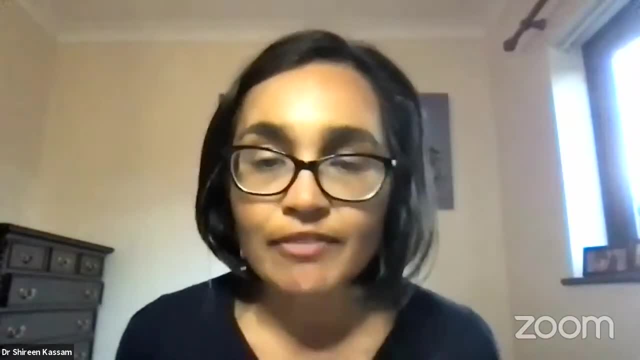 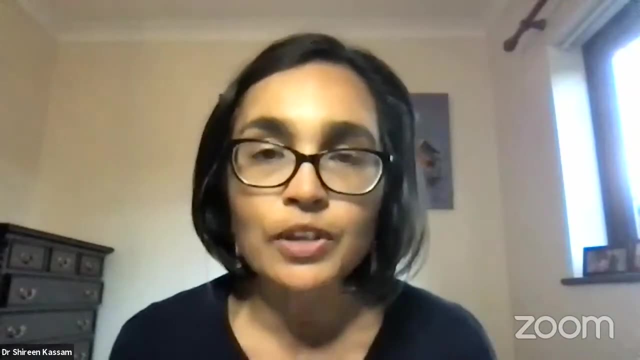 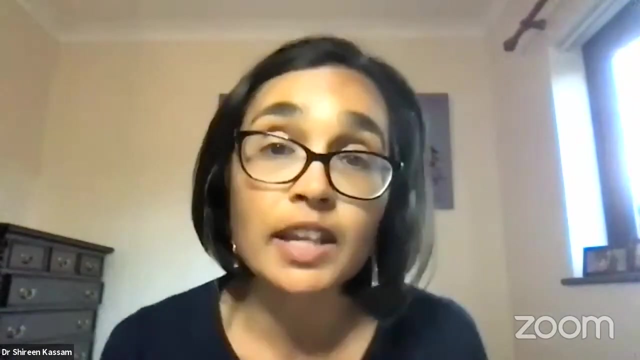 in-depth science. It's science-based, you know, and it also is covering quite a lot of the different sort of plant predominant diet patterns, you know, going into Mediterranean and DASH and all those sort of things. so perhaps a little bit broader perspective. obviously got a UK focus rather than the US in. 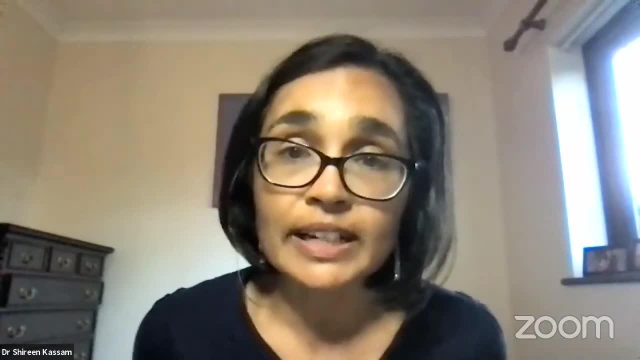 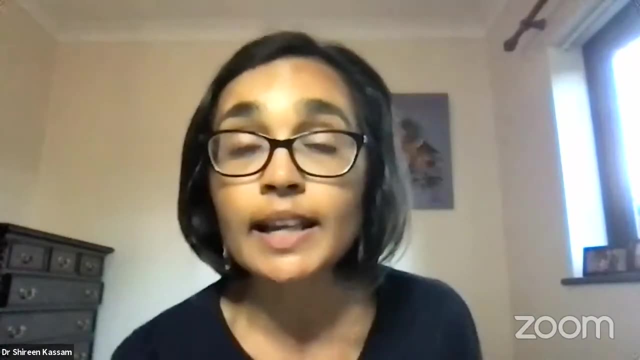 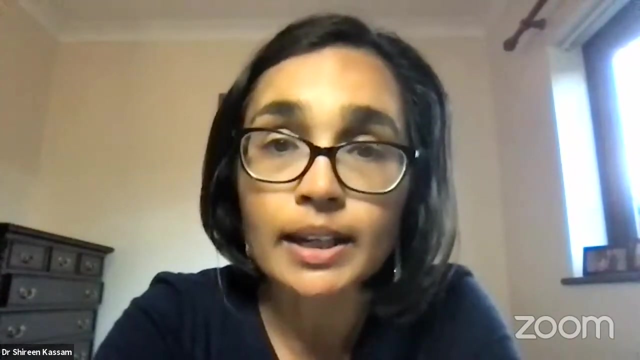 terms of sort of our healthcare system and things and a really deep dive into a lot of chronic disorders and including paediatrics and pregnancy and things like that. so there's overlap for sure, Sure, but it's sort of created with healthcare professionals in mind. So who are the people that normally take the course? Are they lay people? Are they professionals? 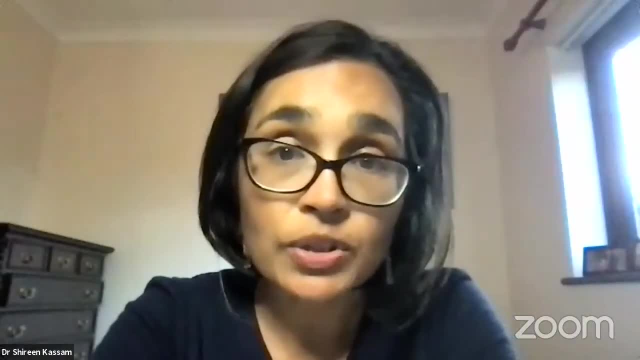 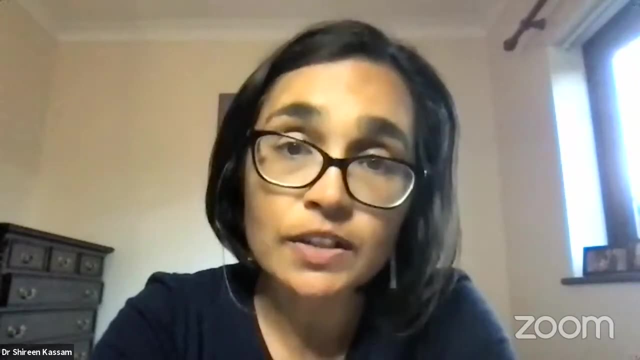 Are they mostly in the UK? Yeah, so again a mixture. two-thirds, I think, have been healthcare professionals, so doctors, GPs, predominantly so primary care, and dietitians and nutritionists, and then sort of more sort of holistic healthcare practitioners. you know well, chefs, of course, because you're healthcare. 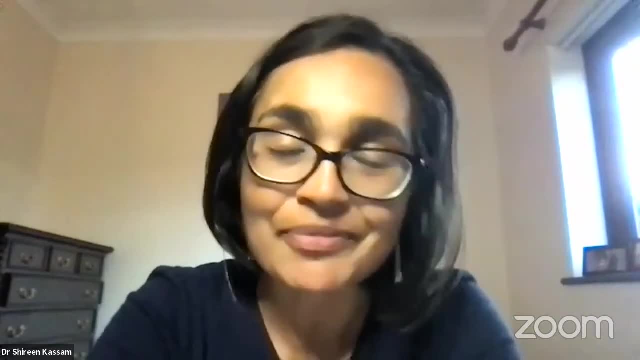 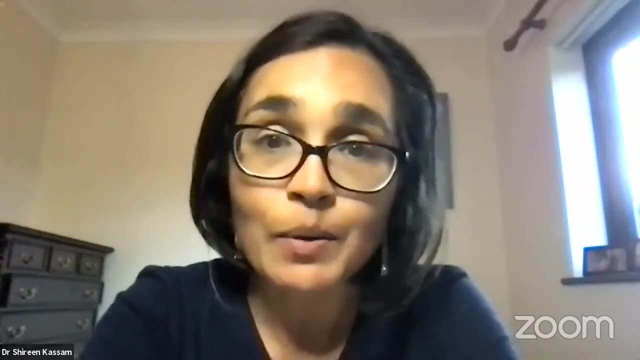 practitioners as well in a way Nutrition- sorry so, yoga teachers, pilates, that sort of thing. but yeah, general general public and those that are sort of at that level where they want to take it a bit further have definitely taken it and enjoyed it and given good feedback. 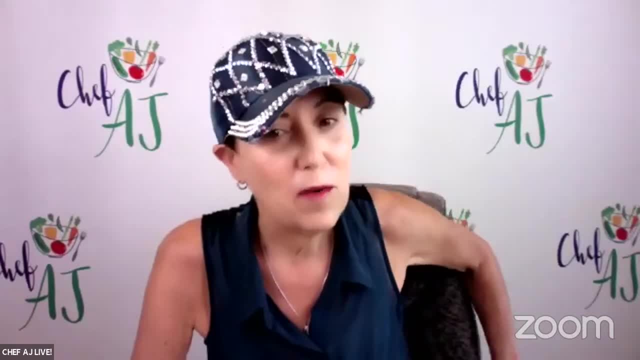 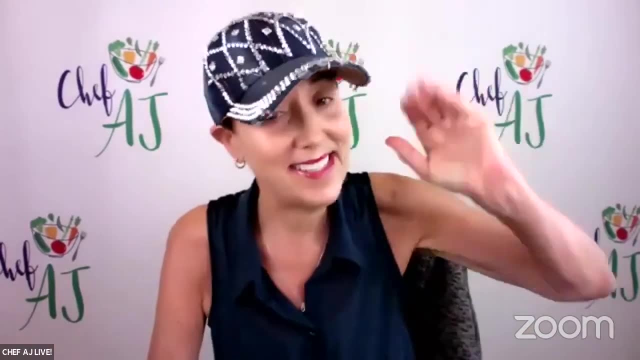 I love these online courses. I was just teaching in Mexico for a week and I had some spare time and I finally took the Dr John McDougall Stark certification course and I love that and I passed the test- Wonderful- Not a hundred percent, but I was- but I did pass. so if you don't mind this, 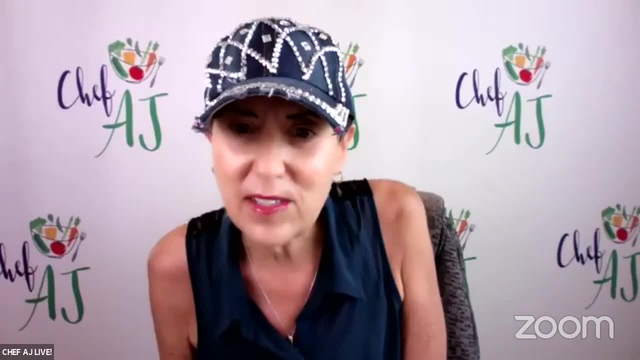 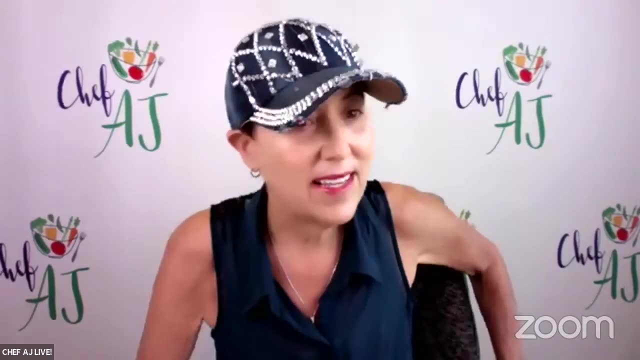 There's a question from Crystal, who's watching live, and she says her best friend's son has some kind of a blood disorder that he has to be very careful not to get cut. What is that called, and is there anything that can help? Oh, I see. well, it could be a number of disorders or underlying conditions that make you bleed too much and they can be inherited or they can be acquired. so it's a little bit difficult to say without knowing the actual underlying condition. so it could be a coagulation system or the platelets and, as I say, could be inherited. I mean, you know, I get, I guess. 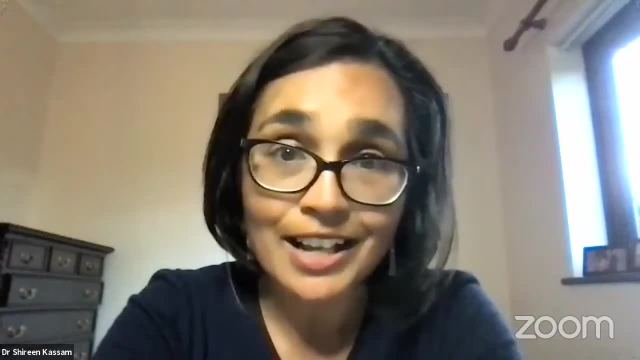 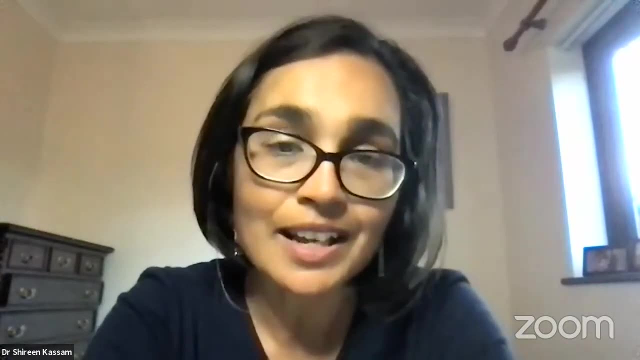 we all need to have, you know, good nutrition to have a normal blood count. and you know the the usual things like b12, folate and iron play into having normal blood counts. but I you know that without more detail it's a bit difficult to be specific. 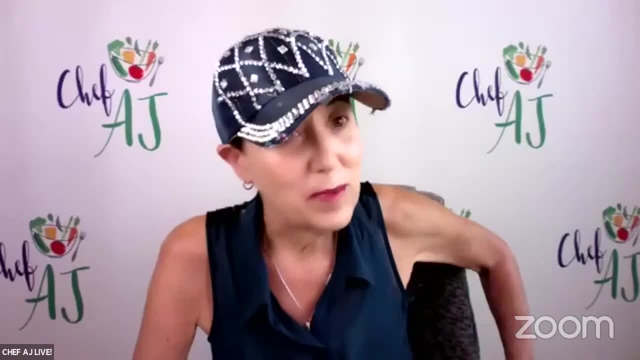 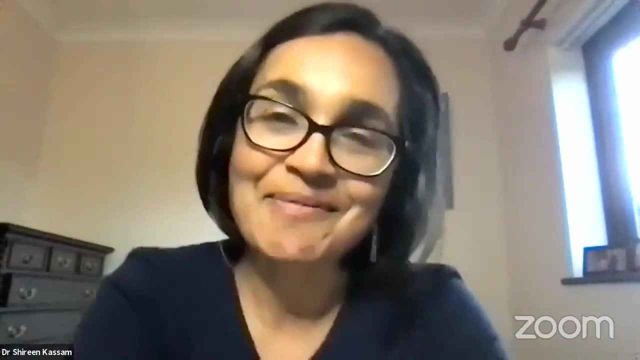 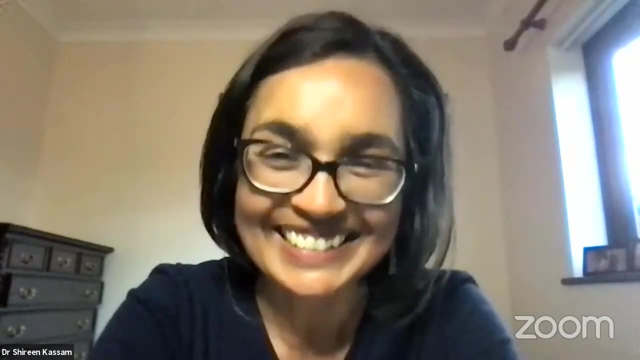 Thank you. You mentioned before we went live that your husband's also a hematologist. Is he also a plant-based hematologist? He is, he absolutely is, and he's not the only hematologist I know who's plant-based. so I think we could have a mini subgroup of hematologists who are plant-based. That's good. What kind of? 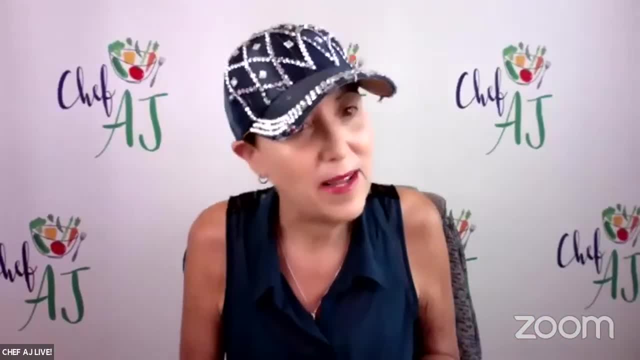 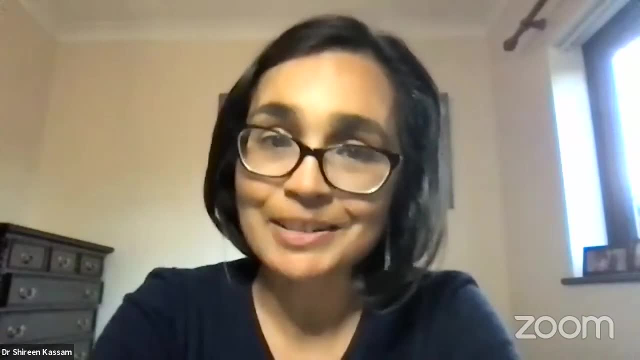 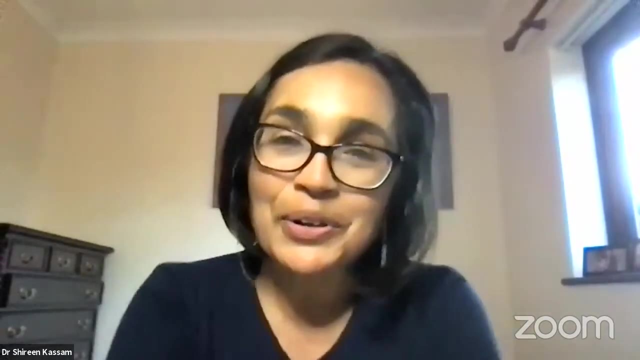 changes have you seen since going plant-based or in your patients that you've been able to encourage to go plant-based? Yeah well, I mean my patient at home, my husband, since lockdown has managed to really get back into good shape. It was the sort of kick he needed to, you know, lose. 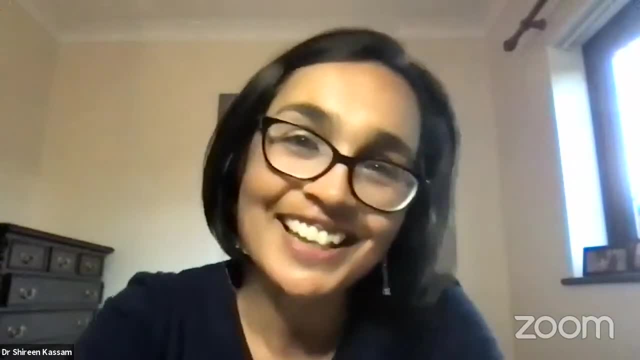 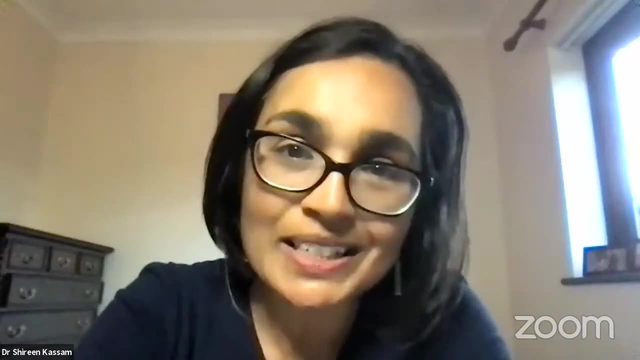 weight. so he's lost a good two stones and got fitter and brought his cholesterol down and things like that, and it's interesting because he was already vegan before that. so really upping the quality of the diet and going properly whole food, plant-based- was the thing that he needed. 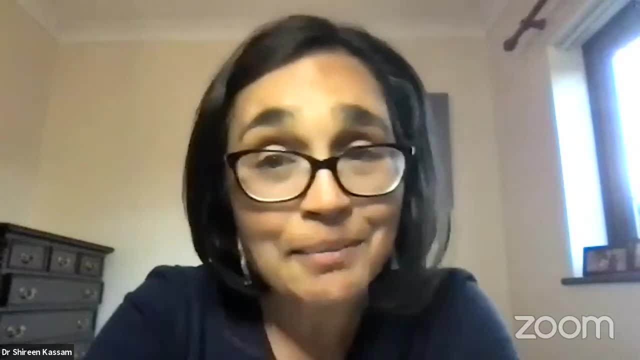 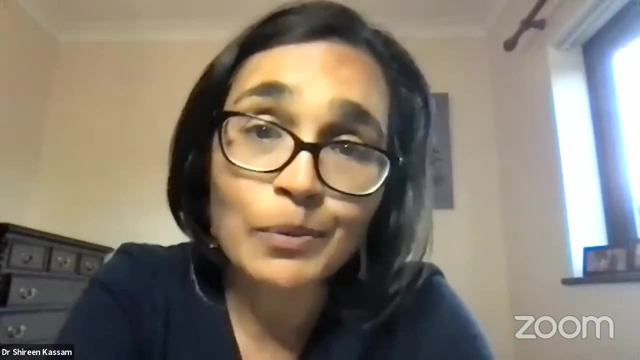 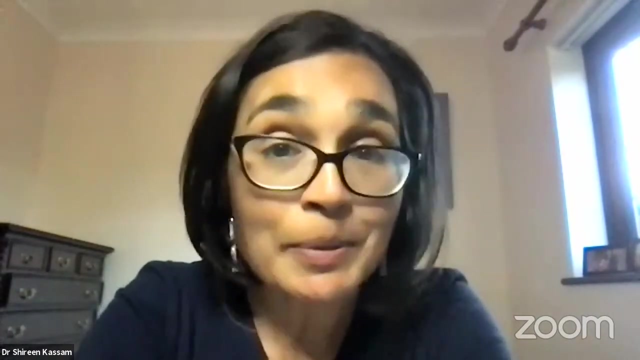 at the start of the pandemic. so that's been nice to see. and my dad was actually diagnosed with pre-diabetes at the end of last year. He's previously had a Whipple operation and, you know, had a third of his pancreas removed. I thought, oh gosh, well there's no hope. but actually, with a bit of upscaling of the quality, 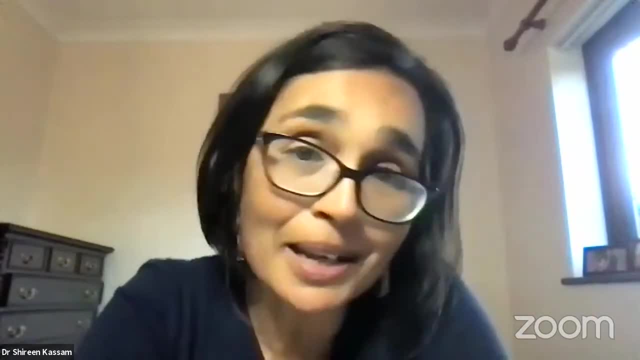 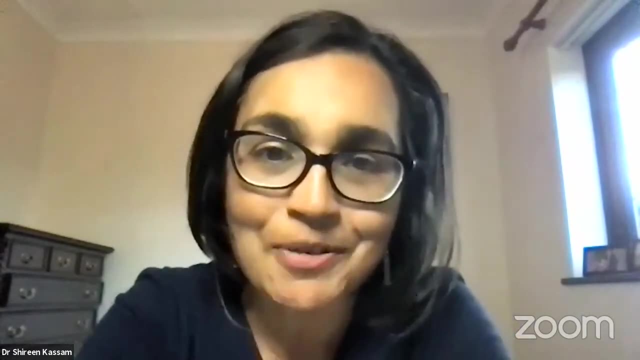 with one of my colleagues on our team, Rohini Bajaykal, who's been able to reverse that too, so that's been really nice to see. It's nice to see that what you read in the books actually can work for your friends and family too. and then, yeah, in the cancer space in my 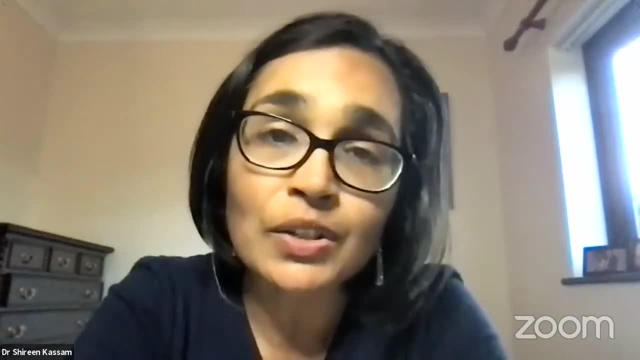 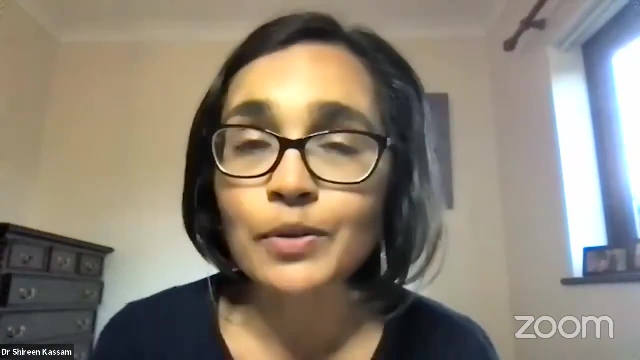 clinical practice. you know, just the usual things that you'd expect: people feeling like they've got more energy, that they've lost a bit of weight, their blood pressure comes down and those sort of things. it's a bit more difficult to track the longer term because we, if they, if people do. 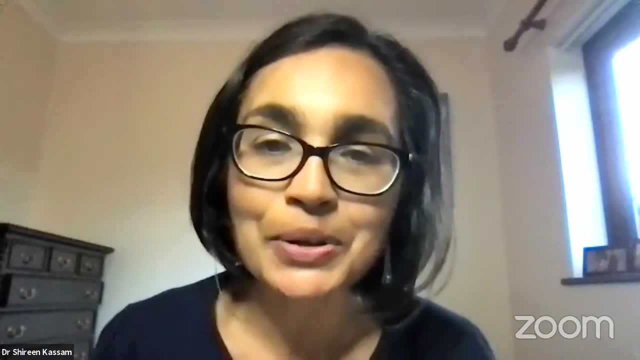 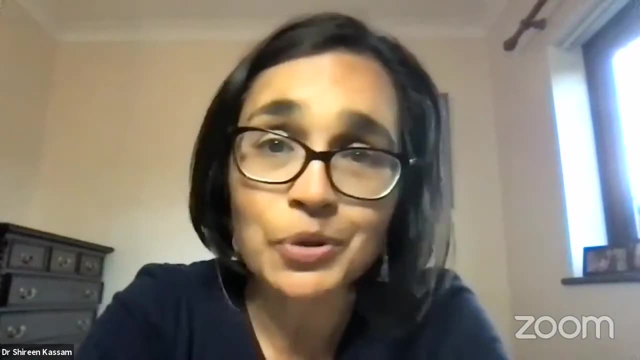 well, they kick with their kicked back out to primary care. we don't. we don't keep them in our clinics for years and years. but there's so much to be gained and, and you know, with cancer care, we know it's even part of all the guidelines to be more plant-based. you know when you want to prevent. 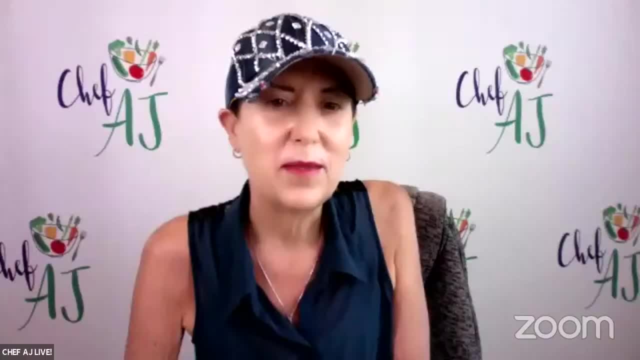 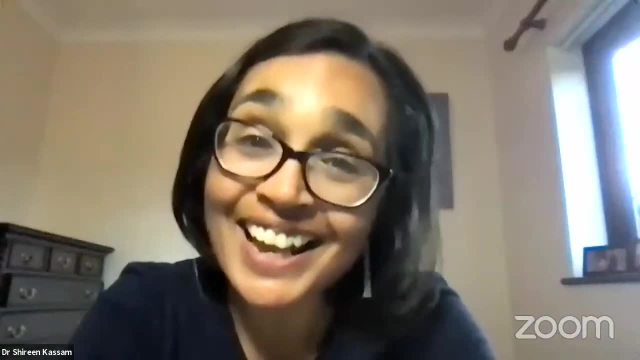 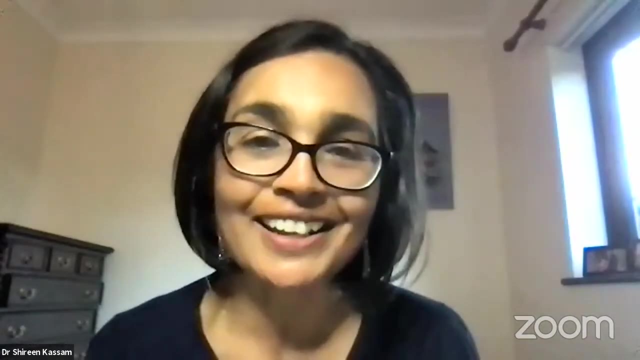 cancer, but also if you've had a diagnosis of cancer. Absolutely, Mari wants to know: do you know any plant-based doctors in Ireland? That's countries right next door, isn't it? Yeah, not far away. well, yeah, interesting, Yes, and if you look them up online and they're called plantbaseddoctorsirelandorg, so or I can. 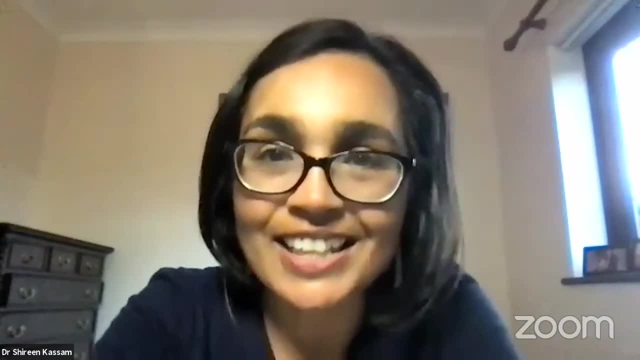 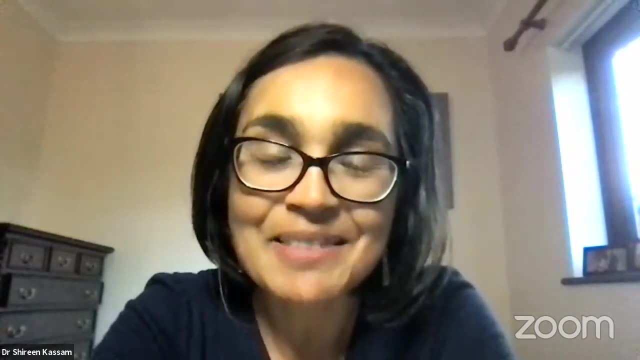 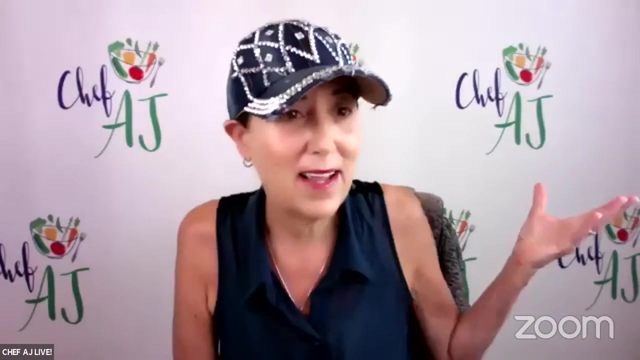 I can make sure that I send Chef AJ the link, but there is a small group of Irish plant-based doctors, for sure, and so yeah it's, it's coming to all four nations. That's fantastic. I love that. what you just took something that was successful here and replicated it, I mean, I think that'd be. 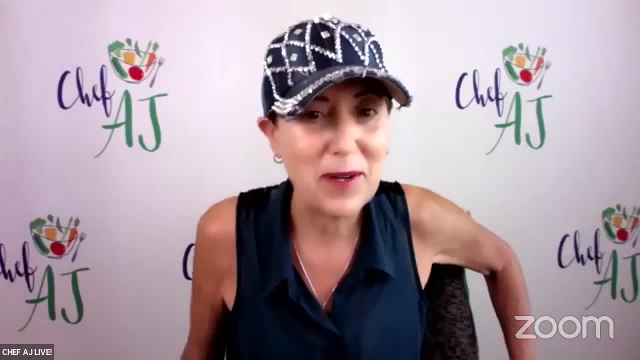 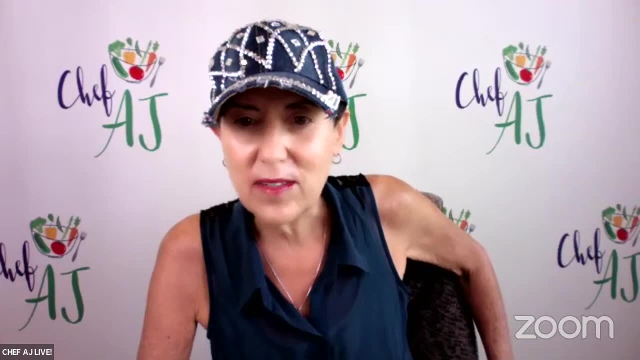 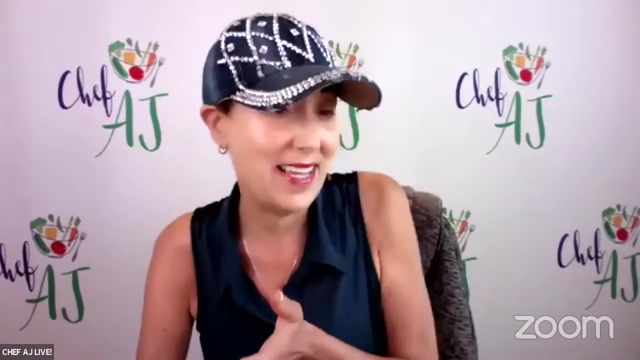 fabulous. if every country did that, you know you don't need to reinvent the wheel for this. so Susan says: have Dr Layla, the plant-based doctor of nutrition, on the show, as Dr Kassam mentioned. she's wonderful and focuses on nutrition and sports. of course I will. this is how I find my 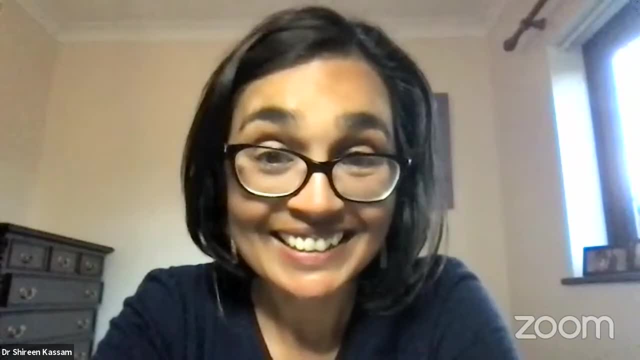 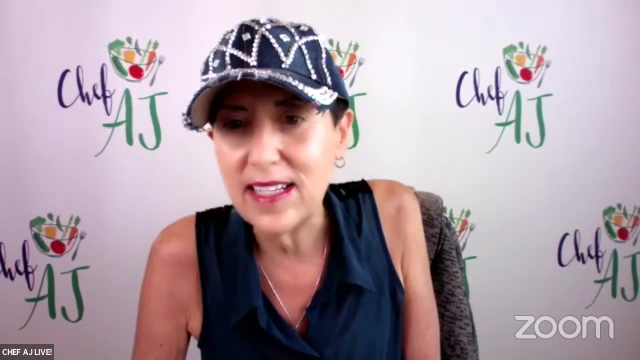 guesses from other. really I don't. I don't go to people unless it's referrals, because I don't like rejection when they say no. so she sounds fabulous. Jesse says: would you please ask Dr Kassam if she has seen an increase in cases of immune thrombocytopenia? 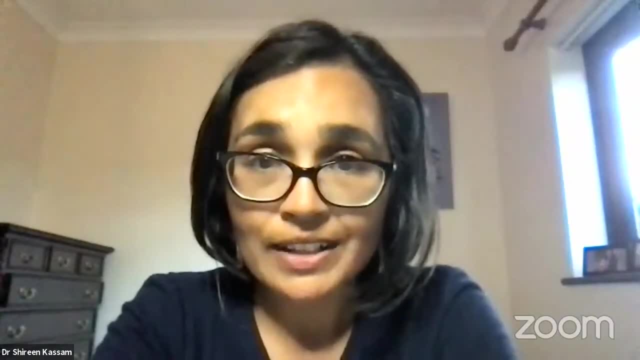 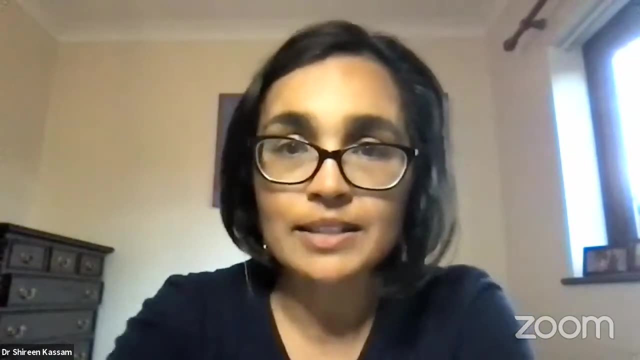 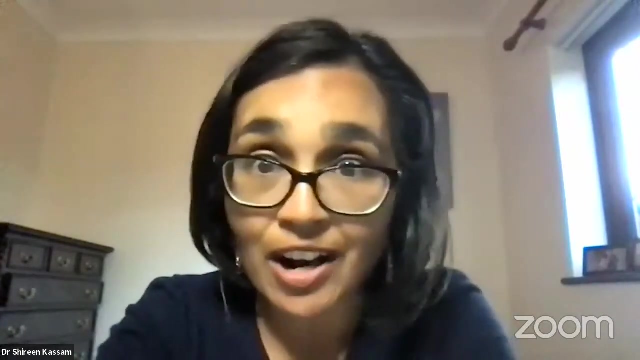 Is this related to COVID, do we think is? I suspect that's probably the link. I'll take it as that's possibly what the person is referring to. yeah, I mean, I think you know, in our practice we do see that any viral infection, whether it's Epstein-Barr virus, whether it's the flu, whether it's a, you know, bacterial- 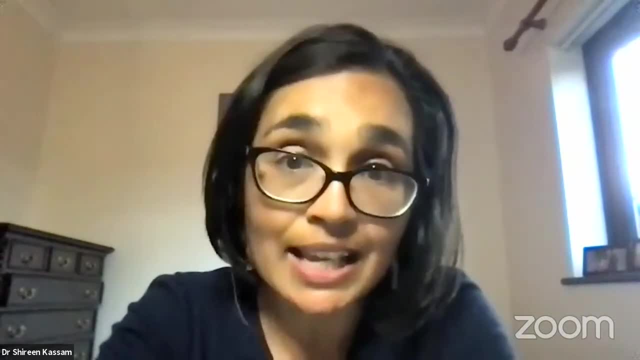 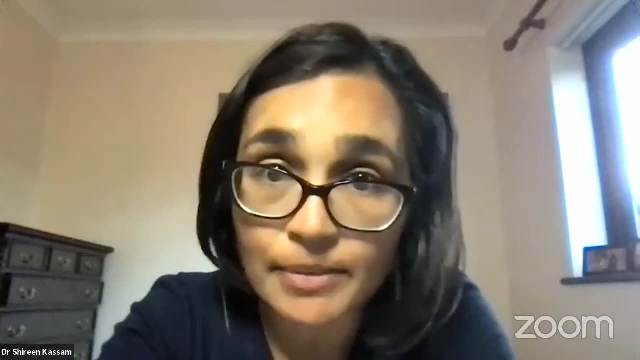 chest infection, the blood counts can take a hit and certainly ITP, or immune thrombocytopenia, is a complication of many viral infections and I don't think COVID has been any different, and obviously there's been issues with some of the vaccines as well, causing an. 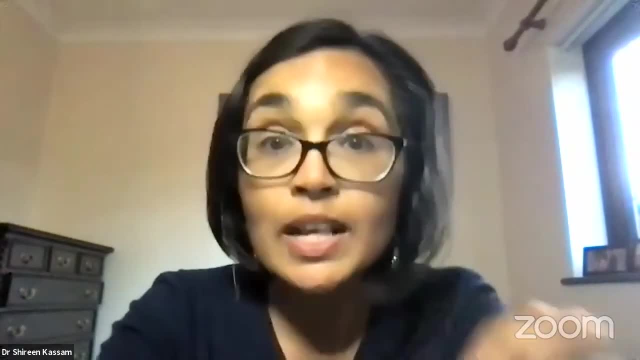 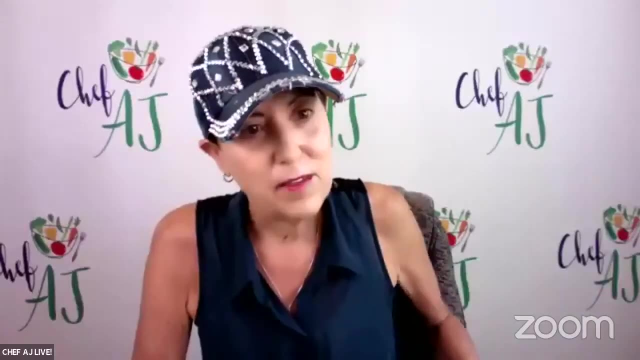 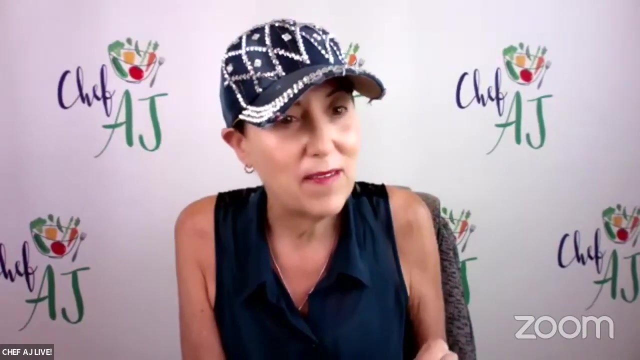 immune type thrombocytopenia. so yes, it has been sort of rare occurrences with both the virus and and the vaccine. You know it's interesting. I've done two weeks worth of show with doctors from India, some that are living in the United States, some not- and it was interesting that so many of 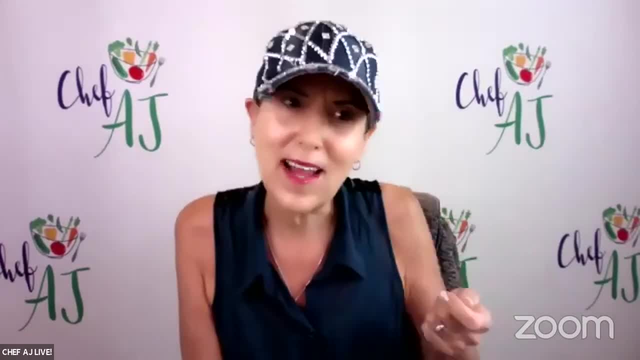 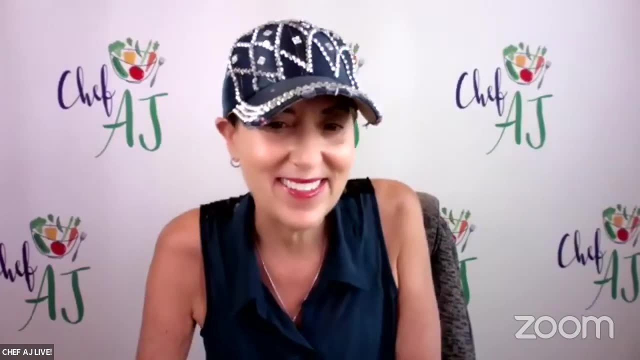 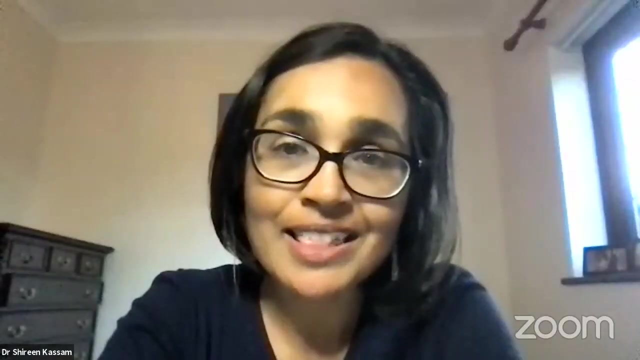 them went vegan for ethical reasons, as did you, because you think, oh, they're a doctor, it must be because of health. so I love that. you have that Absolutely, and I think you know we all have to use our platform as best we can, and I think, as a 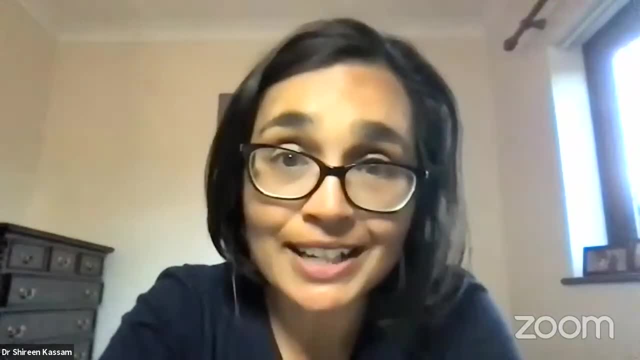 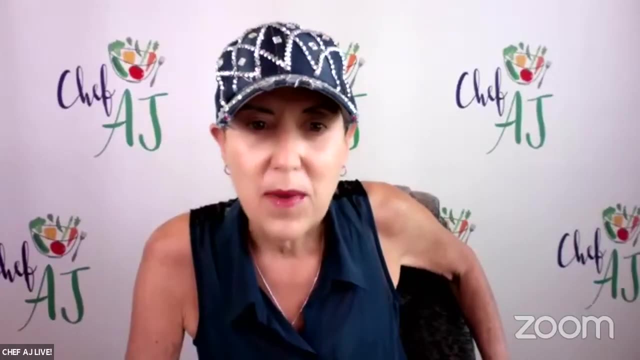 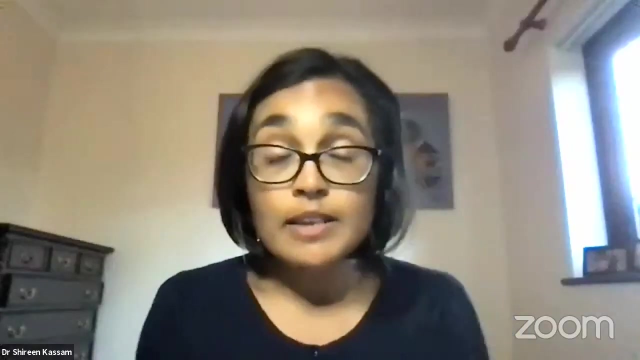 healthcare professional. we're trusted to give health-related information, and that's kind of how I use my voice in this. this movement- Great, thank you. Karen says: have you seen better hemoglobin numbers go up with nutritional intervention? Well, so that's. that's also can be a complex question. I mean, there's absolutely no doubt. 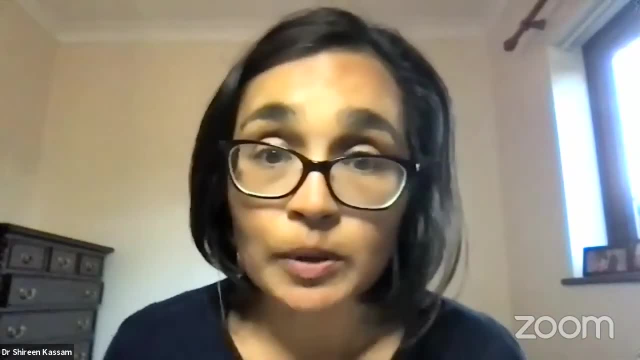 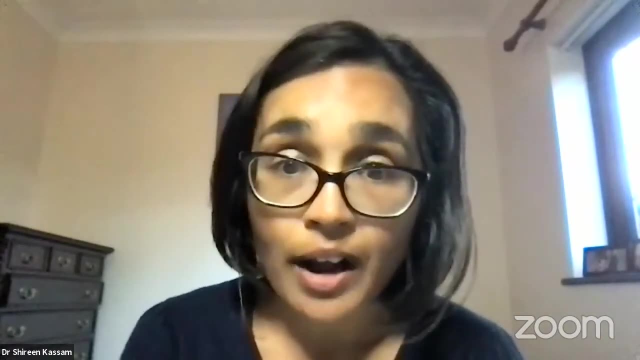 that you know a plant-based diet is going to support normal, healthy blood counts. There's so many reasons why your blood count may not be adequate and, as we know, iron deficiency is one of the commonest nutrient deficiencies globally, and especially in young girls and menstruating. 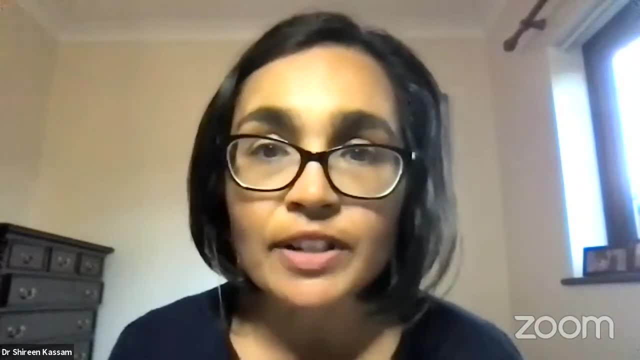 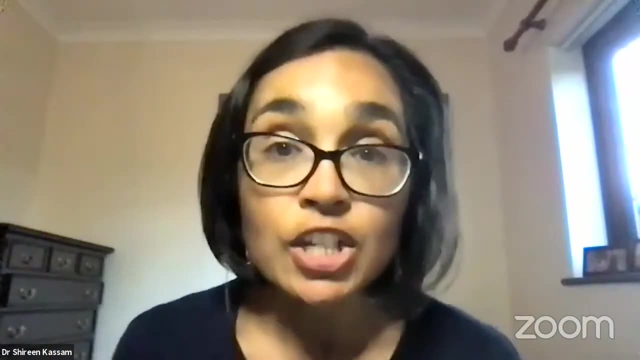 women. so I don't particularly see a difference in terms of, you know, good and bad. in terms of blood counts, I think anyone, regardless of diet pattern, can have issues with certain nutrients and their blood counts can take a hit, and vice versa. you know all diet patterns can. 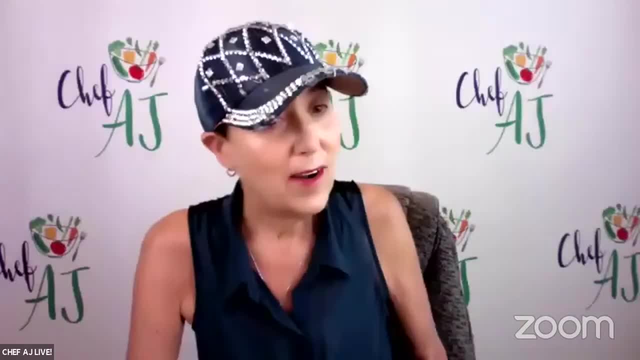 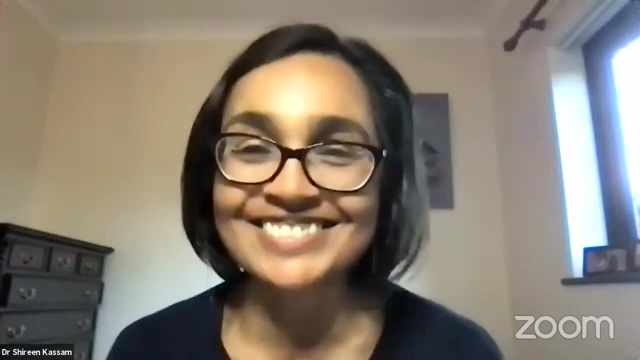 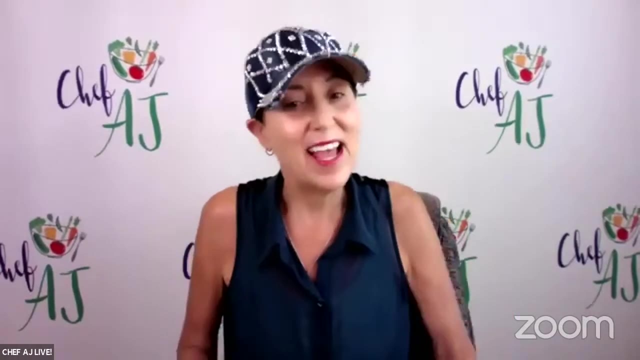 support a healthy blood count. Nice, Are you the primary chef in the family? I am, yes, yes, traditional roles, Yeah, well, that is I just think. whoever does it, I don't. I think whoever is better at it should do it. that's my feeling, you know. regardless, Do you have some of? 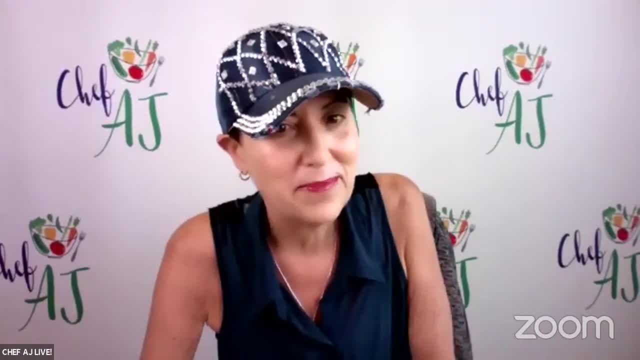 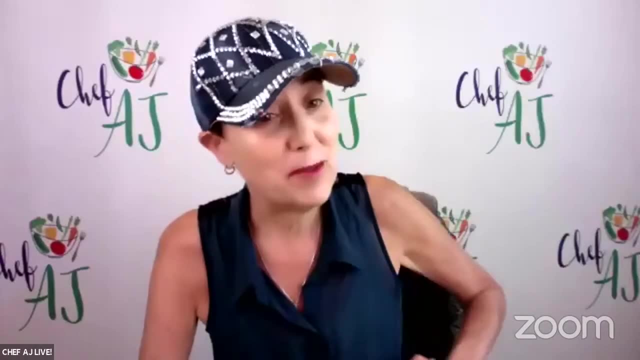 my favorite foods. I think I have a lot of favorite foods. I think I have a lot of favorite like the instant pot or the air fryer at your disposal. I don't actually. I think the most complicated I've got is a vitamix actually. Wow, they have those in England, though you just don't. 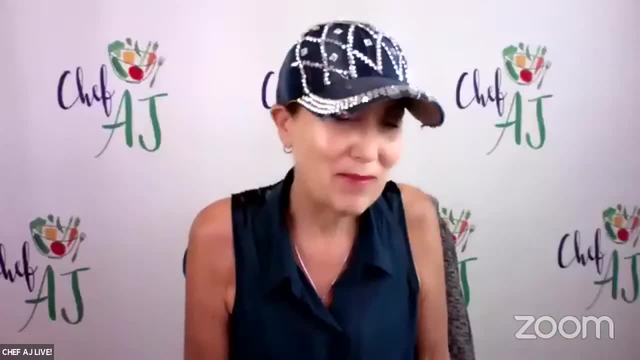 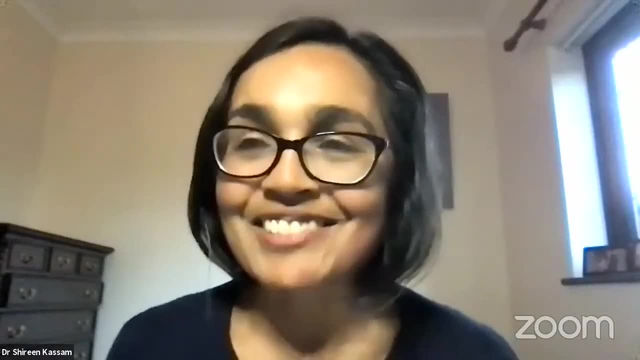 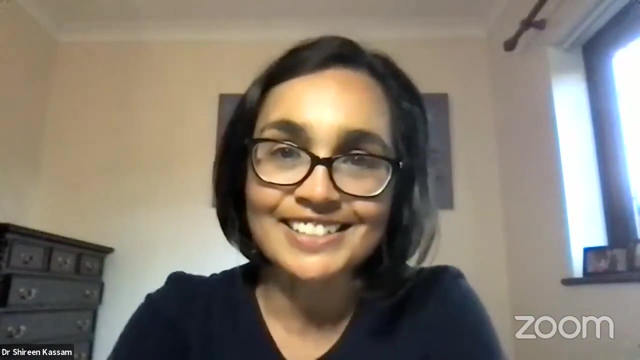 have? They certainly do. Oh, they're a game changer, Dr Kassam. consider at least getting the instant pot. What kind of things do you eat and feed your family? Yeah well, I mean I'm not very excited, exciting in the kitchen. I go back to my traditional roots, really. so curry is a firm favorite, so you? 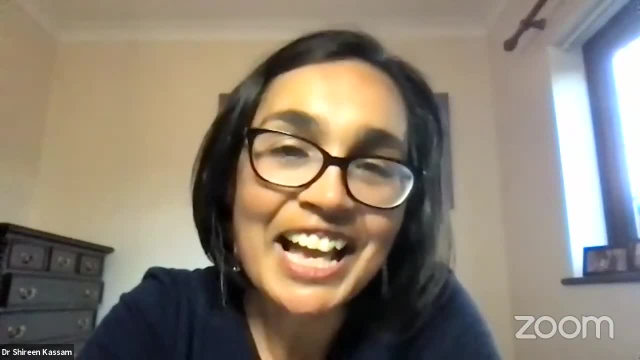 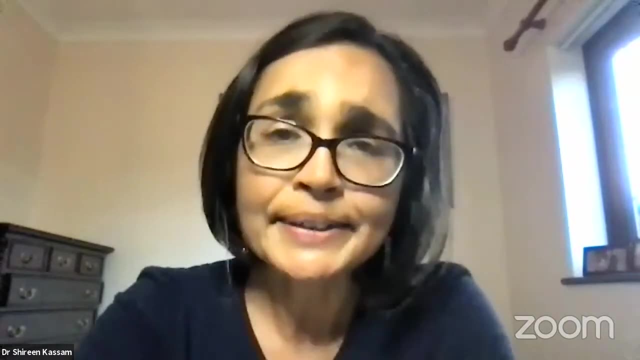 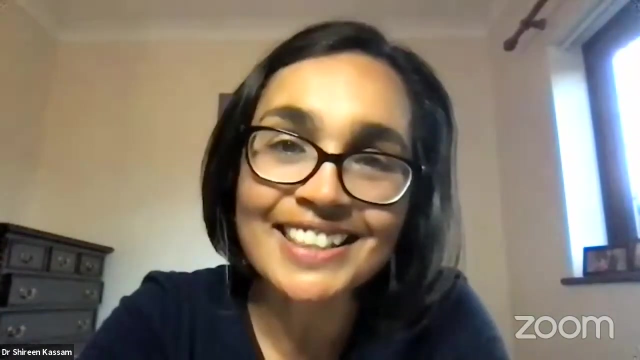 know tofu, curry, vegetable curries, the dals, etc. and actually I have to say my husband's a really good cook, but it comes down to wanting to make healthy meals and if I let him cook then you'll get the added this, that and the other that I don't necessarily want, you see so, but yeah, so I stick to. 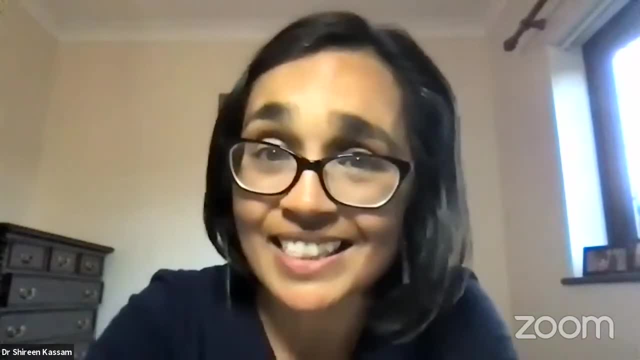 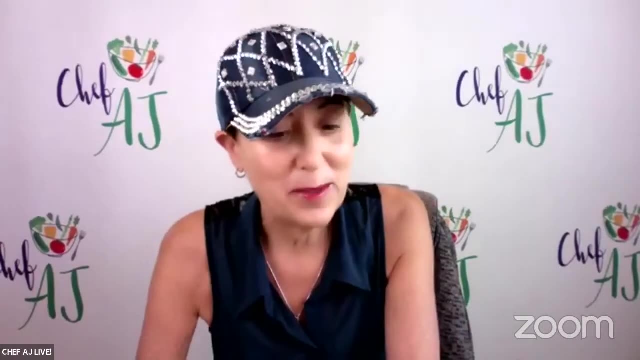 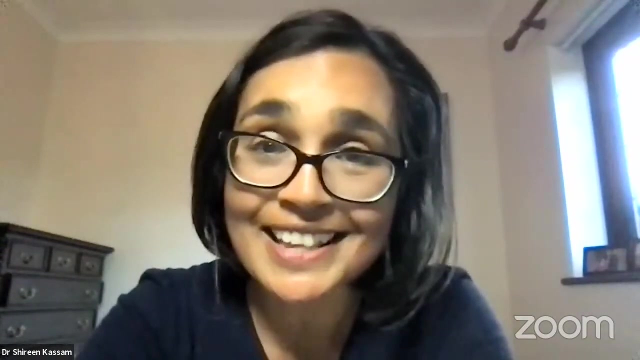 the spicy foods, the curries and the stir fries and that sort of things. anything in a one pot, a pan, will do. Wow, that's nice, let's see. are you an avid exerciser? I do exercise. It's not something I've always enjoyed, but we have a dog, so you know it necessitates, you know. 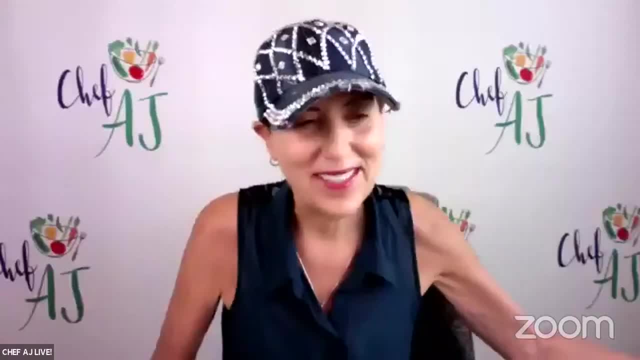 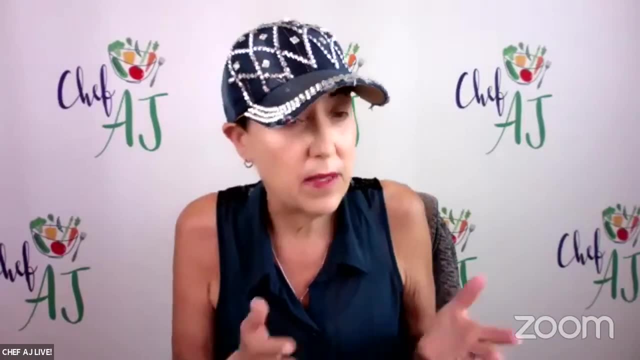 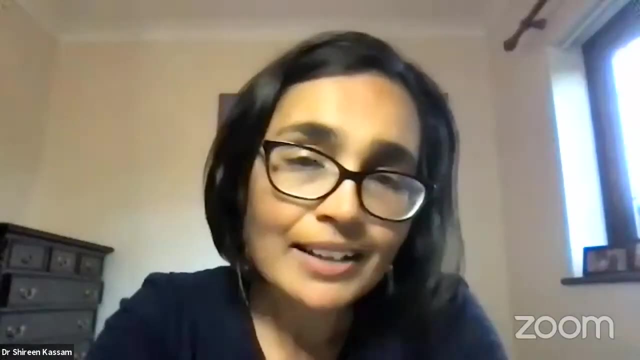 lots of walks, so that's lovely. I love dogs- great. How much do you think a plant-based diet can really affect cancer in people, either when they have it or before they have it, because, as you know, most doctors aren't telling people this when they have cancer? I think it's hugely important for 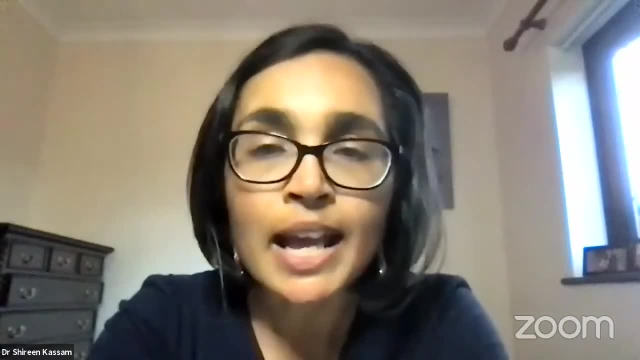 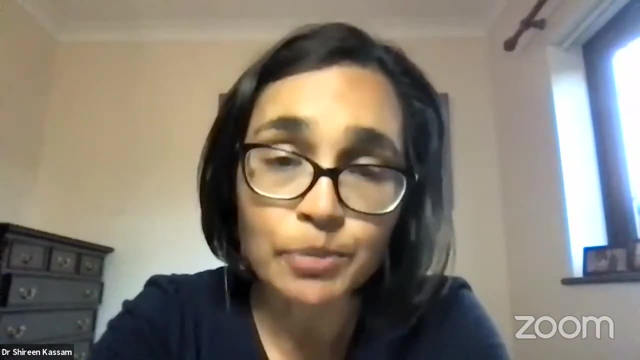 quality of life, well-being. you know how you're going to do with treatment. You know, I guess the best evidence we've got to support this is for the common cancers, so breast, colorectal and prostate cancer. You're never going to get a big study in my specialty of. 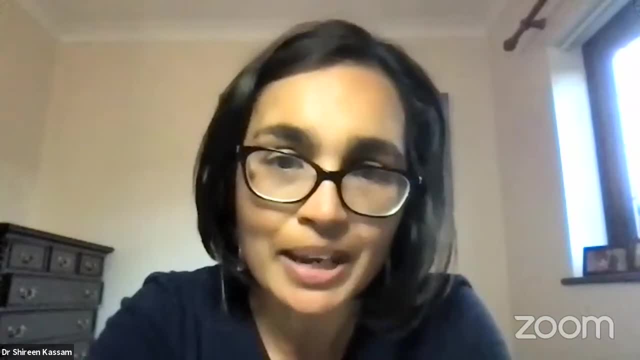 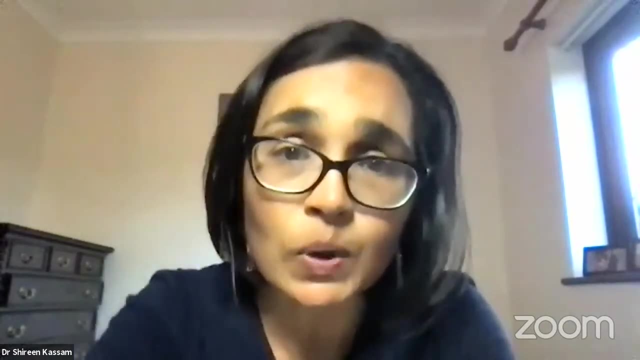 lymphoma, where there are 40 different types and you're never going to get enough information. but, as I say, it keeps people well to tolerate the treatment. if you do get cancer- because of course we can't prevent all cancers, but we do know for the big three- you can reduce your risk. 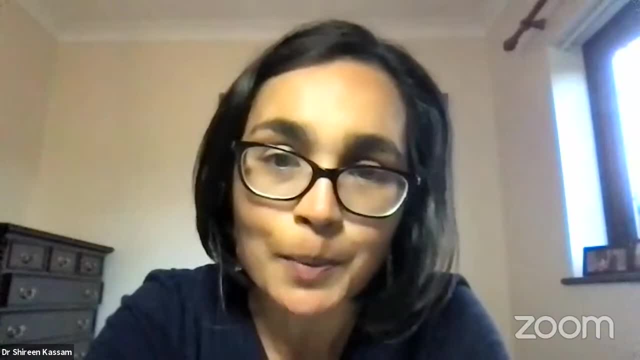 considerably so. over 50 percent of bowel cancers, for example, are cancerous. So I think it's really important to have a good diet, and a good diet and a good diet are related to lifestyle habits- about 25 percent for breast cancer- and, as I say, the guidelines. 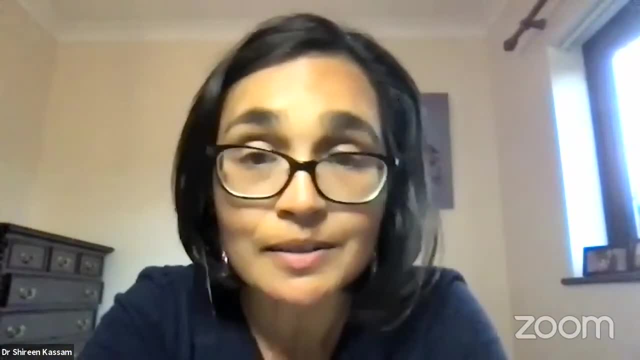 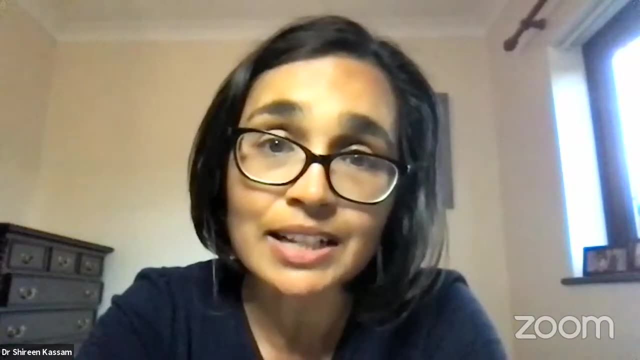 say we should be eating a healthy diet full of fruits, vegetables, whole grains, beans, nuts and seeds, because they're the only foods that have been associated with good health and reducing your risk. So I think it really does have a huge part to play. Yeah, you would think people know. 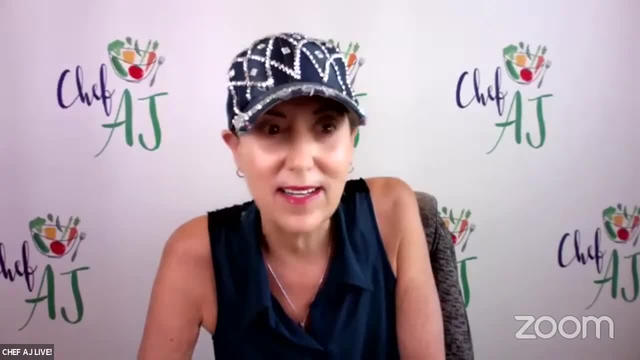 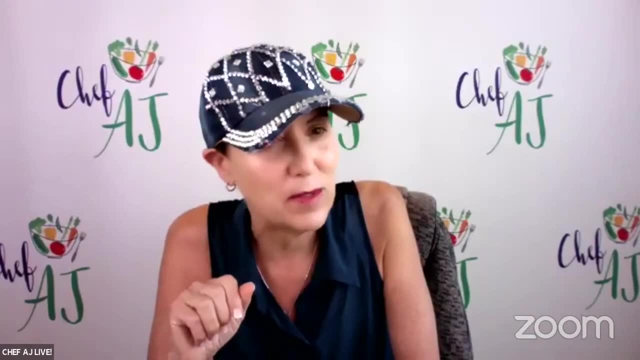 that. but there's diets now that are based on just meat. I mean, there's this, and some very famous people are doing this carnivore diet and I don't get it. you just eat meat, you eat nothing else. I mean, that sounds very unsatisfying. 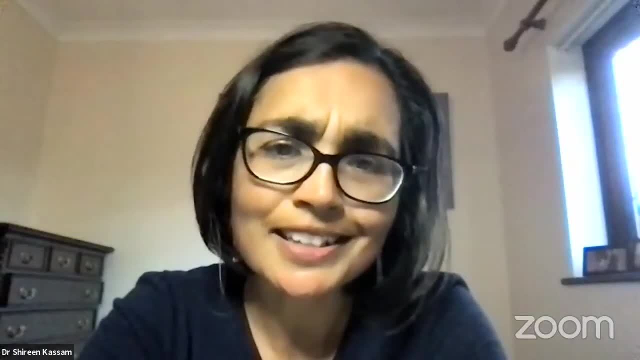 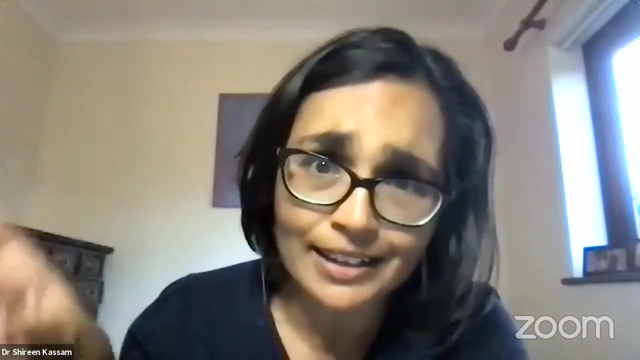 Well, I mean, you're going to be so nutrient deficient. I mean, the only foods we need to survive and thrive are plant foods, and you know, if you choose to eat meat, it needs to be a tiny little portion on your plate as a condiment, doesn't it? and really it's just the the wrong way. 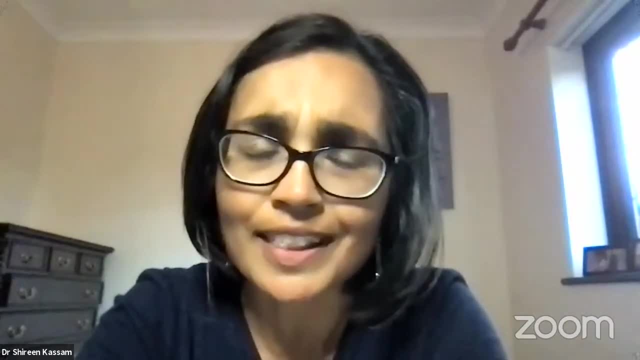 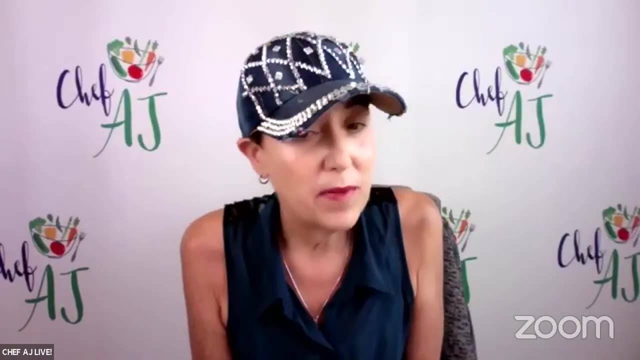 around. I really do hope that health professionals are not advocating for that because it goes against all the scientific literature and teaching. I don't think they're advocating for the carnivore diet, but I hear a lot of people that come to me for help with diabetes that their doctor has. 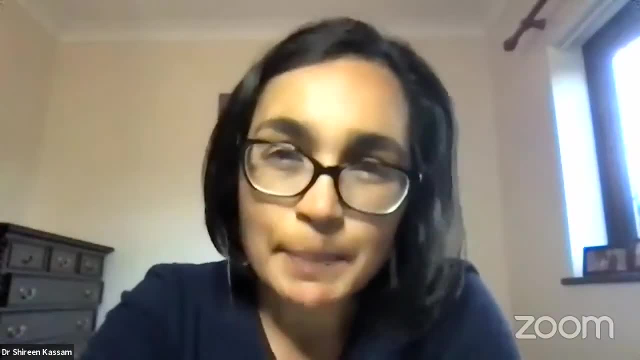 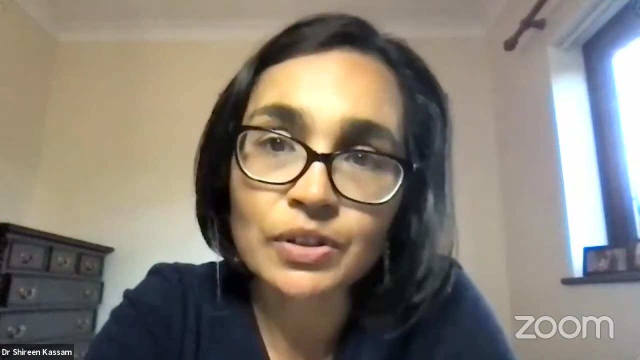 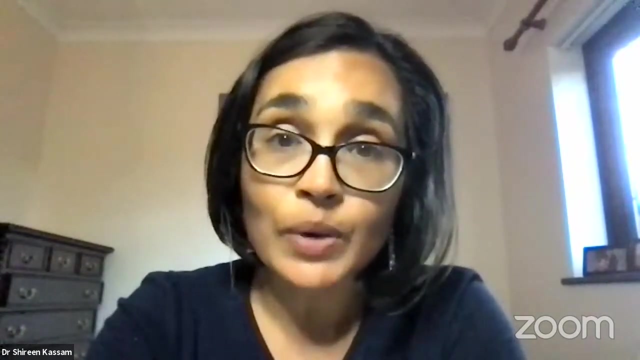 suggested keto. Yeah, I mean, that is a particular problem in in the UK. We do have a large body of healthcare professionals that advocate for sort of a low carb approach and, to be honest, you know you, you can get short-term results and and you know we can't deny that there are short-term 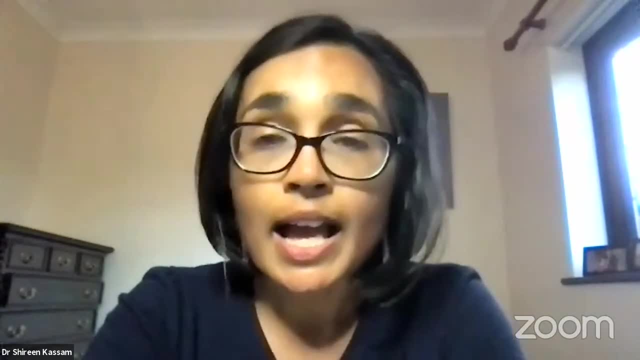 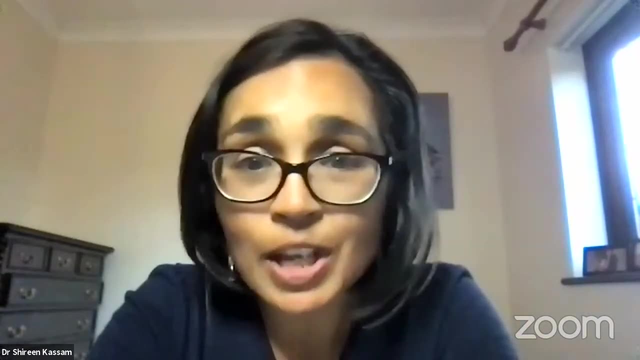 results in weight loss and lowering your blood sugar and, you know, maybe lowering your triglyceride levels. but you know, beyond six months to a year there's very little data. We know people can't stick to it and again, you know you're excluding some of the healthiest foods. you know: whole grains. 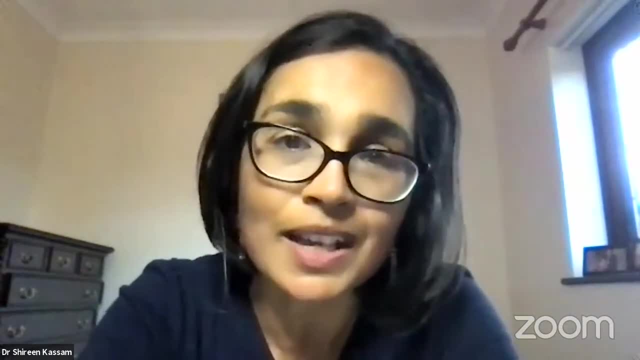 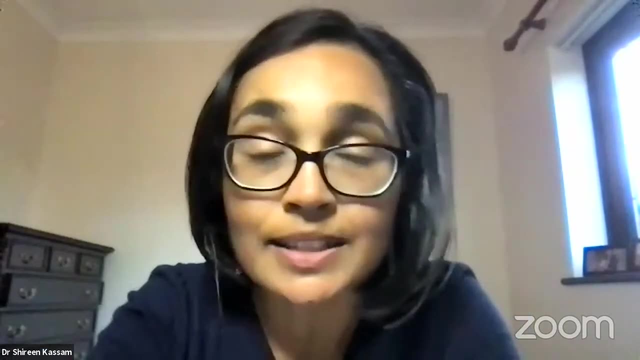 and beans and limiting your fruit consumption, all the foods that have been associated with promoting insulin sensitivity. and then when you look at the long-term studies, you know you find that people on low-carb diets, especially if it's heavy in meat and you know animal protein and 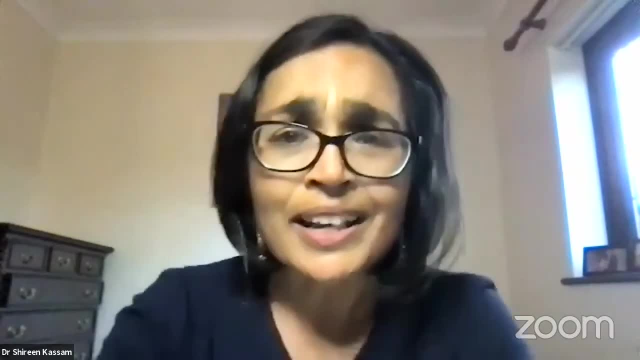 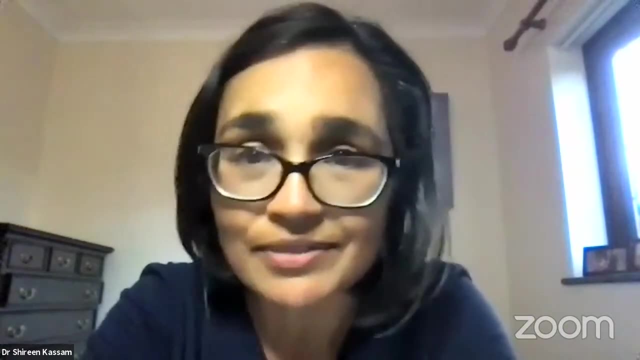 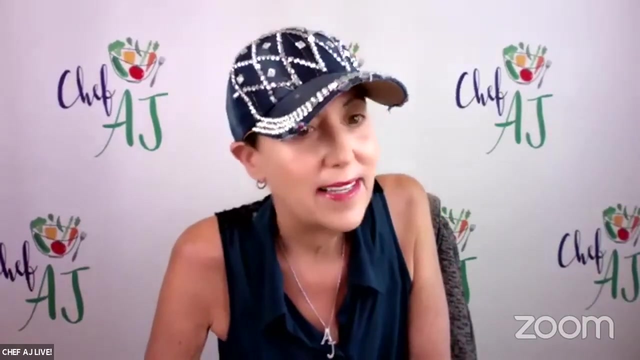 animal fat that they get increased risk of heart disease and cancers. so you know well as we know, if you choose a plant-based approach, you don't have to have those trade-offs for short-term, long-term issues. Right, have you been able to influence any of your colleagues, your medical 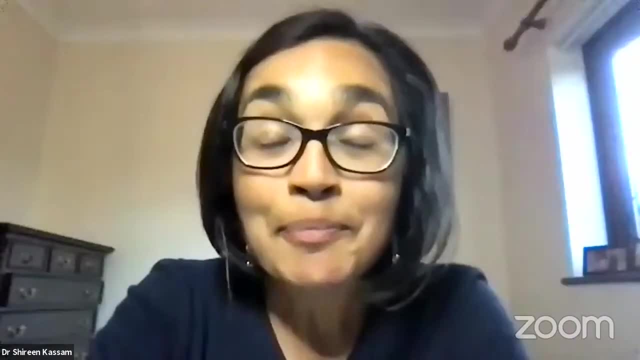 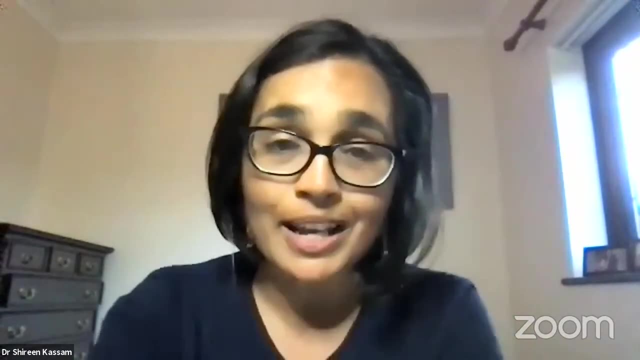 professionals by your dietary choices. Yeah well, I mean I certainly I've seen the growth in our membership in plant-based health professionals, that's for sure. I mean I think more and more people are coming on board. I see from the discussions we have on our course at Winchester. 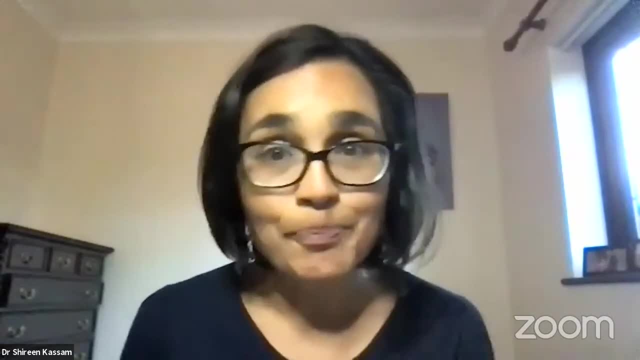 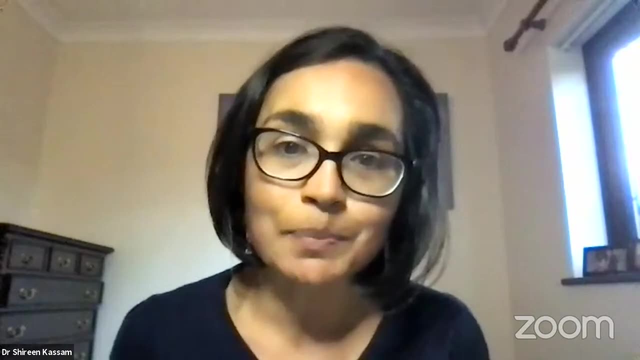 University because it's facilitated. there's a chat. you know people you know responding about: well, I'm going to cut down my dairy, I'm going to give up my dairy. I'm going to give up my dairy, I'm going to give up eggs, you know. so not everyone's coming to the course as being 100%. 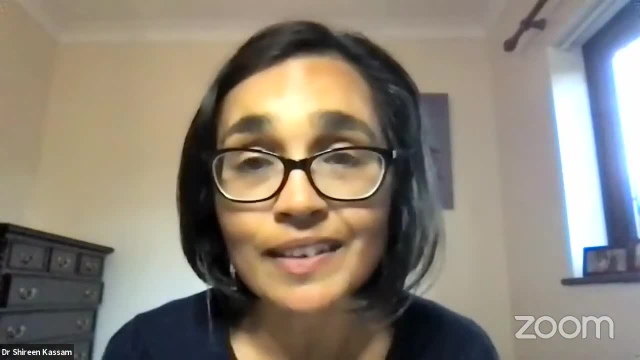 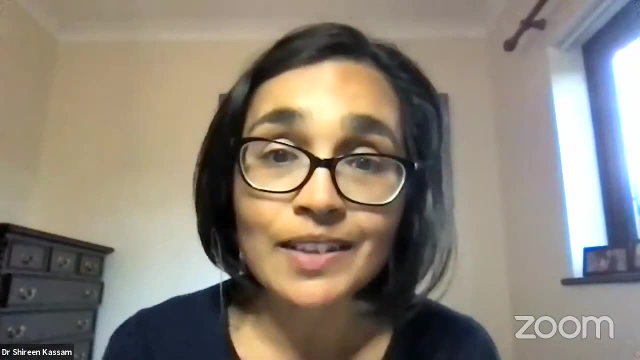 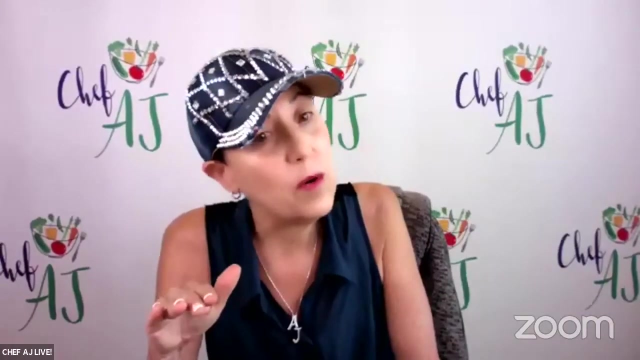 plant-based. so I hope, in that way, that I'm having an influence and, as I say, our sort of online education and webinar program isn't just pulling in already vegans or plant-based. so I'm hoping that it's slowly- slowly, you know- infiltrating through. How long of a commitment is the course? 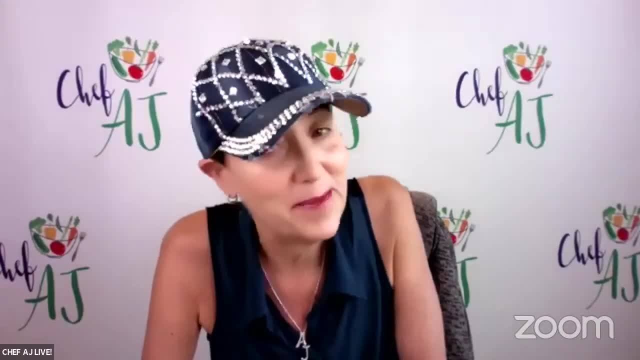 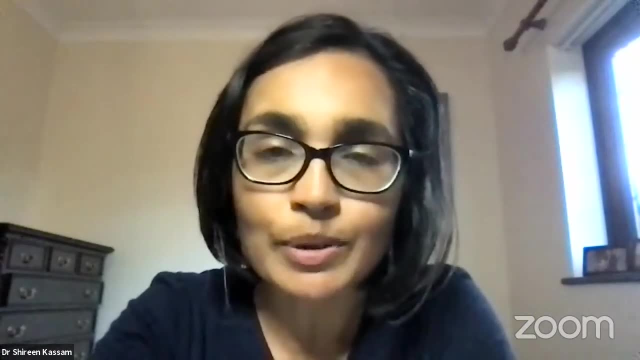 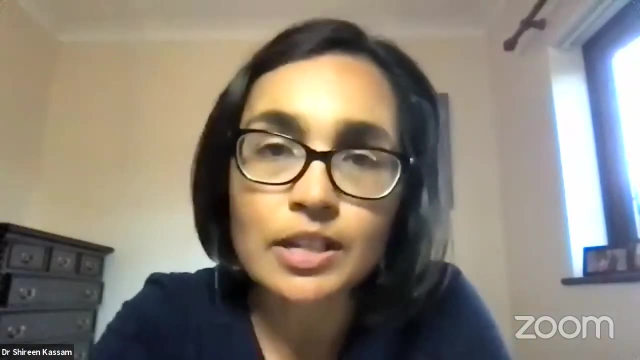 if any of our viewers want to take it. is it weeks, is it months, is it years? Yeah, no, it's eight weeks but, like with everything, tried to cram in too much, so we've allowed people eight weeks to finish it, which is plenty of time and, yeah, and it runs sort of, you know, back to back during during. 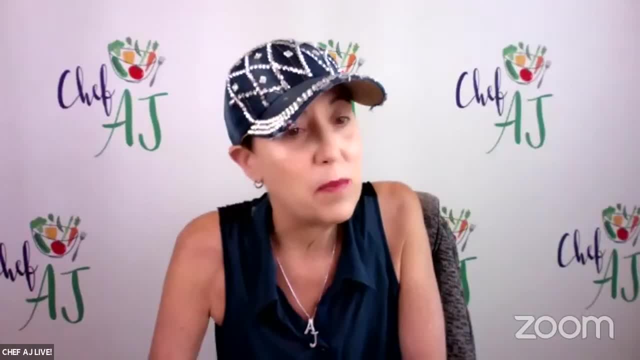 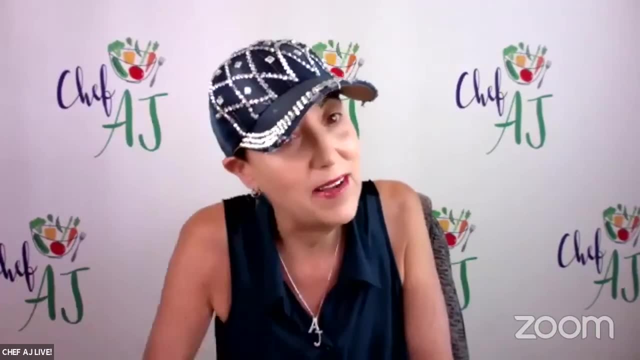 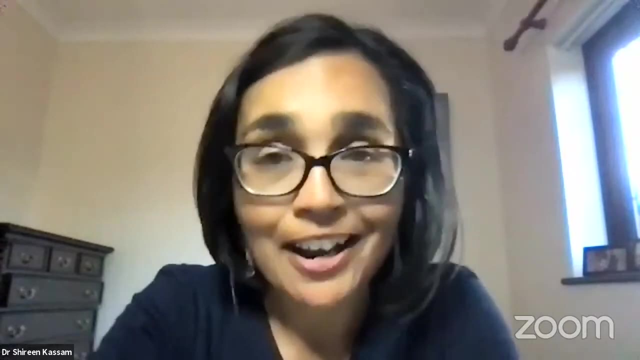 the year. So your telehealth service it's multidisciplinary, it's not just primary. so people in the UK have like need a GI doctor or an orthopedic doctor, would they have access to different specialties? Well, not immediately right now, because we just launched in January the idea. 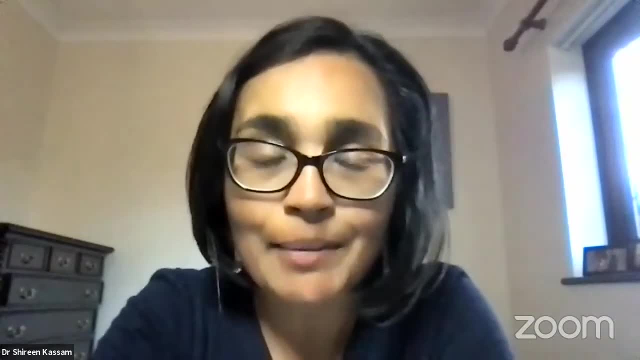 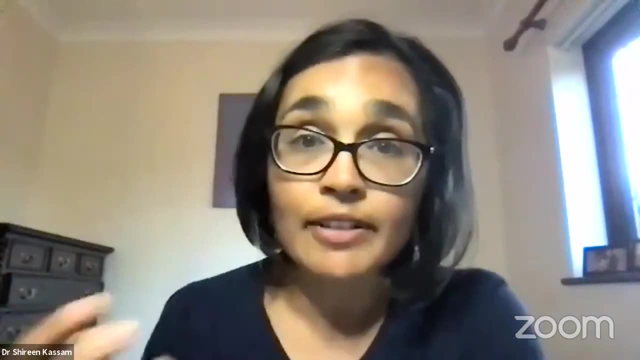 is obviously to expand and we're going to have a lot of people in the UK who are going to have to expand and be multidisciplinary and certainly within our plant-based health professionals we have virtually all of those specialties covered, but not necessarily under the plant-based health. 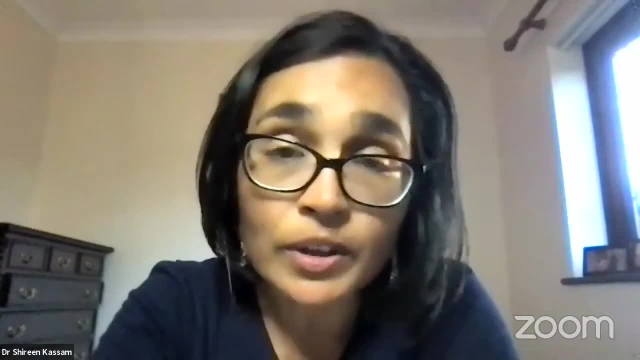 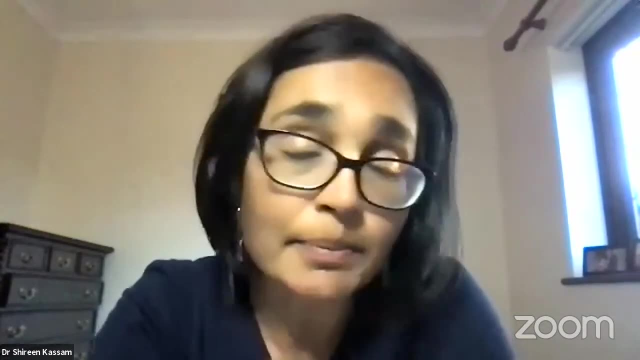 online umbrella. so if anyone is in the UK and wants to find a plant-based health professional- and there's specialty- it is listed on our plant-based health professionals website, but you can get in touch with me and I'll point people in the right direction. if plant-based 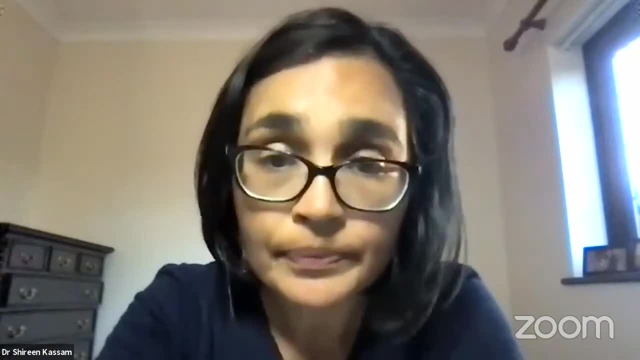 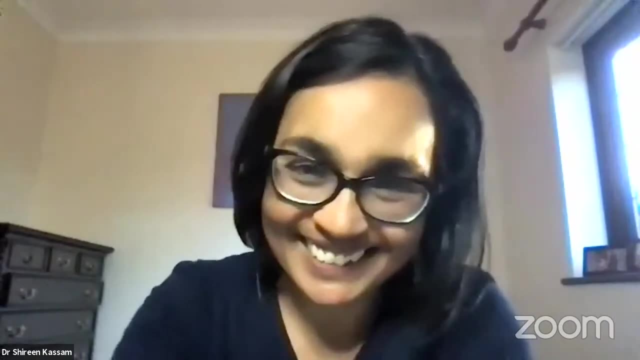 online is is not the right thing for them. Great, thank you. So talk about the research paper you wrote and selenium, because I find that fascinating, because the only the only place I think you get selenium is like Brazil nuts, right, Well, one of them. you do find them in seeds. 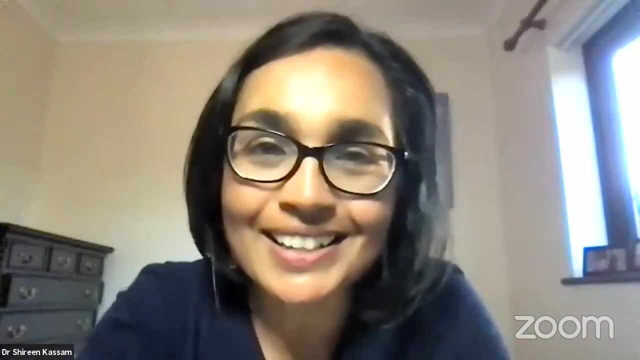 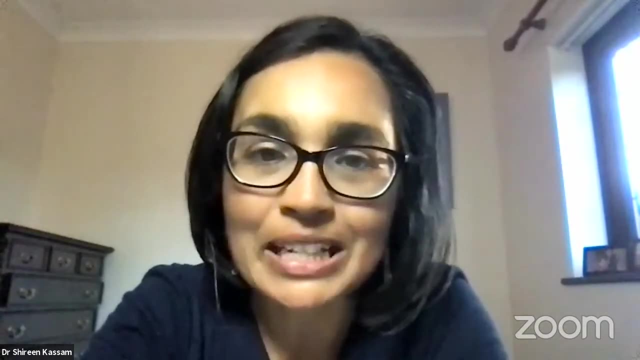 and whole grains as well, but obviously it all depends on how good the soil is and how much selenium in the soil. but yeah, having one or two Brazil nuts a day is a good way of meeting your requirements. Yeah, I mean I wasn't vegan at the time, I was vegetarian. I hadn't really been thinking. 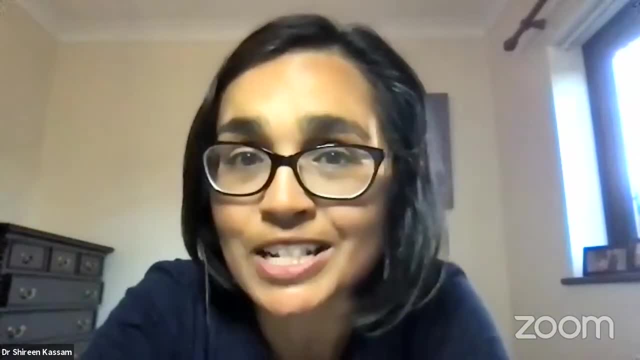 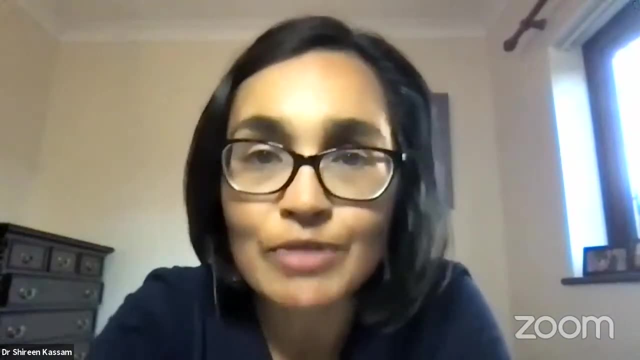 about diet and nutrition and I sort of knew I wanted to do some further studies, but I didn't know what I wanted to do. so I decided to study in a PhD and understand sort of laboratory practices and also, you know, delve into reading research papers and things, and this project came along. 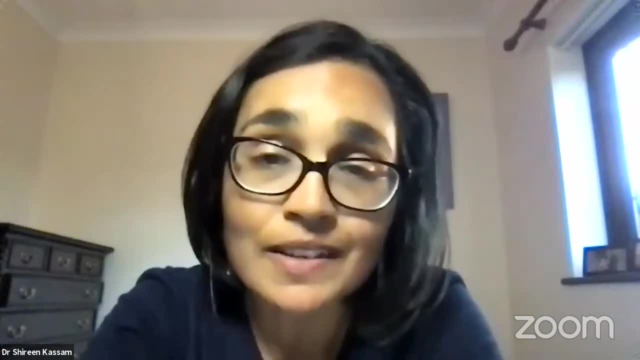 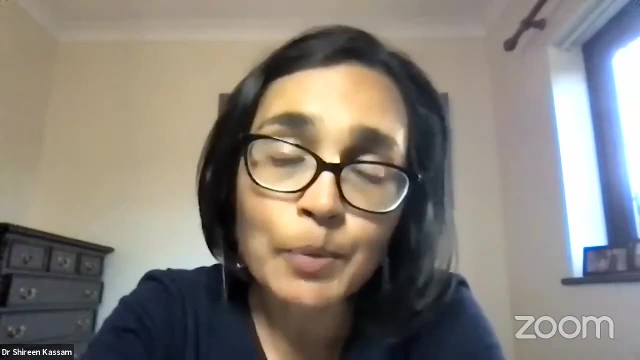 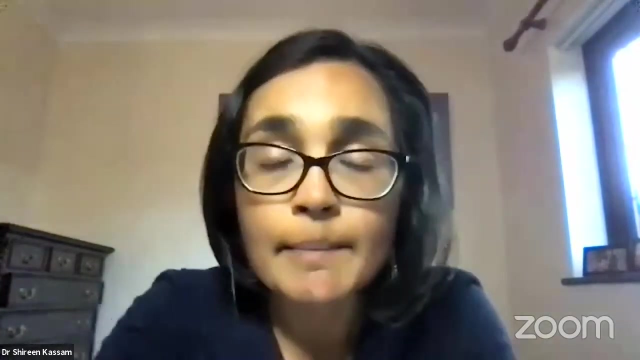 and it sounded interesting. so I looked at the impact of high doses, so super nutritional doses, of selenium and its ability to sensitize cancer cells in the laboratory to chemotherapy. and so in the US at the time people had been doing some experiments in the laboratory and in humans and 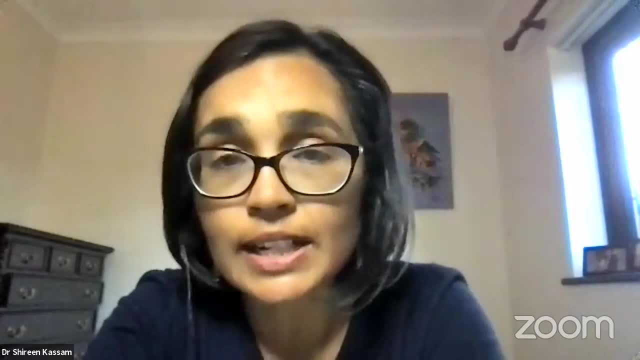 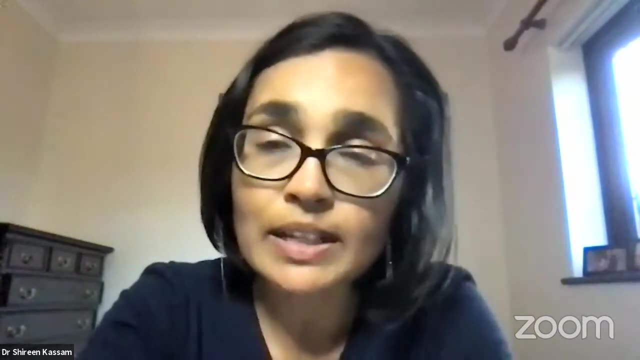 looking at this sort of combination of chemo and high doses of selenium in people with bowel cancer. and so I was doing sort of similar things with human cell lines. I wasn't doing animal research, human cell lines looking at the impact in lymphoma cells to see whether there could be an additive or 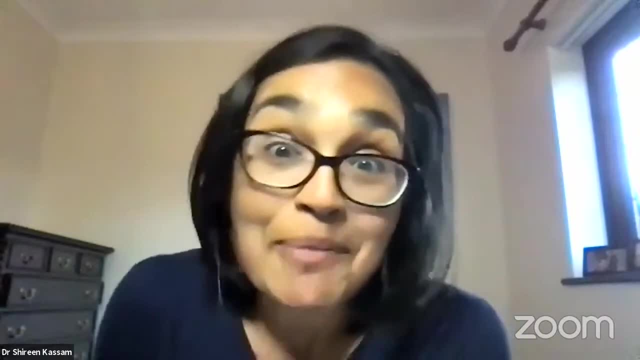 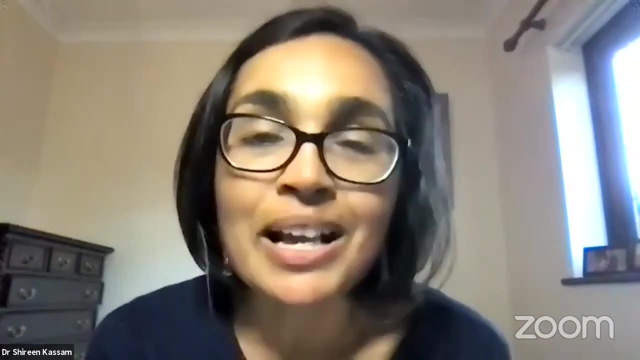 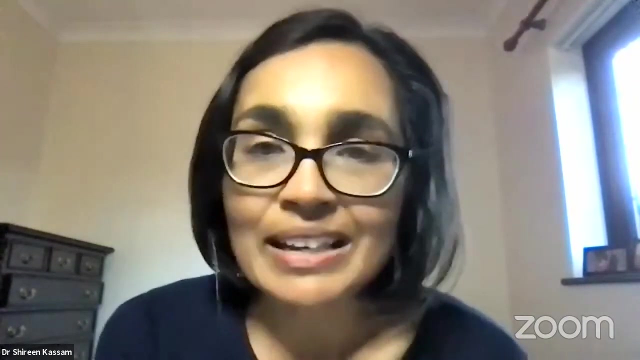 synergistic effect of adding in selenium and of course I mean there was actually interestingly, so you know- we were able to see show in the laboratory setting that high doses of selenium was able to sort of enhance the cell link impact of the chemotherapies. but we didn't actually make it to the next step, which was the 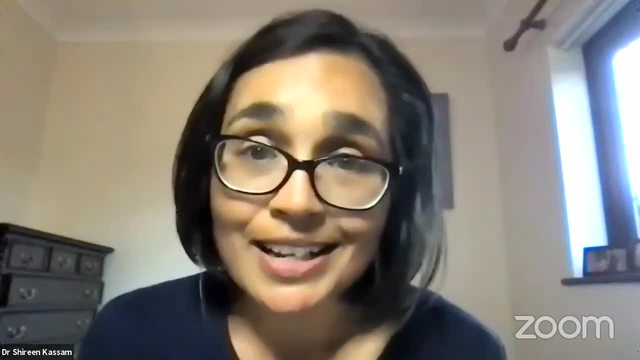 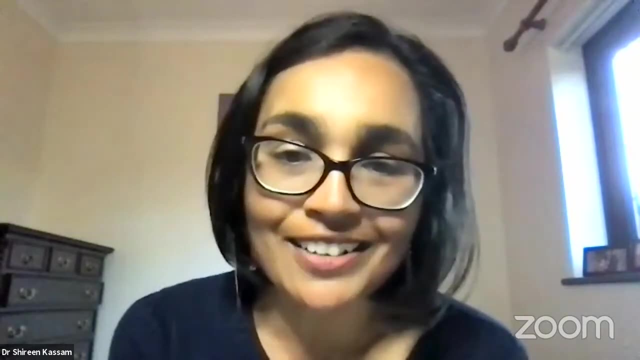 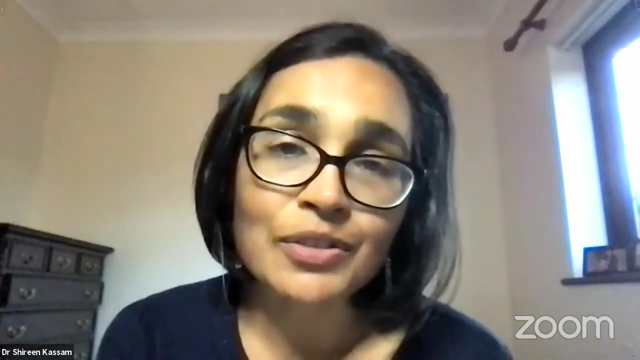 sort of patient stage and for all the reasons you might imagine, it's quite difficult to get a non-pharma funded study off the ground and you know the nutraceutical industry are not used to funding big clinical trials. and also, at the same time, sort of a note of caution in that there was 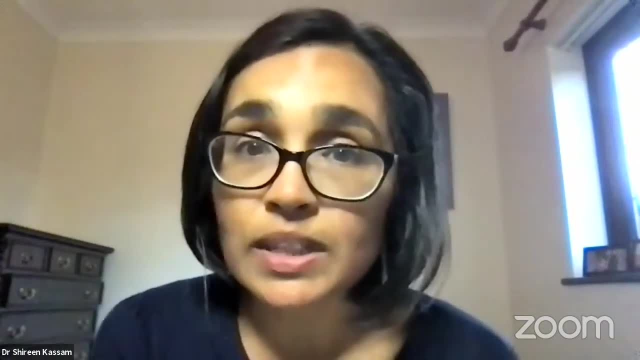 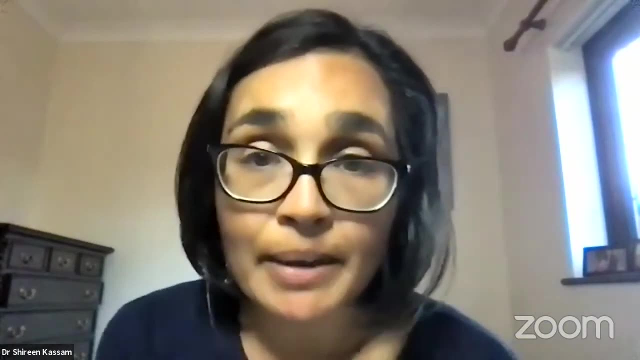 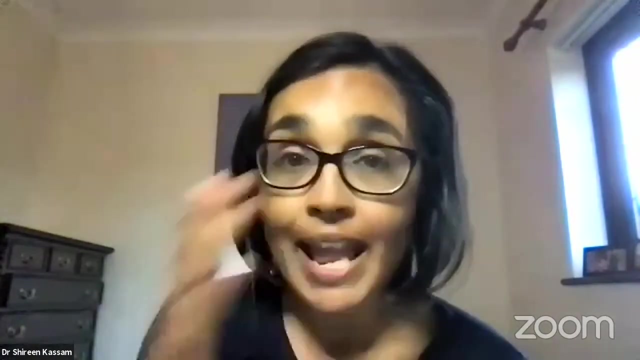 this big study- I think it was mainly out of the US- called the Select Study, that was looking at people at high risk of prostate cancers and men with prostate cancer and they were supplementing with vitamin E and selenium to see if they could prevent future prostate cancer. and actually that study had to end early because the selenium group had a signal for 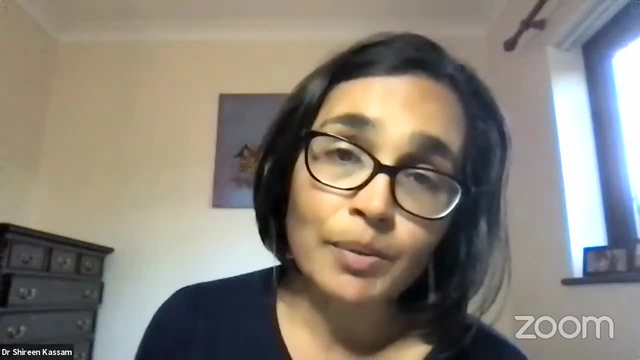 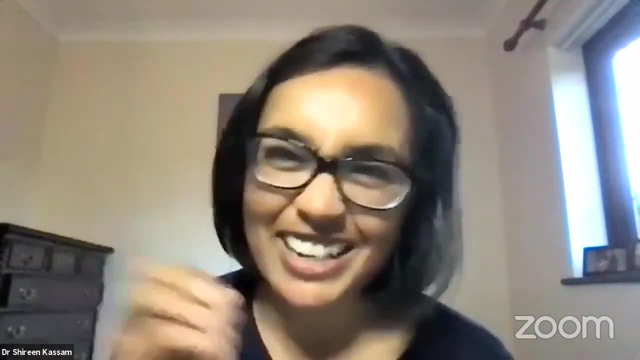 increased risk of type 2 diabetes, and the vitamin E group had a slight signal for increased risk of prostate cancer. so it sort of brought me back to what I should have known already is that you really can't take the nutrient out of your body, and you can't take the nutrient out of your body and you. 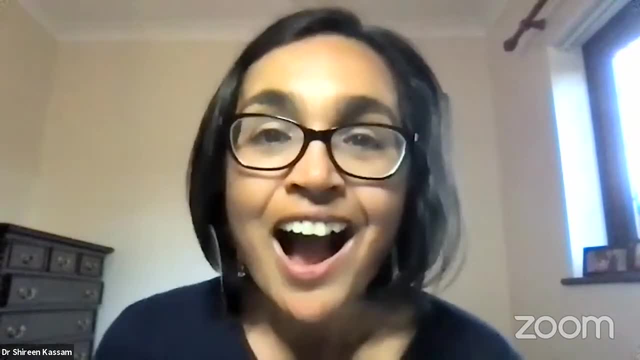 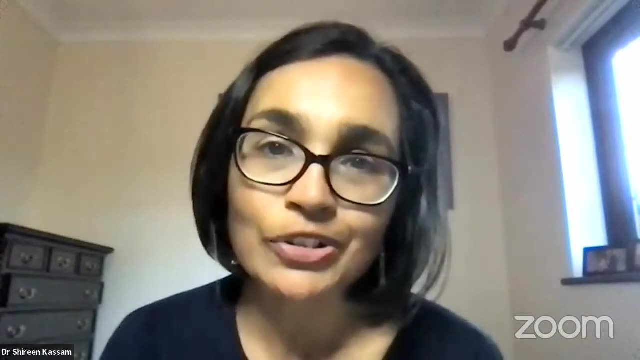 can't take your food and expect it to do wonders, and I don't think that approach is really going to be useful for us going forward for cancer prevention. I think we need to concentrate on diet quality, as you do on your show, and think about the combinations of the healthy foods. 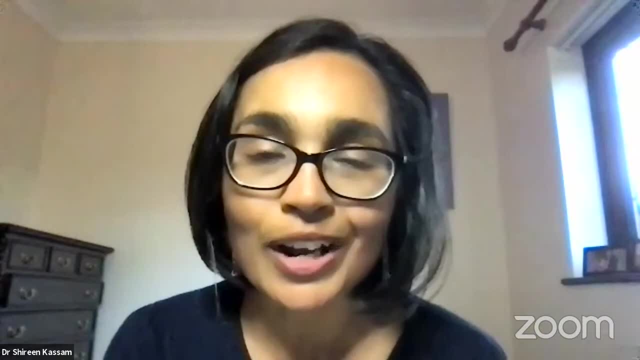 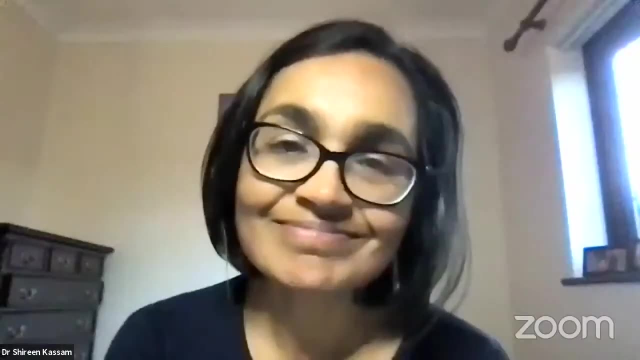 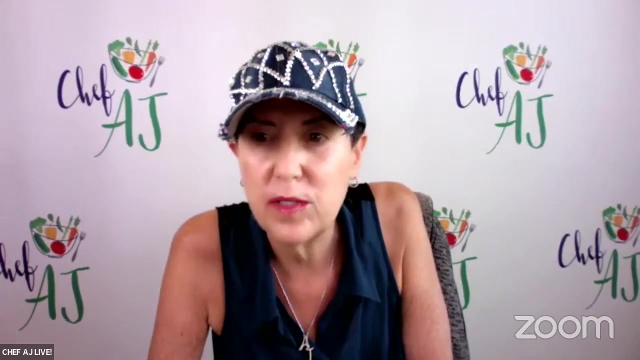 rather than extracting little bits and hoping it's going to do the trick, and that's what people are looking for. don't you think, though? a pill for every ill, rather than having to do diet and exercise? I know well Sharon has been asking regarding your research on selenium and cancer. which form do you suggest people? 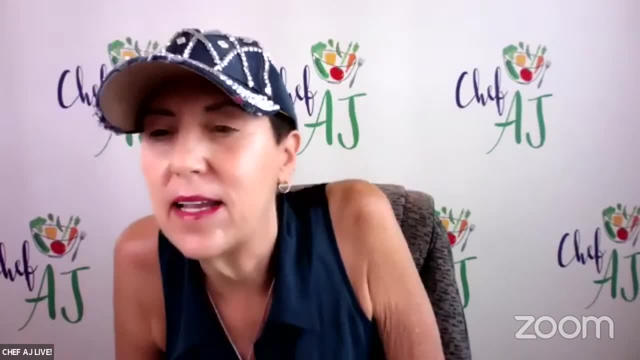 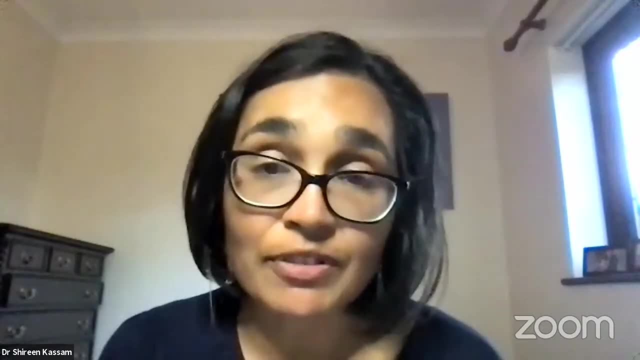 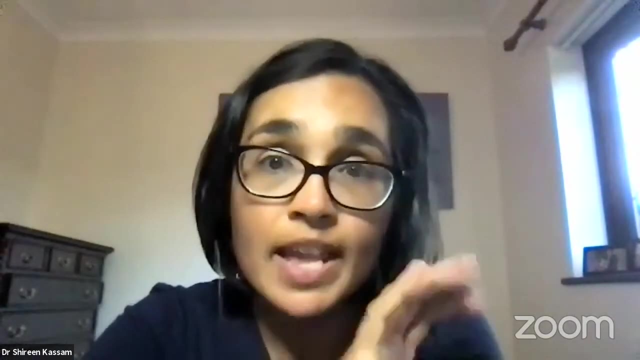 supplement with sodium, selenite, brazil nuts, and how much? yeah, well, so I mean I think you know it is best to get it from food if you can. if you are struggling to get it, then this, then a supplement will be all right. the upper limit of what you can tolerate, I believe, is about 400 micrograms. you shouldn't probably go above that, but I don't think the form matters so much- selenium, methionine and the selenite, as you say, so I don't think that really matters so much when you're, when you're supplementing with it, but ideally food sources, and if you can't, then 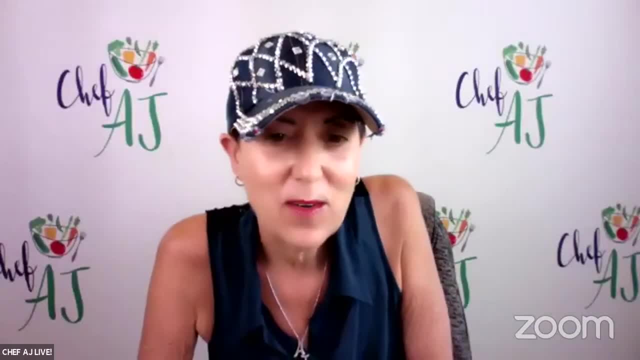 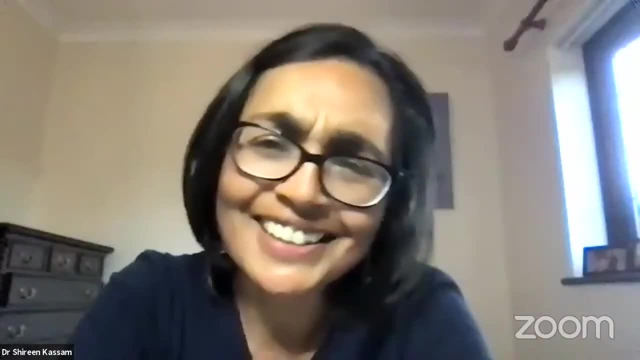 then a low dose supplement. great um. Anne has a question. she goes: will you share with us your curry recipe? maybe you'll come on, maybe you'll do a cooking demo sometime. oh my goodness, no, that would be way out of my comfort zone. I don't think people will enjoy that. but it's very basic. 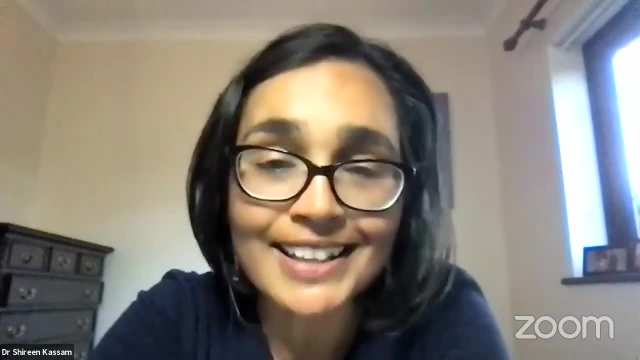 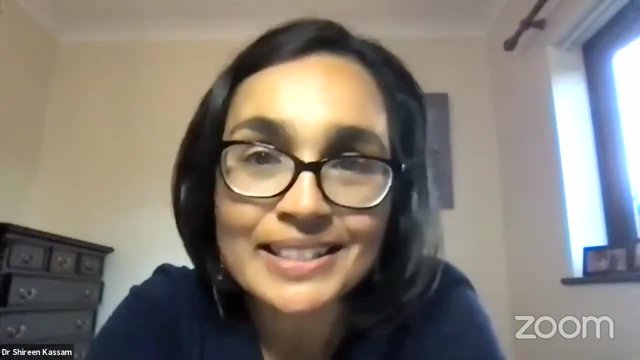 it's, you know, water frying your food, and then you can do a little bit of that with your food and some onions. it's adding some cumin seeds, um, it's then adding some tomatoes and then, um, stirring up some masala with your turmeric and cumin and coriander and then adding in whichever vegetables. 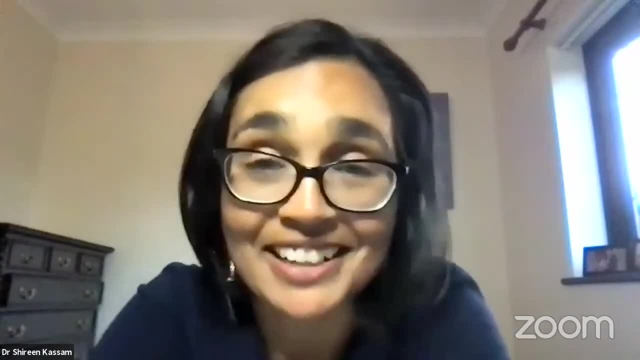 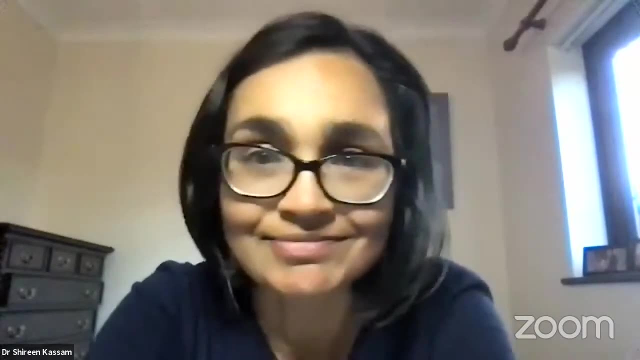 it's very simple, and sometimes i add some curry powder and agar and masala as well, other times like i'm too lazy, and then you use the basic spices. obviously garlic ginger goes in everything. yes, oh yeah, you can't get garlics and non-negotiable uh. so dina says: do you know? 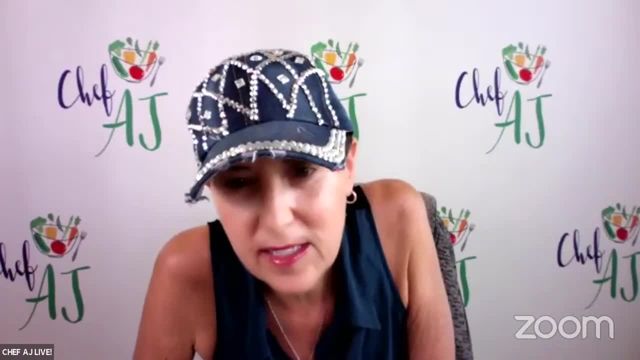 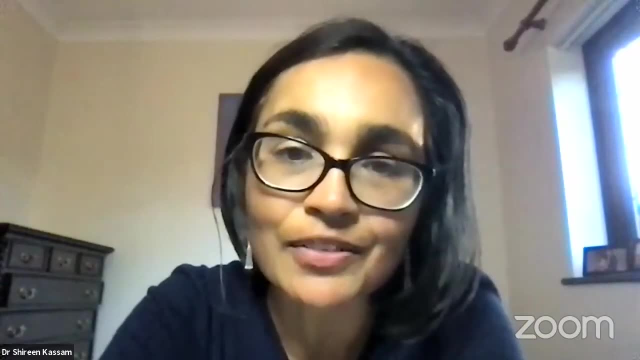 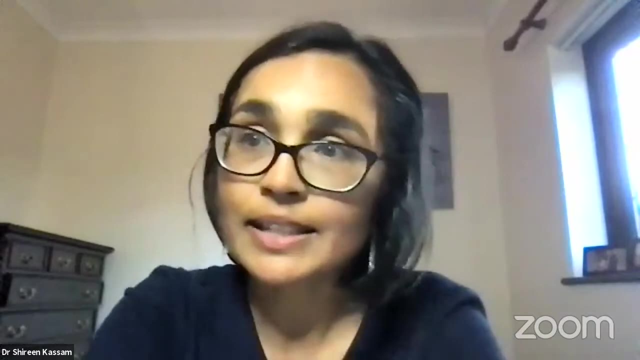 dr, i'm full. i pronounced the name right: ranga shatarji. yes, i mean i don't know him personally, but obviously he's a big influencer here in the uk and and overseas and a big proponent of lifestyle medicine. i don't believe he's described himself as plant-based yet, but maybe soon, okay, i. 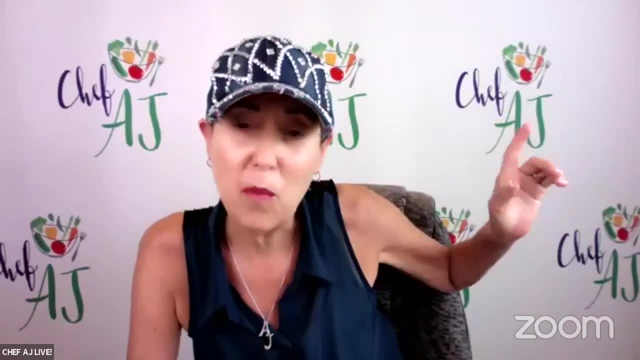 don't really want to get into vaccine territory because it's too complicated. i don't want to get into vaccine territory because it's too complicated. i don't want to get into vaccine territory because it's too controversial. but this is not about the. this is a other. one is asking if you notice an increase. 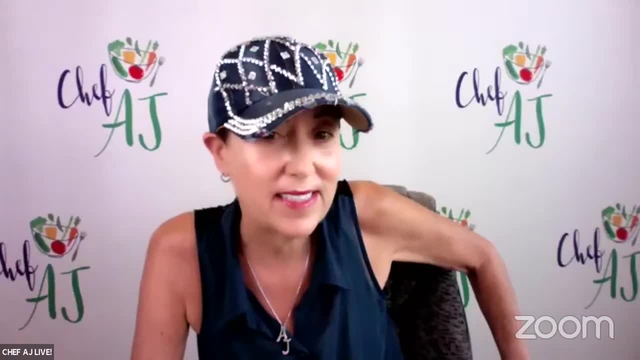 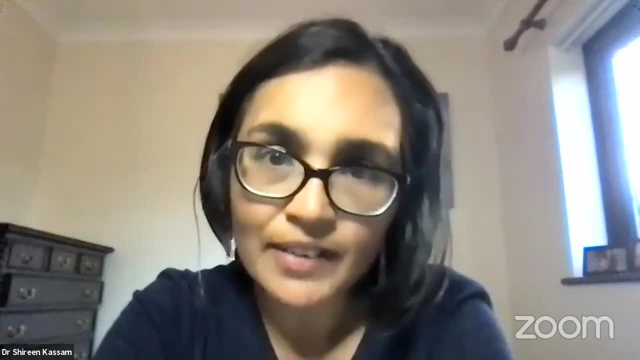 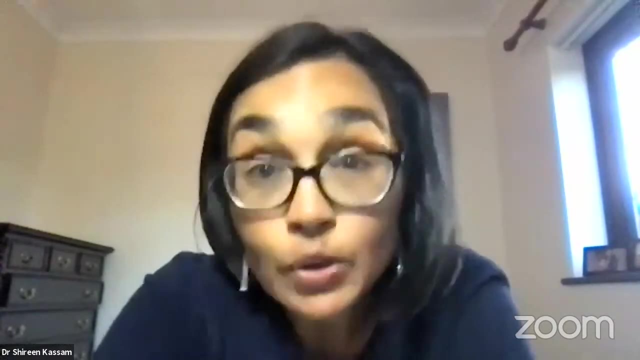 in acquired hemophilia, possibly because of it? uh no, the. the main um issue with some of the vaccines has been this: vaccine induced thrombocytopenia or thrombotic thrombocytopenia, so it's not really. you can get bleeding with that, but it's not the same sort of thing as. 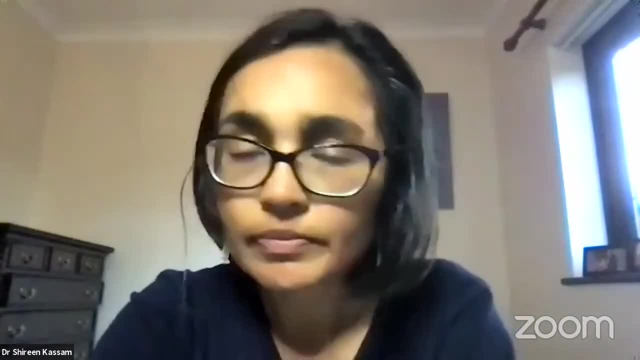 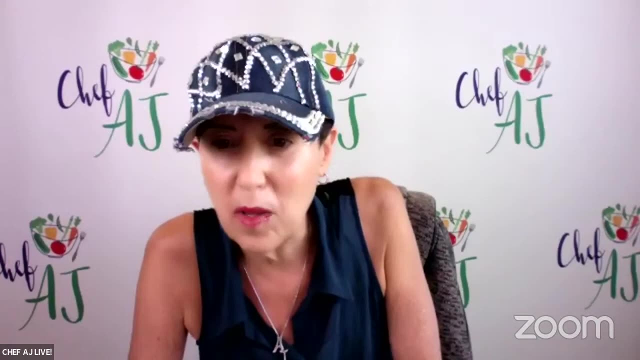 hemophilia, but maybe that's what people have been referring to. right, let's see. oh, here's an interesting question. dr mcdougall warns against omega-3s, alas, because they thin the blood, but it seems inconsistent with other plant-based doctors who promote it. 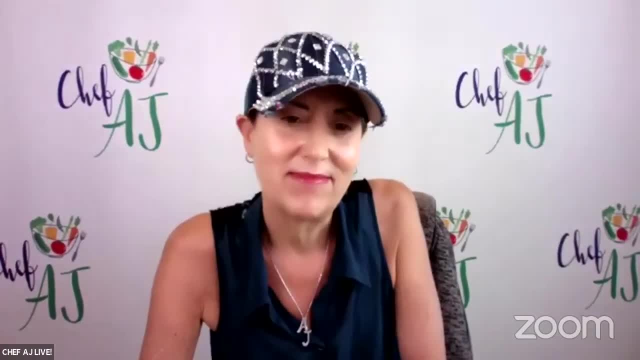 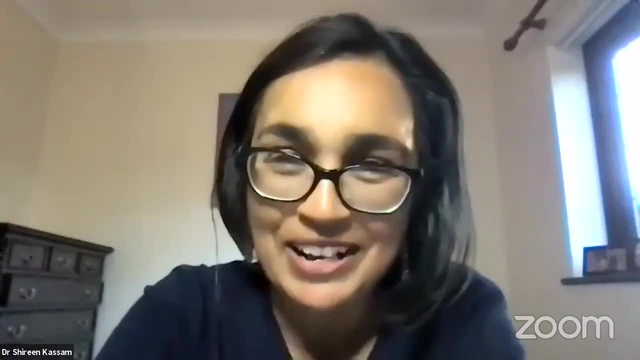 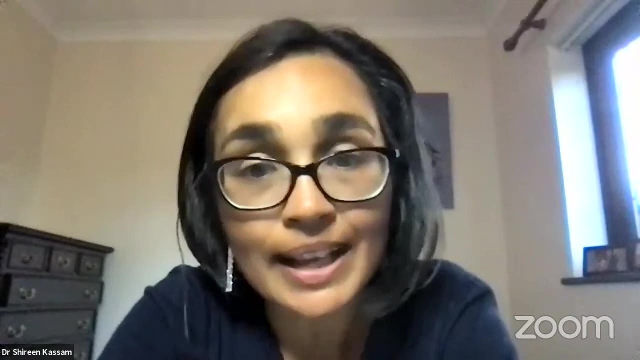 what's your opinion on this as a hematologist? yeah well, i mean, i have to say um. as a hematologist, i wasn't taught anything about um essential fatty acids, so it's what i've learned since um qualifying as a hematologist. i mean, i think we we need to aim to get um enough essential fatty acids from. the diet: flax seeds, walnuts, you know, chia seeds, hemp seeds, um, you know. whether we all need to take an epa dh8 supplement on a hundred percent plant-based diet is a question, um, but i think in this sort of nutritional doses, what you'd find in food, you're not going to have any adverse. 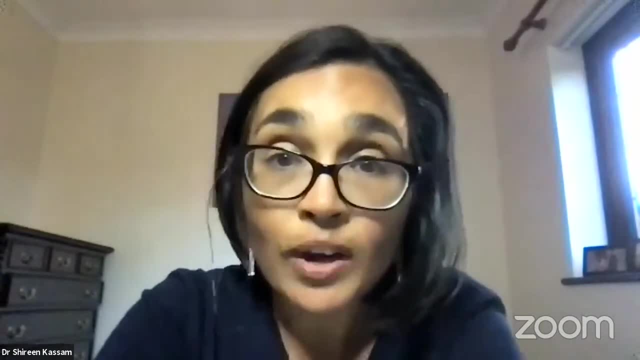 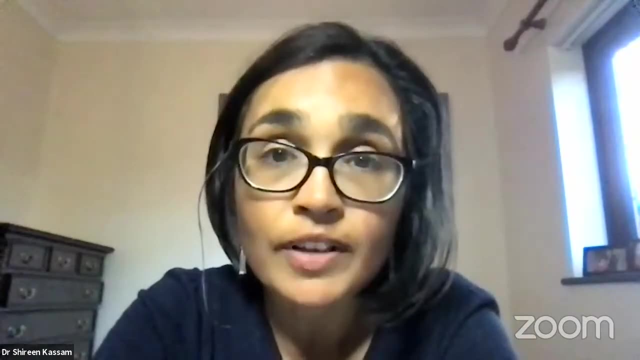 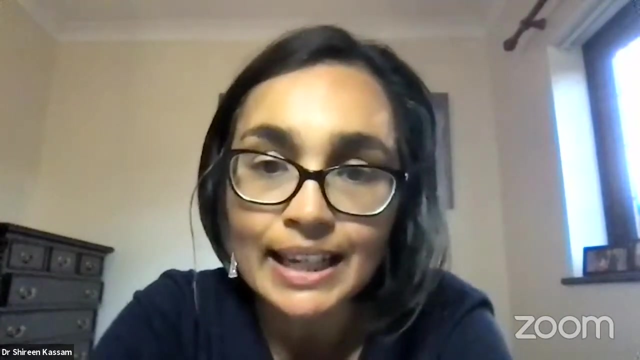 impacts on the blood clotting. but of course, you know, one of the reasons why it's thought that people who have heart disease and who do take supplements of dha epa may be able to get a small bit of advantage is because it- it you know, keeps the platelets less sticky. so yeah, it does impact that, but i don't think you're going to have adverse impacts because you're taking what you find in food and the doses present in food, um, as as your way of of obtaining these essential omega-3 fatty acids, and they're essential, so you do need to take them in some. 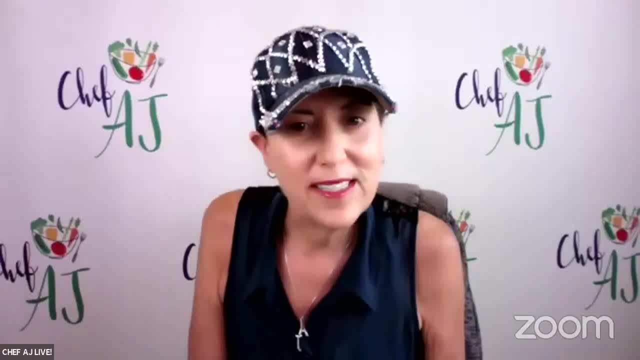 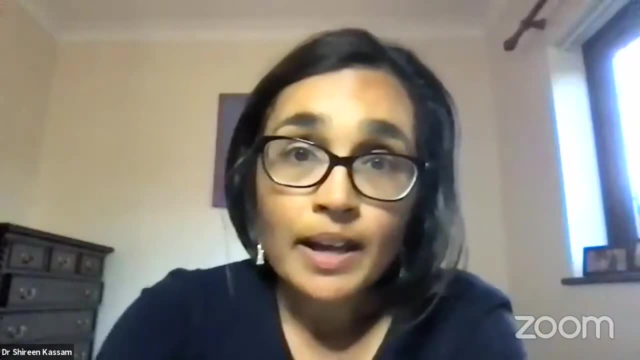 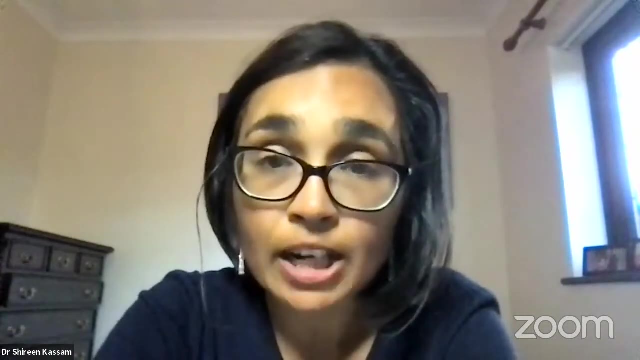 form or other right. thank you. uh, what is your insight on iv infusion versus pills to increase ferritin levels? yeah, i think this needs a person-centered approach really. i mean, i think there's no advantage in in terms of how quickly it brings up um the hemoglobin level, as long as you're. 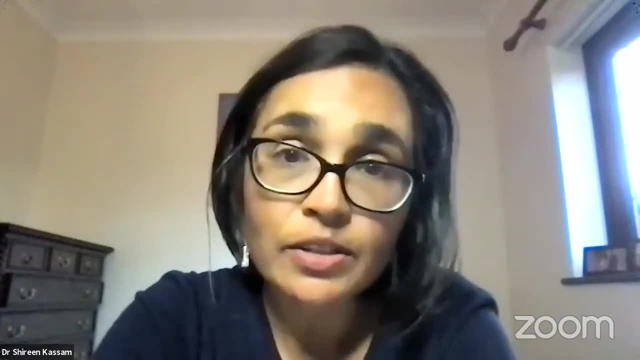 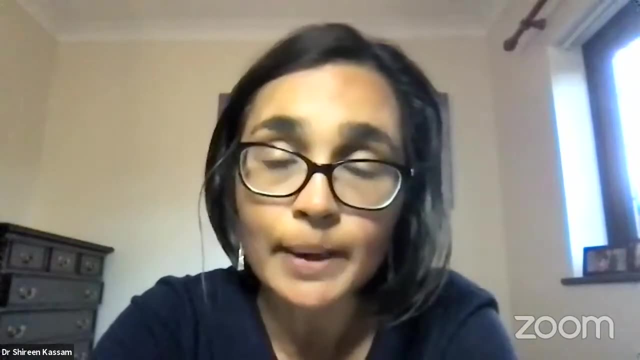 absorbing the ferritin or the ferrous sulfate or whatever form you're taking through the mouth. so obviously if you're taking an oral tablet, you need to digest it, absorb it and it needs to get to the right place. and obviously if you've got a gut issues that prevent you doing that, then maybe 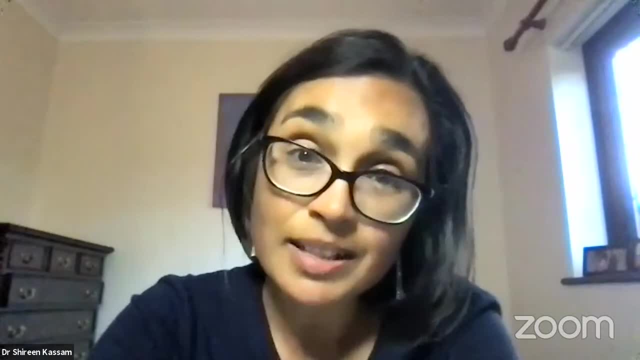 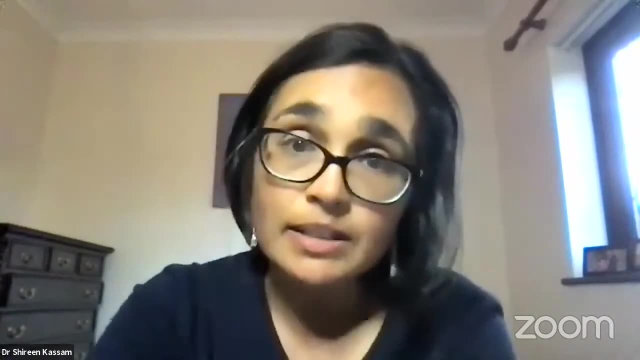 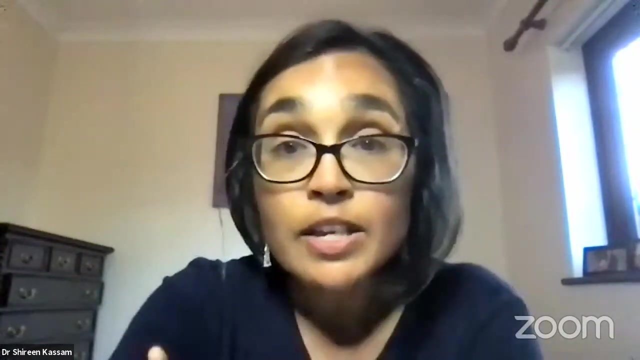 an iv form might be preferable for you. some people do get um adverse side effects, um, you know, with abdominal discomfort and constipation and things that makes taking a tablet intolerable. um, and then iv is an option, um, but i think overall if, if my preference would be tablets to start with. if it's not working, then to go over to iv. 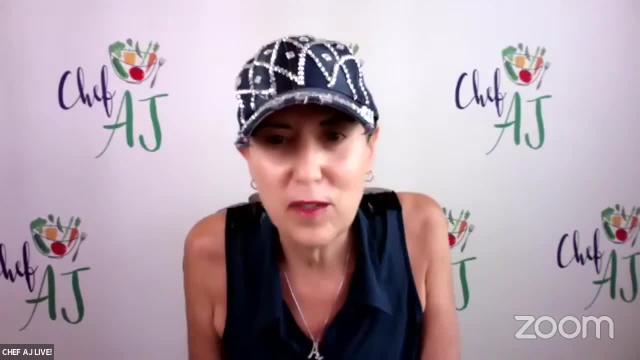 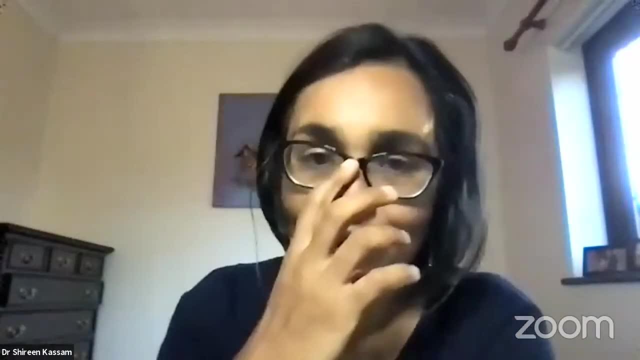 right. laurie says: what's your opinion on chemo versus whole plant foods and ultra nutrition for cancer treatment? that's a little bit of a controversial topic, isn't it? you don't want to answer anything. please feel free. no, i'm happy to answer, you know, i'm afraid. in my practice as a lymphoma doctor, once you have a diagnosis of lymphoma and if you need treatment- not every lymphoma needs treatment, but if you have a type that requires treatment there and then then i'm afraid um, you know, having conventional um chemotherapy type drugs or those. 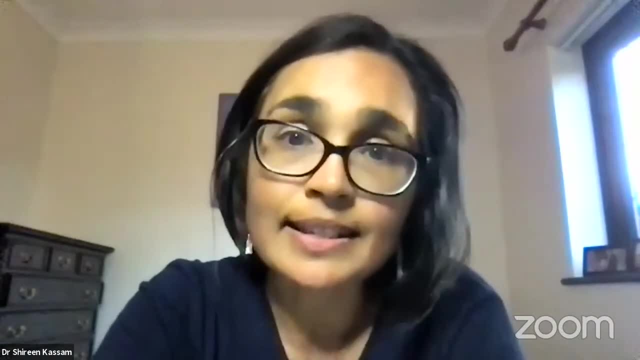 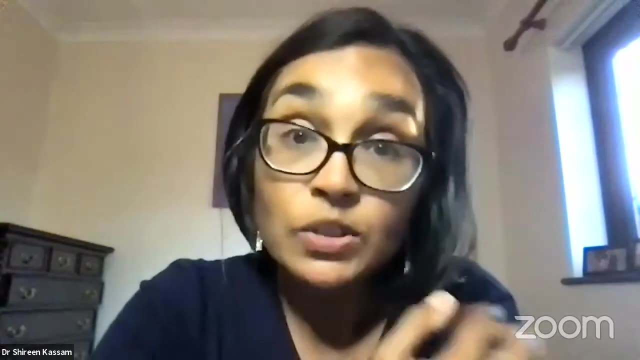 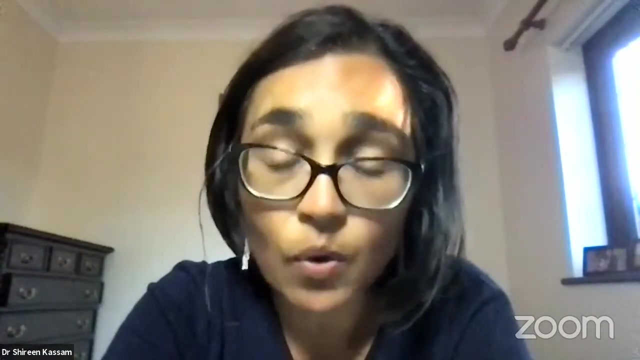 that directly impact that cancer is necessary, um, so i would never be advocating a diet approach um for um my sort of cancer. now, of course, you, your audience and you will all know about the study from dr dean ornish, um, and that was in early stages of prostate cancer, where 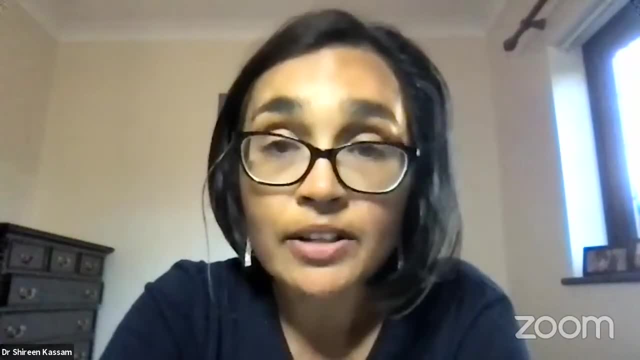 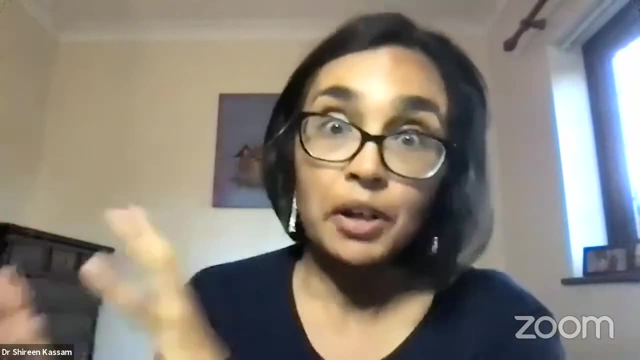 people didn't need conventional treatment and we're going to go um undergo just a watchful waiting. so i think if your cancer is able to have a watchful waiting period, then you know what's to lose, and dean ornish has shown that in prostate cancer you can um. cause arrest of the growth of the prostate cancer and sometimes even bring down the prostate specific antigen. so you know there are hundreds of cancers. just in my specialty there's over 40 different types of lymphoma, so it's very difficult to be so specific. but i do need to treat my 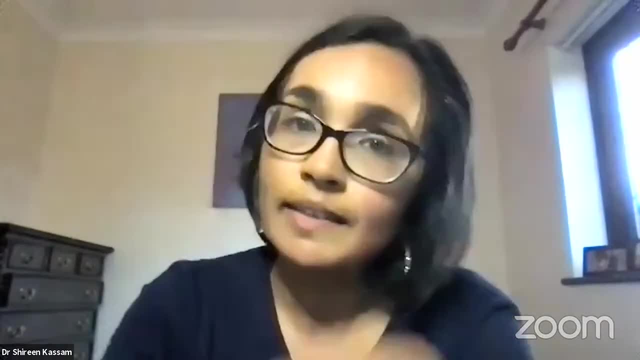 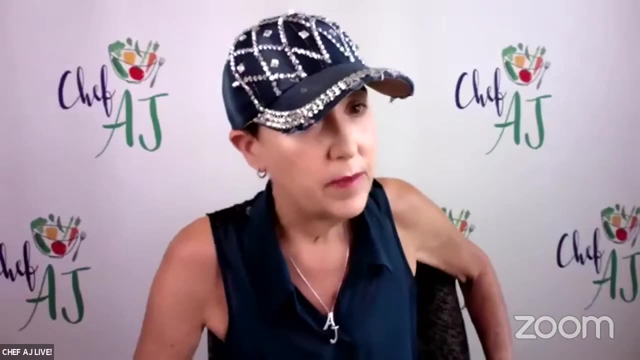 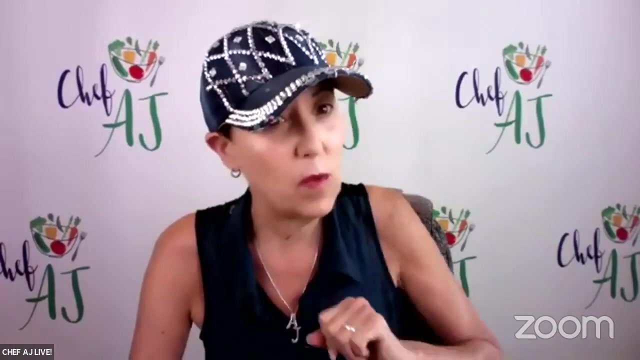 patients with conventional pharmaceutical medications. and then, on top of that, healthy nutrition lifestyle is so important. have you ever used or recommended therapeutic, medically supervised water, only fasting for these types of cancers? or have you heard about the work to the true north health center? because i think lymphoma was? 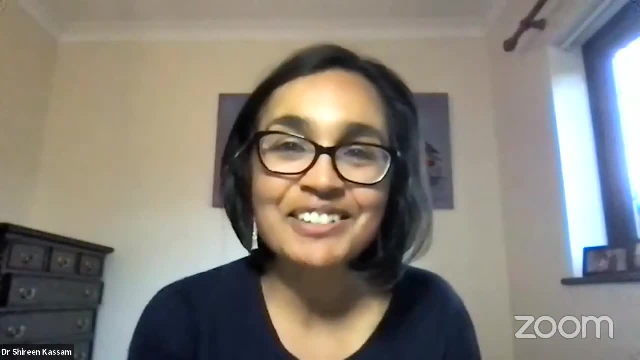 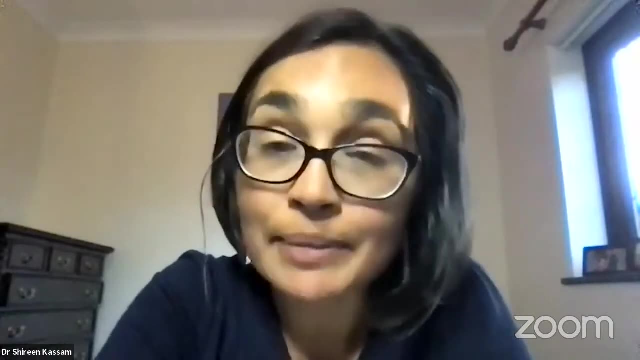 one of them that they actually wrote up. yeah, no, of course i. i've read michael clapper's paper and his co-authors. yeah, i mean it's very compelling. i've only come across that one um case, and that was an. that was an advanced stage of follicular lymphoma, where you do have time to watch, and 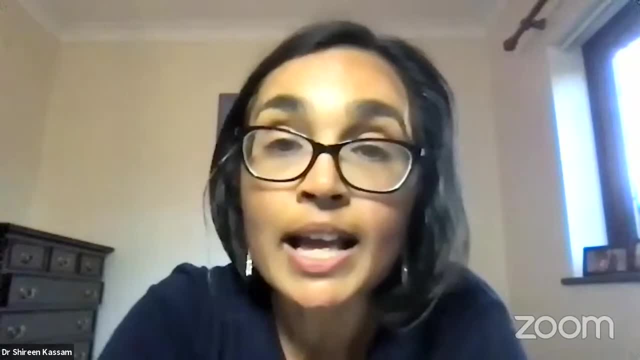 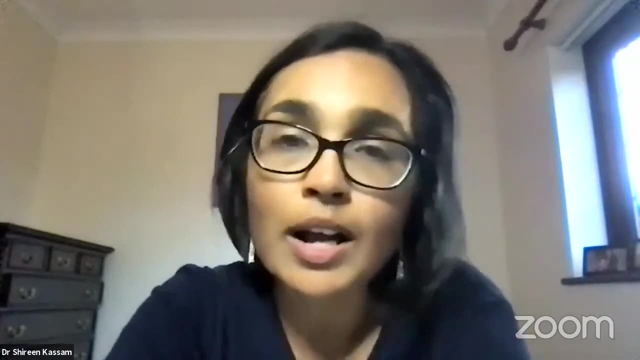 wait and you don't have to go in immediately because it's a slow growing um cancer um, and yeah, it's really compelling. but i think for me i would need more evidence and i'm i'm not sort of experienced in that sort of water fasting. um, i think we possibly have one um clinic in the. uk that does do that sort of thing, but i haven't seen any good data from there and i certainly haven't seen any large enough studies, and i think the area that will come up as being interesting and worth exploring further in due course is the sort of intermittent fasting alongside. 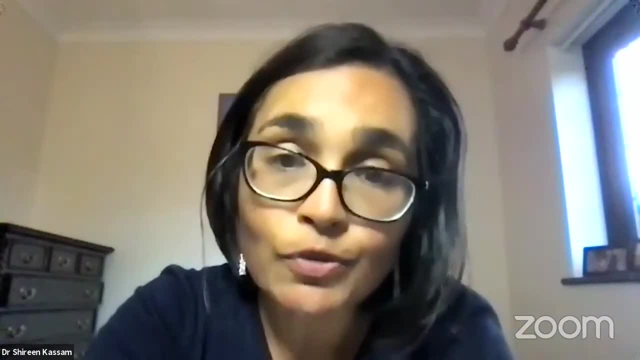 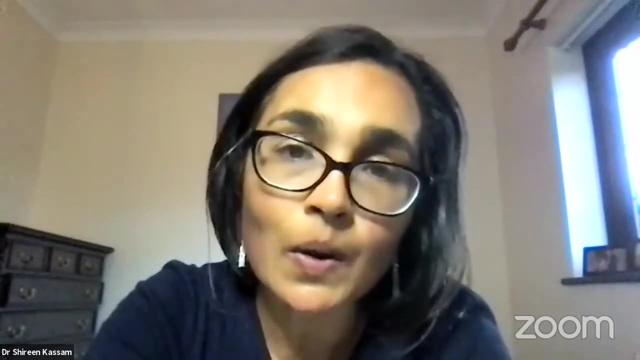 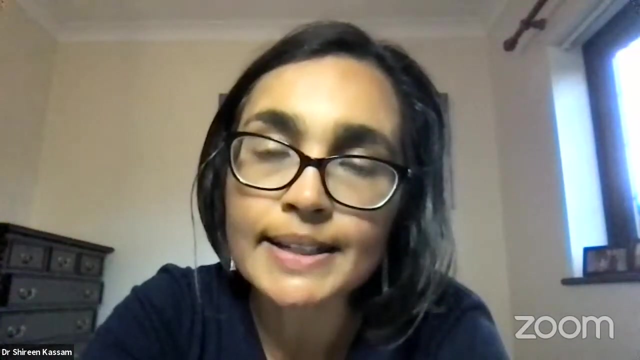 chemotherapy, the kind of volta longo approach, of the kind of five days of low calorie and plant based, and studies are starting to come up on that and i can see how that could um be beneficial. but i i would need much more data to start incorporating something like that and we're very highly regulated. 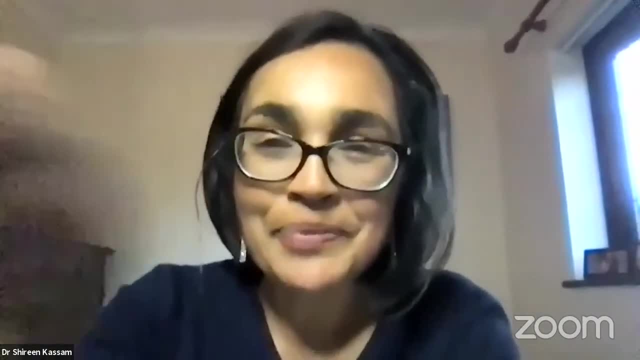 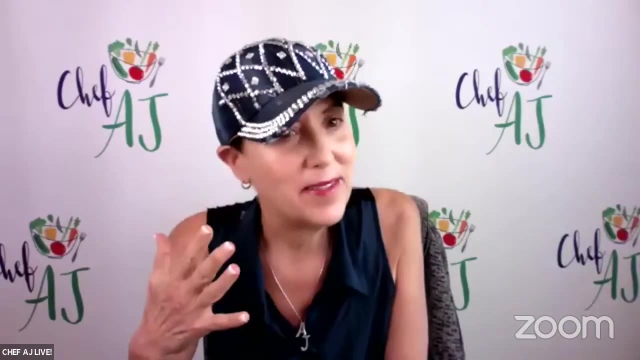 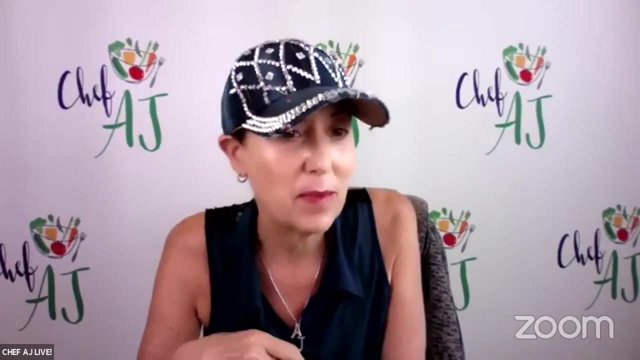 in the uk. i wouldn't be able to do that without um, um, the say-so of uh, the regulatory bodies, that's is. is plant-based becoming more popular in general in the uk, whether it's junk food, vegan or or ethical vegan? are you finding more and more people are adopting a vegan or a plant-based diet? 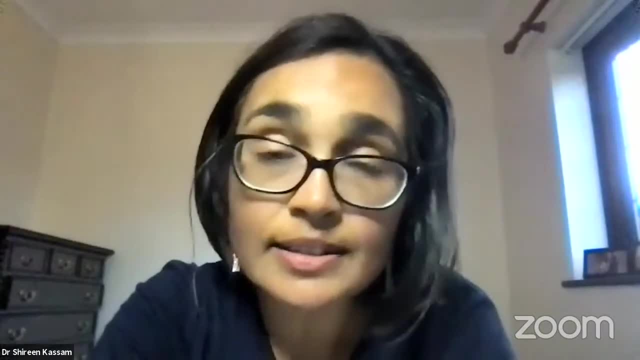 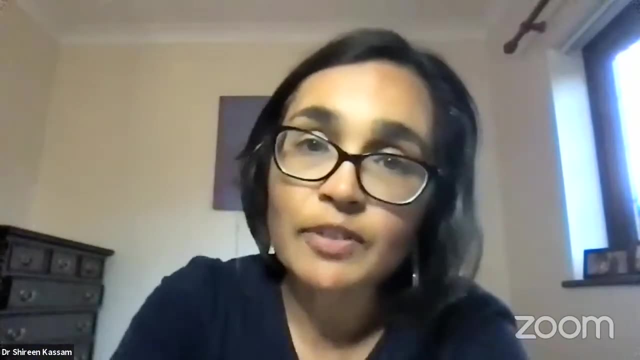 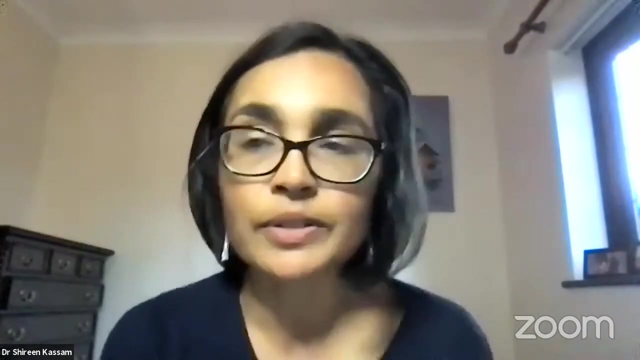 yes, i think it's becoming much more widely discussed and it's much more common to bump into doctors and healthcare professionals and, obviously, general public that are vegan or on that journey for plant-based um. certain things like plant-based milks have now become much more popular, you know. apparently a third of households are choosing plant milks, and that doesn't. 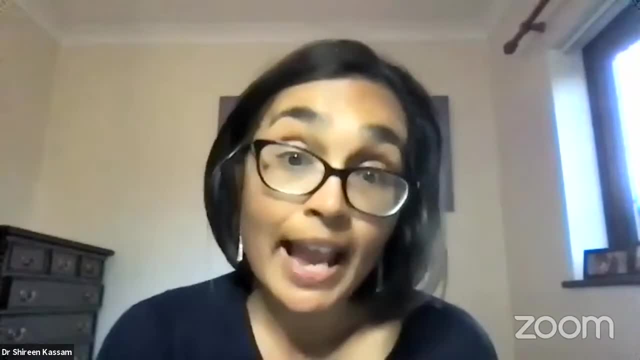 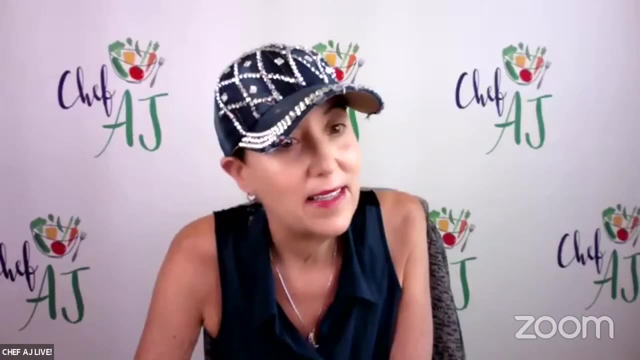 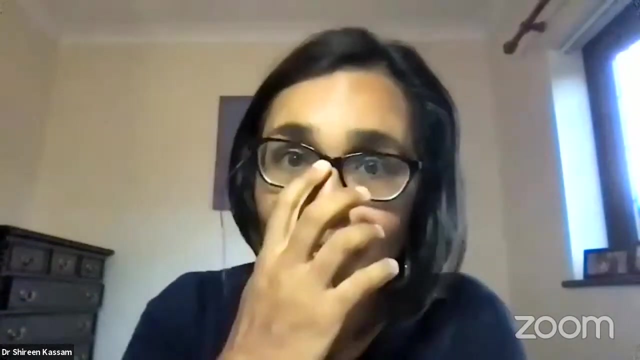 necessarily make them vegan, of course, but um, uh, yeah. so, yes, the numbers are slowly rising, not fast enough, but they they are rising nonetheless. what is the? the number of people who are using plant-based food, like at the hospitals? yes, well, that is an area that i really do want to try and impact and again, you know copying from: 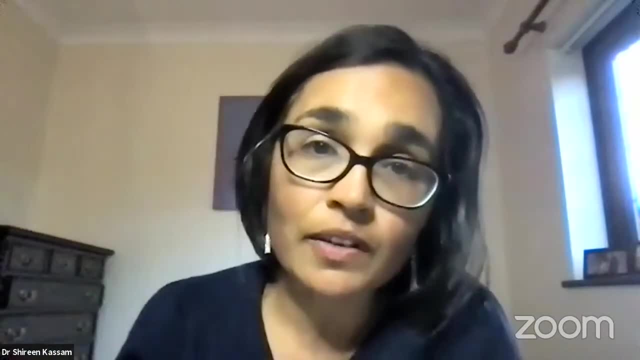 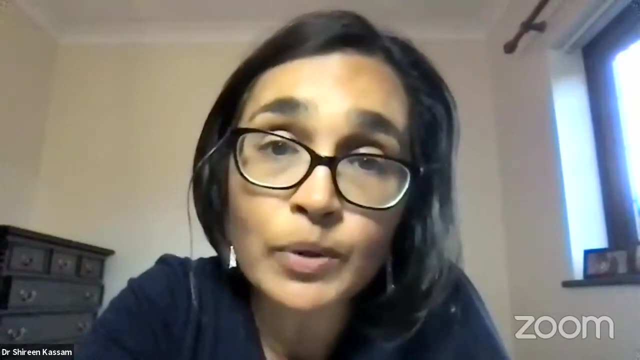 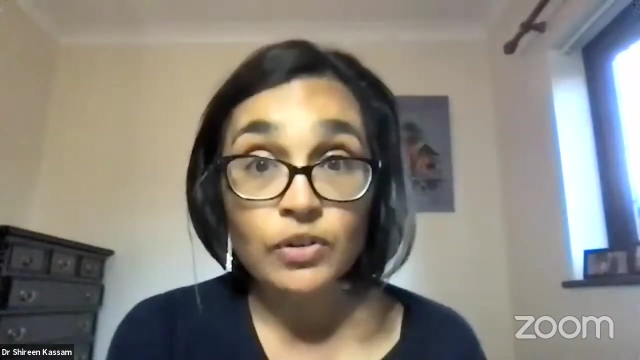 pcrm. we have been trying to campaign to to improve hospital foods, but really with a focus on um processed meats. but to answer your question, i think i actually think it's generally not too bad. um, we did a little survey of hospitals and um, all of the ones we surveyed had a vegan menu. 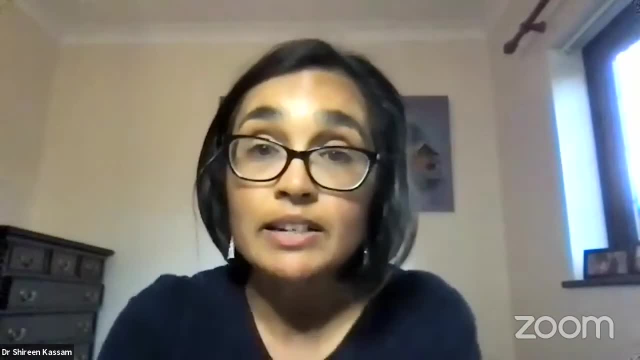 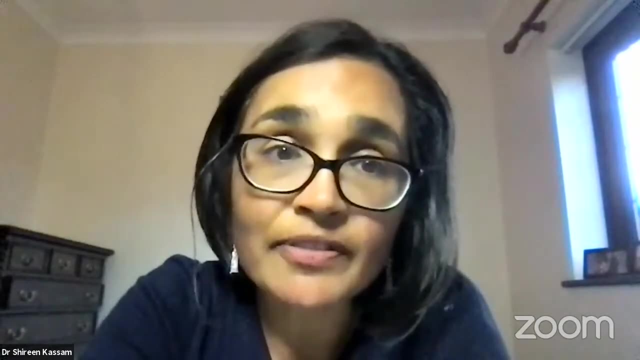 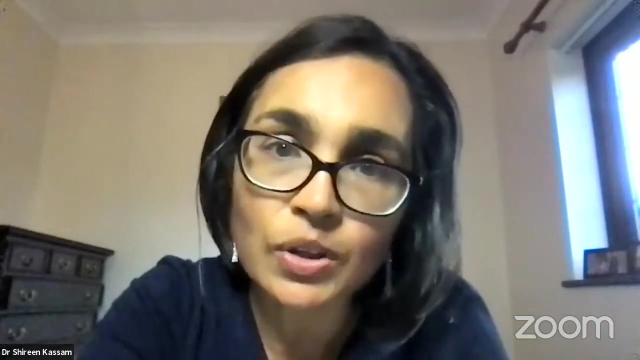 um, so vegan food is served. you know well, whole food- plant-based- is a different question, but you can certainly get a vegan meal in hospitals and I think you know it suffers from the fact that you can probably choose anything and everything and people don't necessarily make those healthy choices and in our sort of staff canteen certainly. 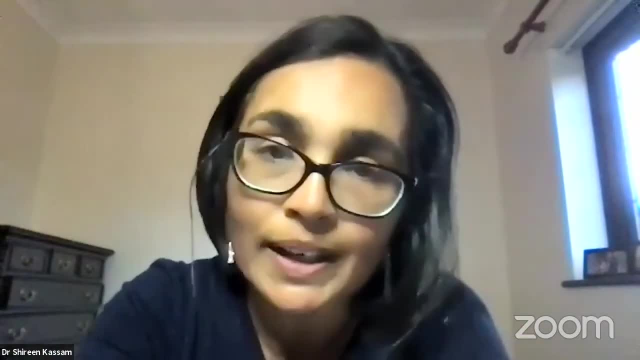 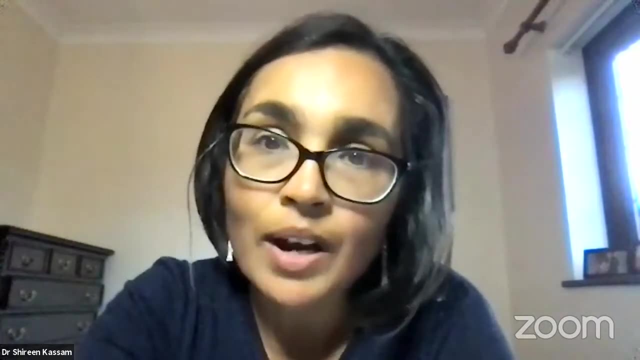 in my hospital you can have a bacon sausage fry up in the mornings for your breakfast, if that's what you choose to do. we have retail outlets that are serving, obviously you know, processed meats and things, so I really do want to try and influence that something our organization does. 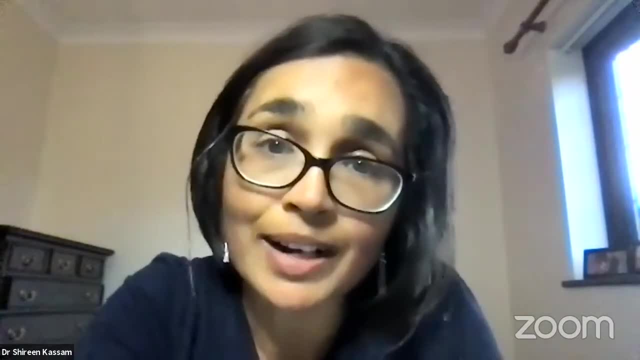 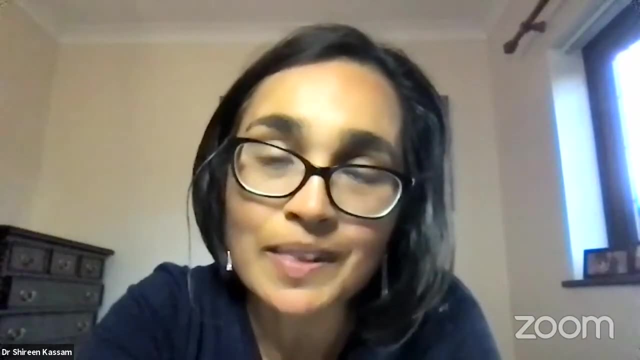 and for. actually for the first time this year in my hospital, we were allowed to run the international campaign no meat may, and so we got permission from all the execs to be able to launch that with the staff, and we had about 60 people sign up and join our whatsapp group and cook alongs. 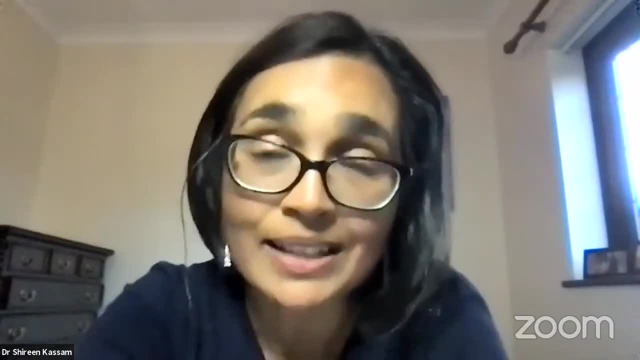 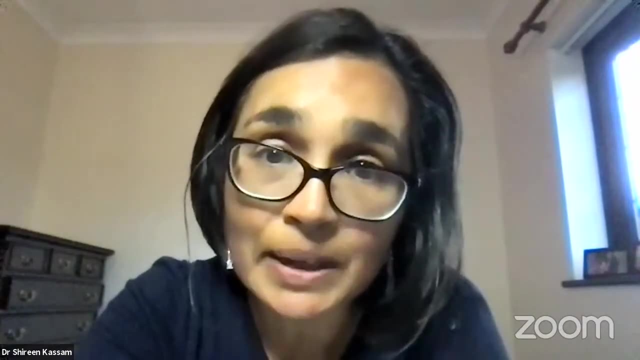 and things, and so that was the really first time that I felt like in my workplace it was okay to be sort of talking about that and getting people on board and, to be honest, that's been mainly driven by the sustainability agenda. so the NHS in the UK has to become carbon neutral or carbon zero by 2030. 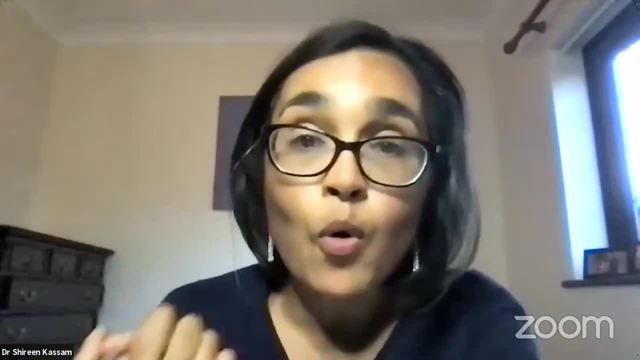 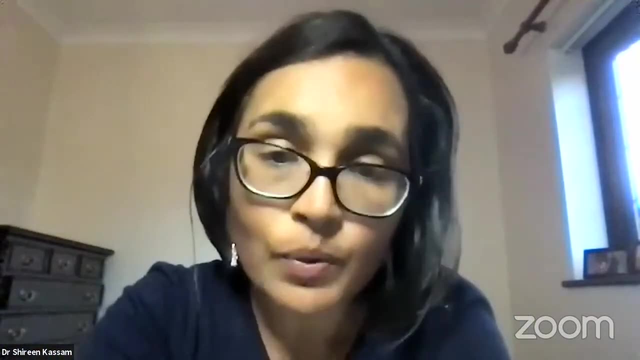 or something. so everyone's you know more, more concerned about the climate, as they should be, and are slowly, slowly making the connection with the food environment as well. so we are now in conversation with our hospital team about trying to remove processed meat, then red meat and then 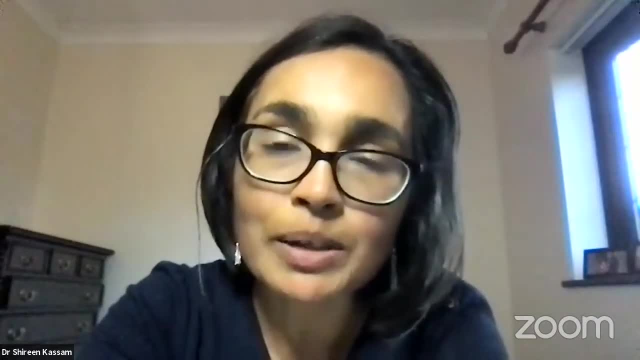 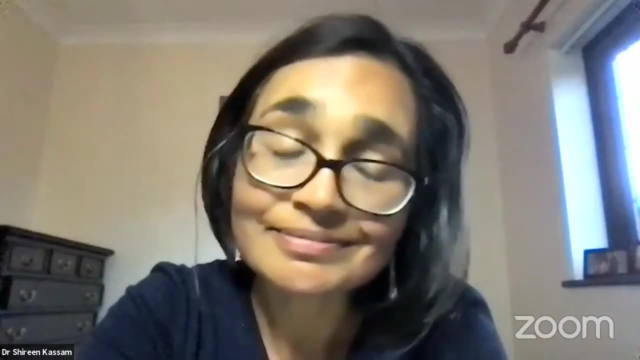 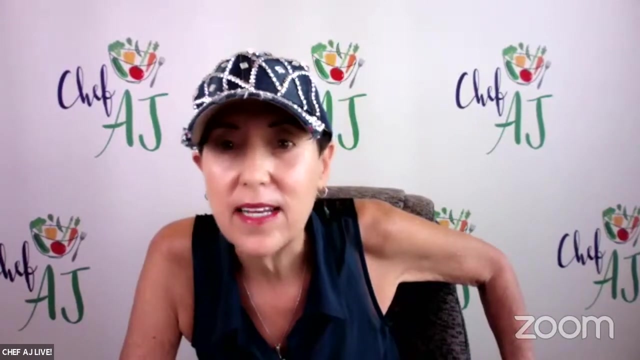 hopefully getting some dairy alternatives as sort of more commonplace. Yeah, the wheels turns slowly, don't they? They really do. Yeah, I've been doing this 44 years and I'm like I just can't believe it. I can't believe that people are still eating meat. so let's see. I just saw a question from Evelyn. why do people get acquired? 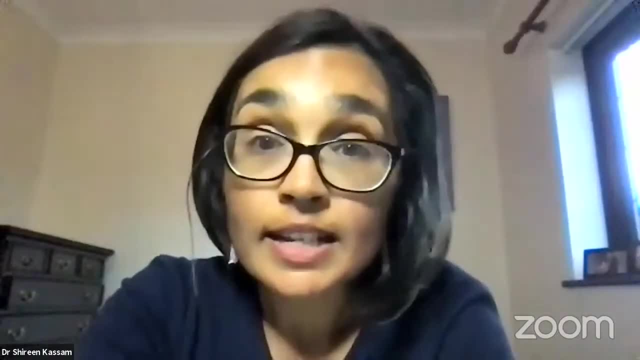 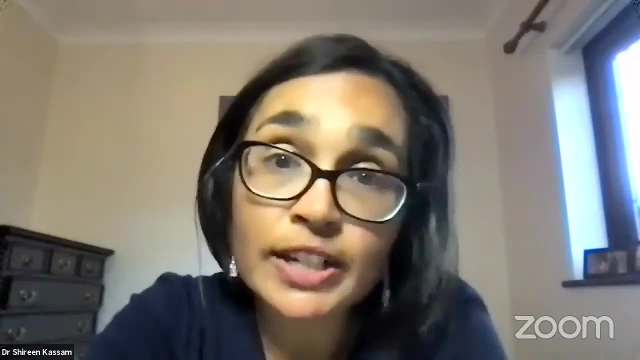 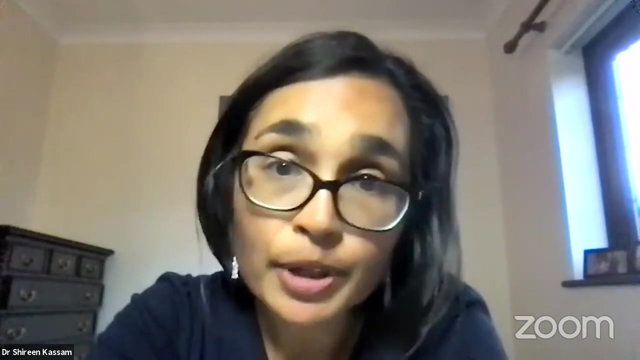 haemophilia? Yeah well, so that's an interesting question. I'll caveat it, with it not being my direct specialty, but it's essentially an autoimmune process. so it sort of comes down to: why do people make antibodies against their own proteins and cells and for acquired haemophilia, you're making an antibody against your clotting. 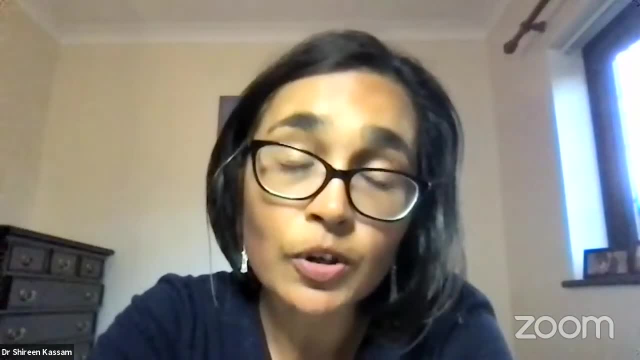 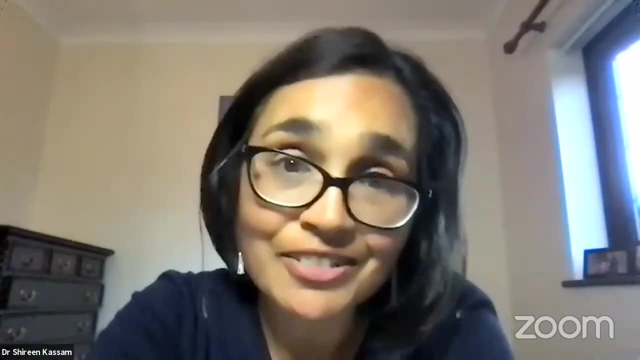 factor and therefore it can't work to clot your, your blood. it's difficult to know why. I mean you know it's always going to be a combination of genetics, environment, lifestyle. I haven't read anything about lifestyle factors on acquired haemophilia. it's very niche, Wow, interesting. 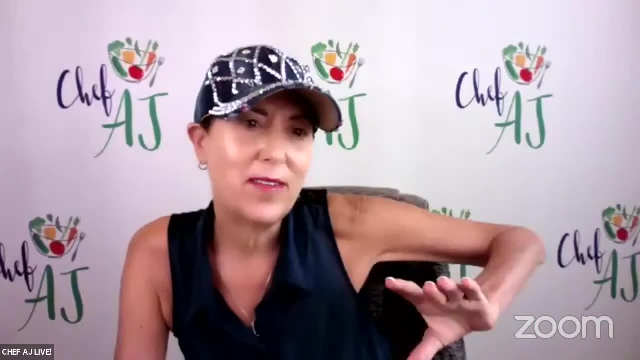 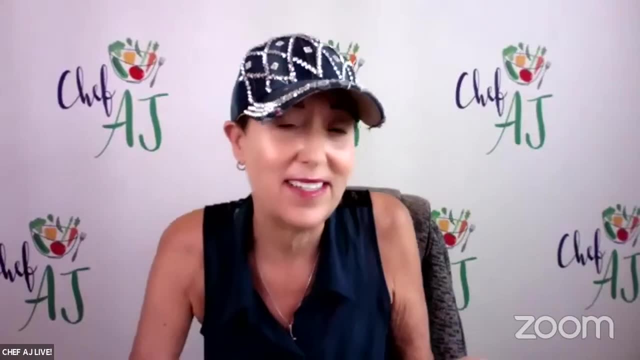 let's see. you know, did you ever think about doing what you are doing in your country, just like being the ambassador, just going to every country and just Just because it seems like you know how to do it? you've done it. you know the telehealth. 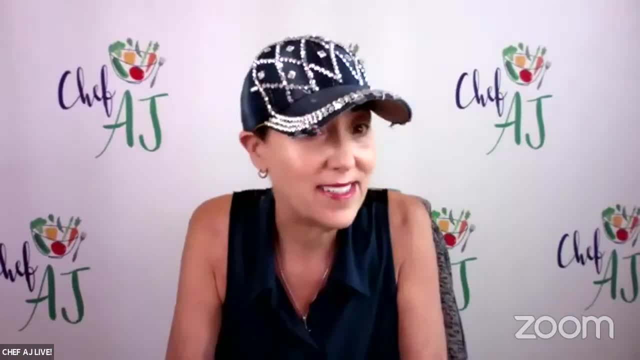 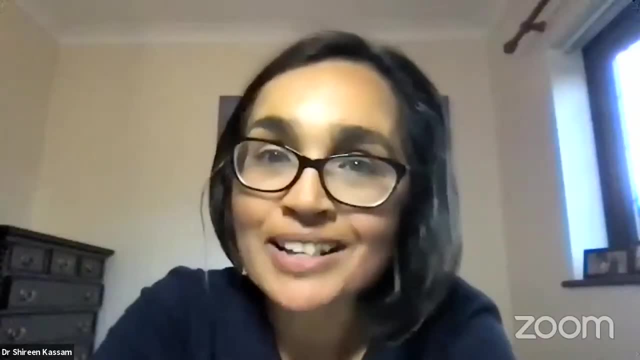 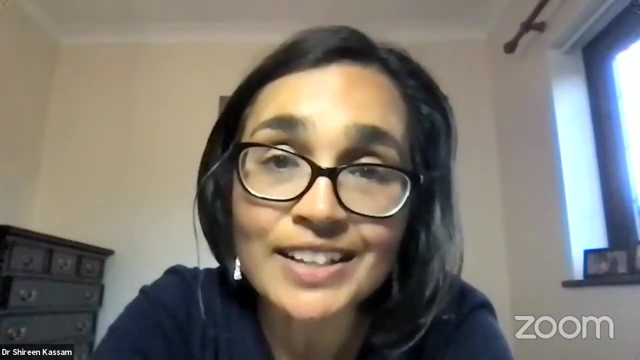 the, the, your version of PCRM, the course, your version maybe of the colon can. maybe you could just go to like every country and just set this up. That would be great. but I think actually others are doing it. so you'll know, Physicians Association for Nutrition out of Germany, and they're setting up little branches. I've already mentioned Doctors. 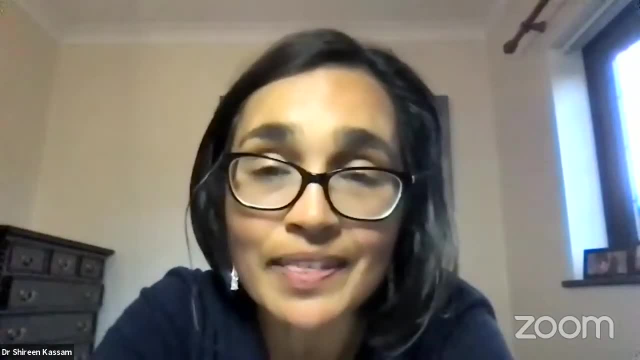 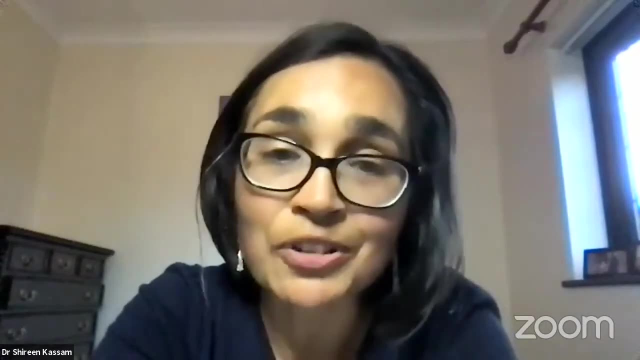 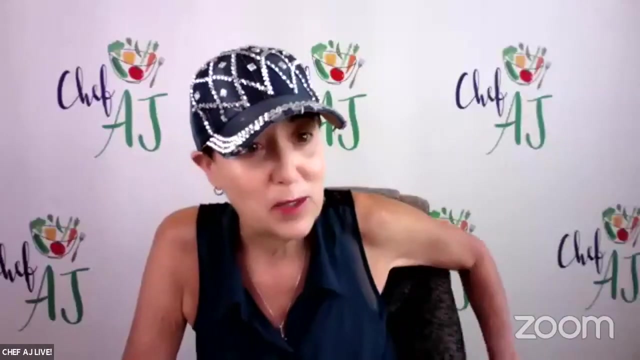 for Nutrition in Australia and New Zealand working together, so I'm connected with them. you've already met the Indian group, but I'm connected with And so I think people are. I think the main thing is to network, to not duplicate resources, to share our expertise, and hopefully we're managing to do that. It's amazing that the treasures I'm finding 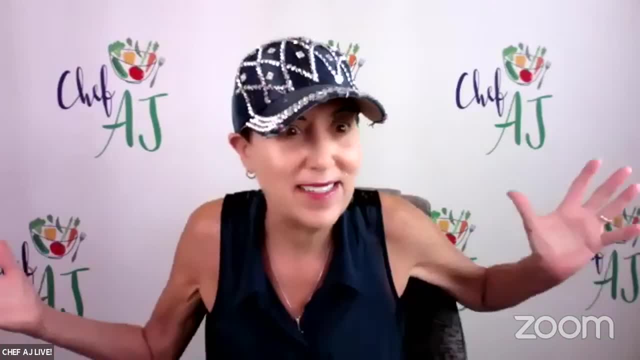 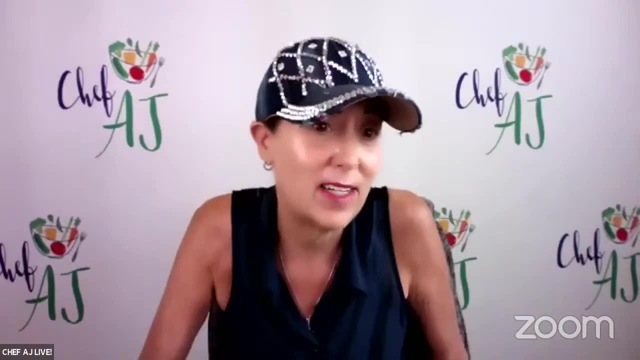 I mean, who knew there was this whole organization of Indian? I mean there's Indian doctors and they're fabulous. I mean people need to know because, who knows, they could stumble across a video if they could be in that country or that city. you know, Yeah, absolutely Yeah. so yeah, I've heard this. 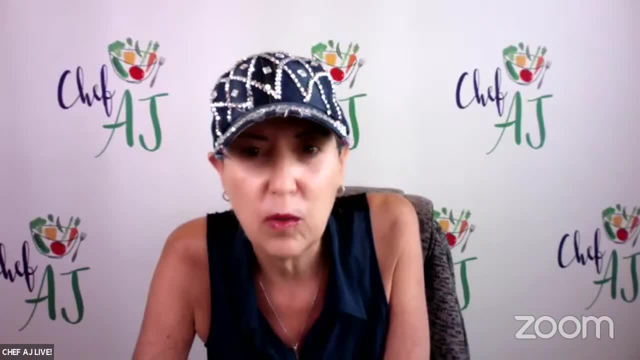 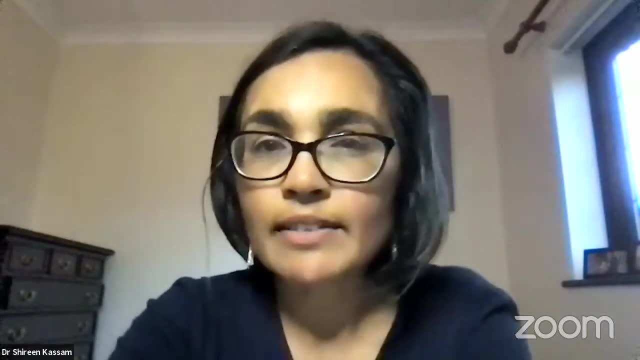 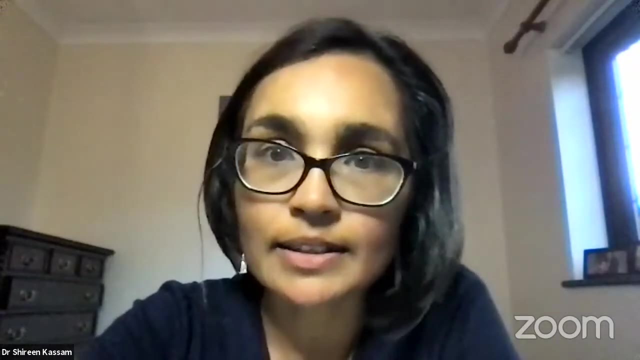 before a question from Sharon: Do vegans tend to have lower white blood cell counts and why? Yeah, interesting question, and the biggest study I've seen is actually from the UK Biobank. They're producing quite a lot of good data. so do look up just on the internet- UK Biobank- and there's lots. 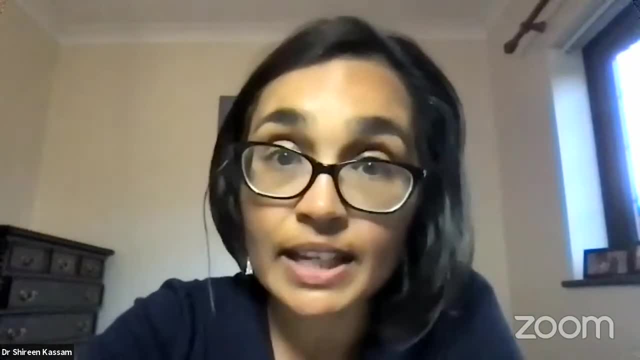 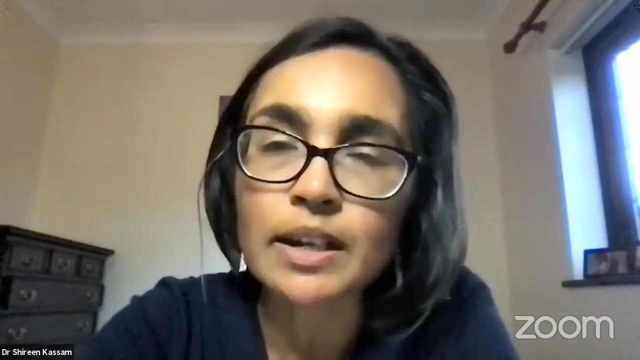 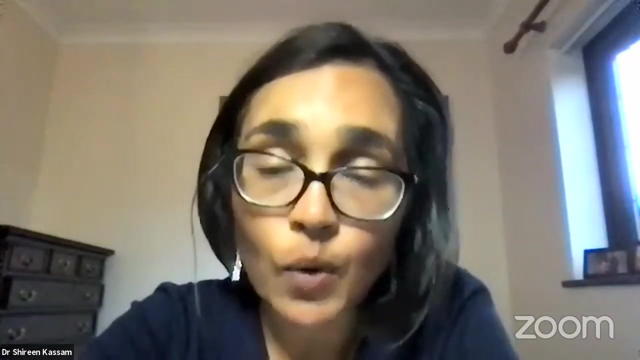 of good studies there. They've got a sizable number of vegans and vegetarians in that group- mainly vegetarians, to be honest- and there was a big paper- I think it was 2019- where they looked at blood counts specifically in different diets. So they did show a slightly lower white cell count, platelet count, in vegans, and but it was still within. 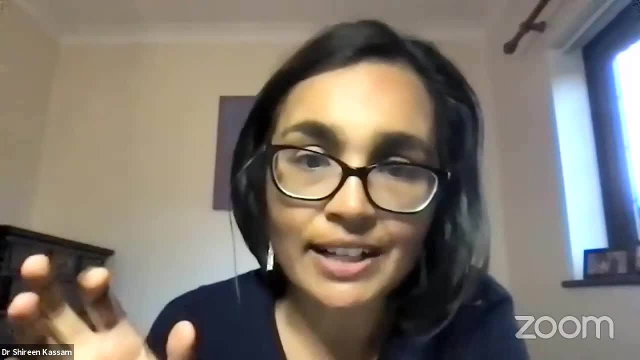 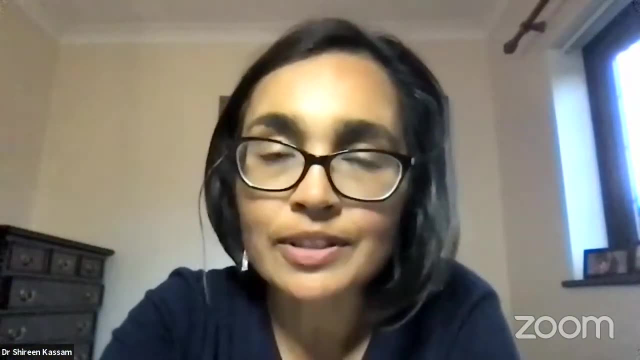 the normal range. so you know clearly, you can statistically find a difference between numbers, but it doesn't mean it's abnormal. so I don't think people should worry that they're going to be outside what we call the normal range. and yeah, I mean, I think that the theory is that because 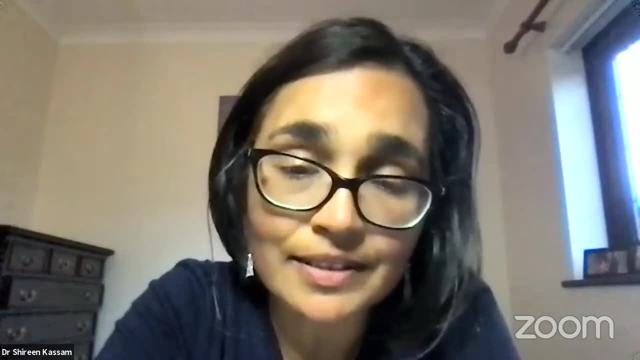 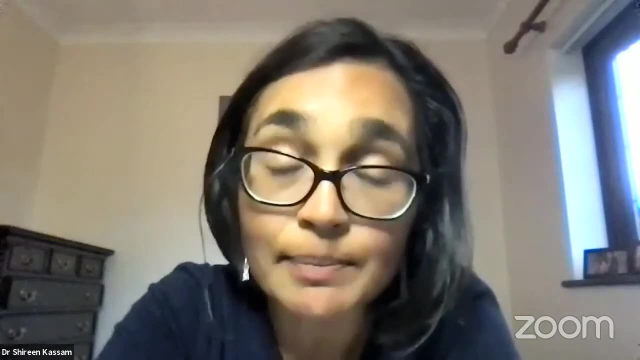 a vegan diet is anti-inflammatory and the white cell counts- oh, the white cell counts are going to be white cells. are there sort of fighting infection, inflammation, et cetera? And you know, if you're on an anti-inflammatory diet, maybe you will see a slight reduction in your white count and your 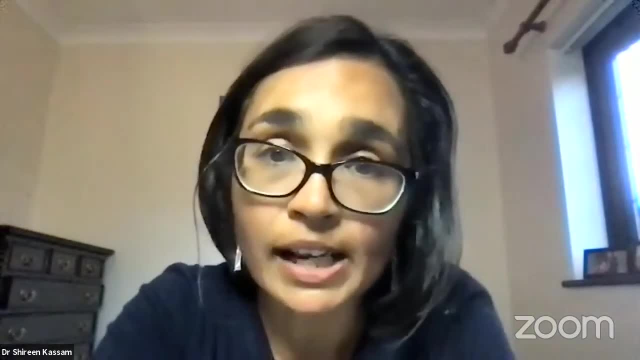 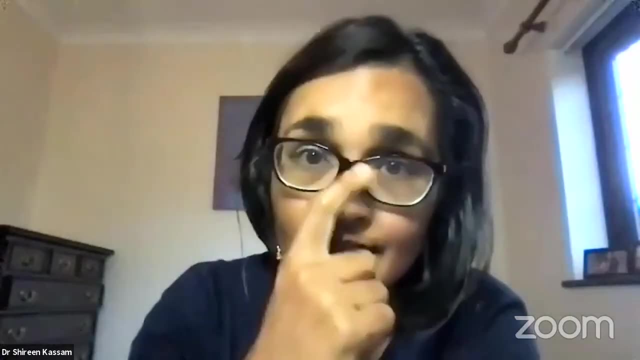 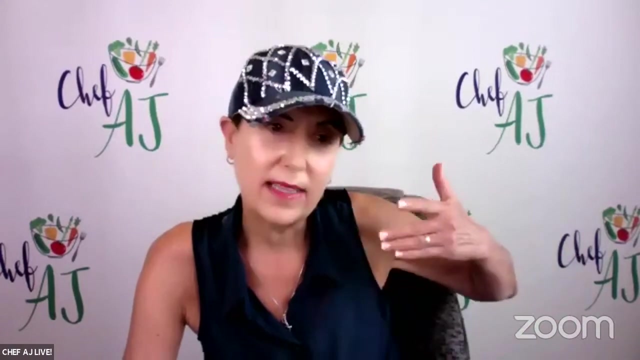 neutrophil count, But, as I say, still within the accepted normal range. Right, But it's not nothing we should worry about, Oh no, no, quite the opposite. I think that the theoretical reasons why it's lower is a good one. Nice, You know, it's really funny. We have this system where I 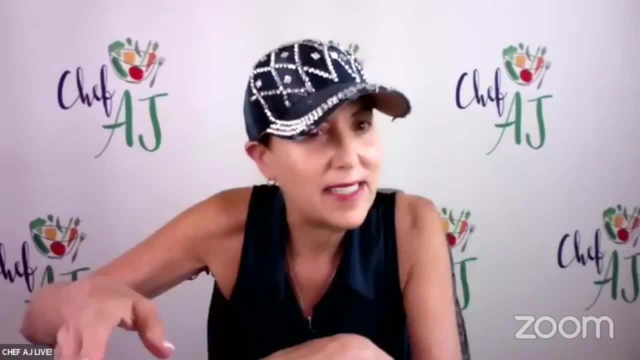 live now and it's like a my chart, it's like you know all the information, So you can contact your doctor and all your results are there. It makes it easy now for- and I you know I had to. 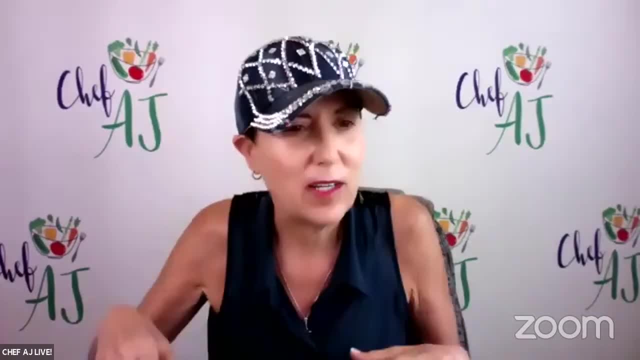 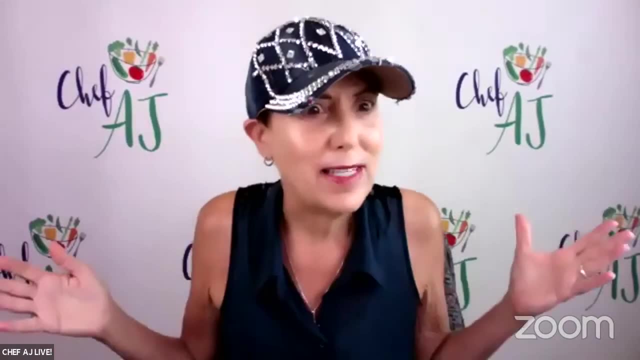 update it today. And I was they were saying: is this information accurate? Like your my allergies. I have a lot of drug allergies, for example, And so when they listed my medical conditions or the past ones, they listed vegan as if that's like a condition. and I'm cracking up and I'm thinking. 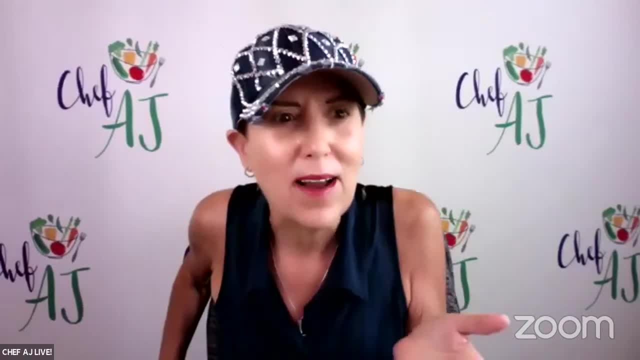 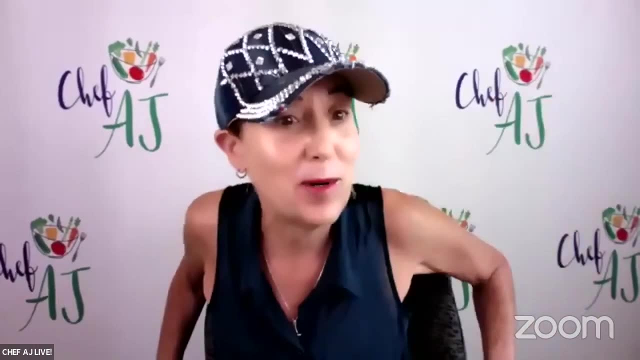 like I want to keep it on there, just so they know I'm vegan. but why is that a medical condition? That's like a good thing. That is hilarious that there's so few vegans that this is considered a medical condition, that if you're vegan, you better put that in the chart. It's hilarious, isn't it. 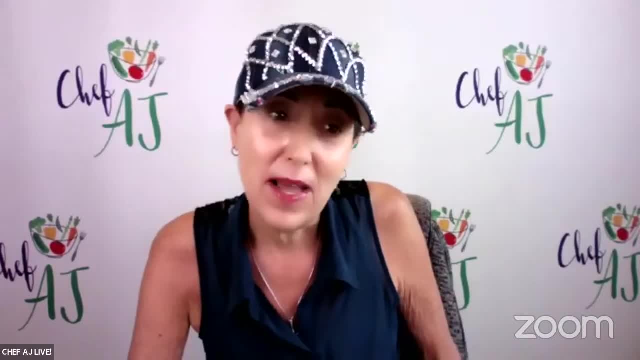 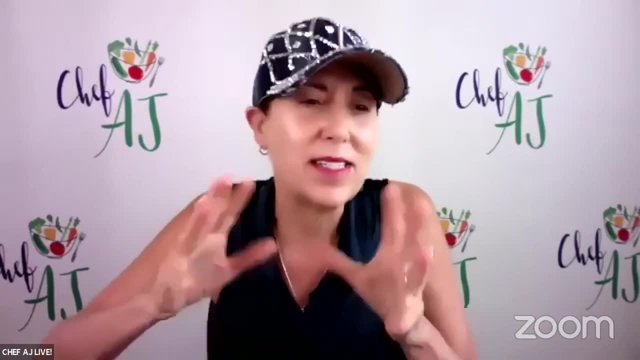 I just think that is so funny. I have not, unfortunately, I've met one vegan doctor here since I moved from LA three years ago And he's, he's not, he's. I can't see him because he's like like a teacher of doctors, He does precepting and he and so that's it, Like if. 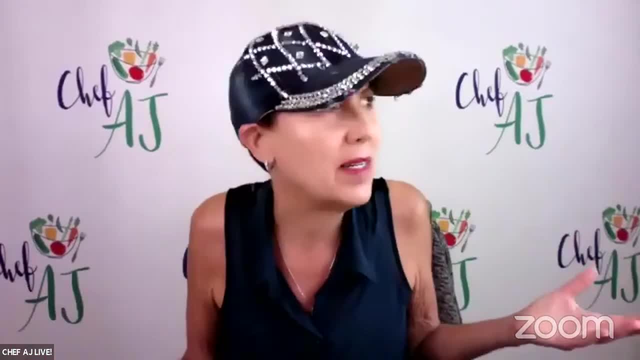 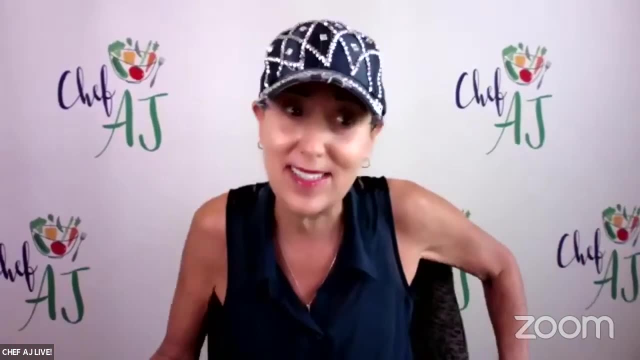 there's another one, I haven't found them. So, whereas in LA it was pretty common- cardiologist, internal medicine doctors, dentists, veterinarians- everybody was vegan, My hairdresser here in the desert, it's like, I don't know. it's very strange. So anyway, that's funny. So do you have? 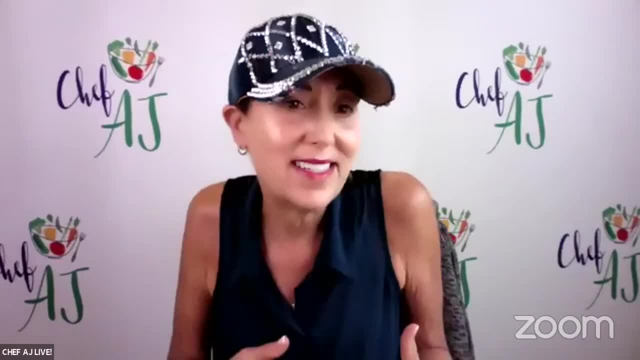 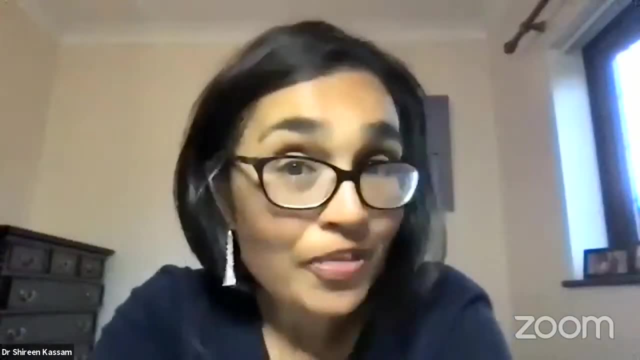 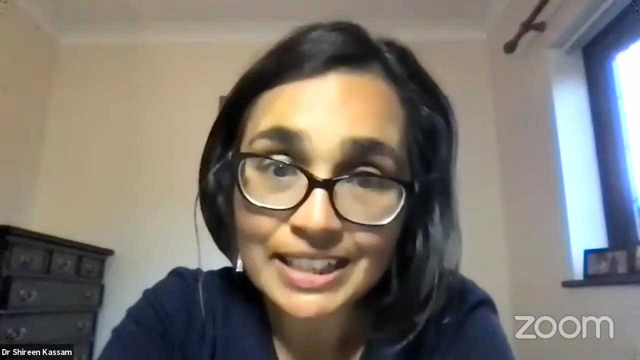 any like success stories of patients that you maybe work with that have improved their diet and either felt better or overcome their diseases. Well, I mean not their cancer specifically, because, as I say, I treat with conventional, So what I see is those other lifestyle conditions. 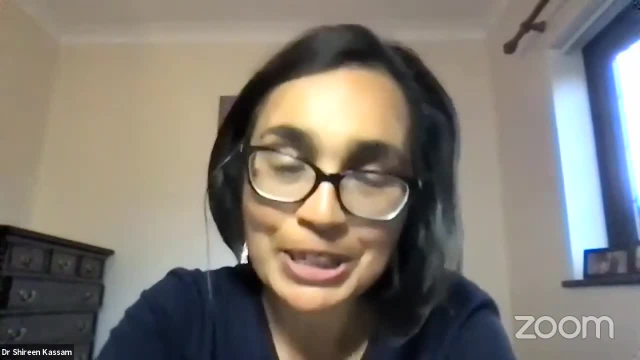 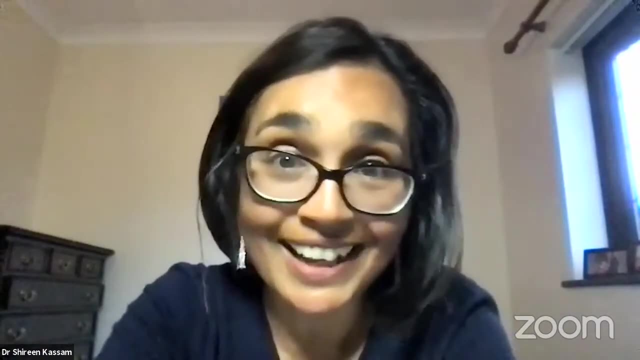 improving. So weight loss, blood pressure is coming down, blood cholesterol, you know, blood sugar is getting better. So so those are the things that are on offer really, once you see me in the cancer clinic, in, in, in inverted commas. So yeah, just the everyday primary care. 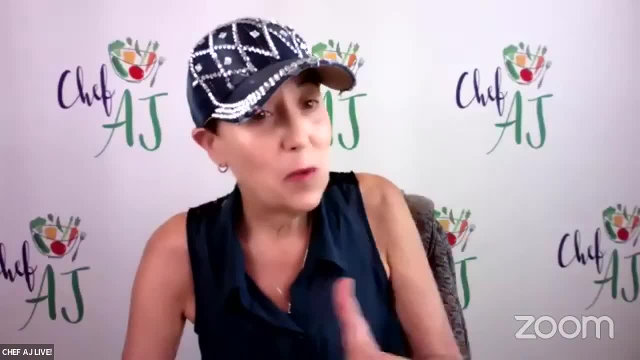 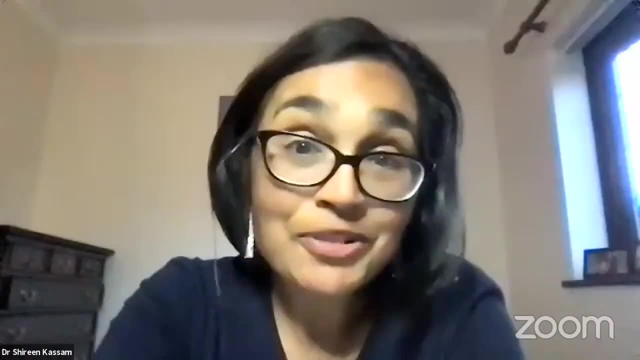 stuff, Nice Well, anything else you want to share with our audience either, about your practice, the courses, your, your, your own particular lifestyle? Yeah well, no, just that you know. I just hope that your audience now know that there are advocates in the. 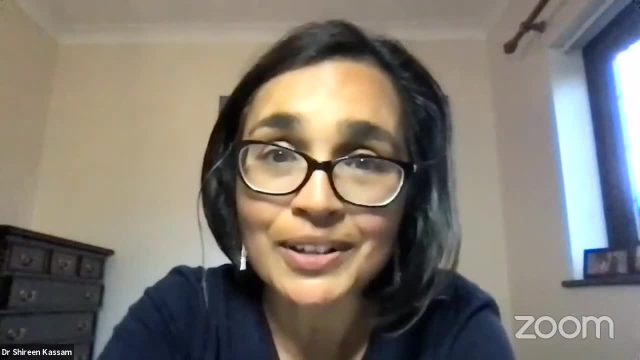 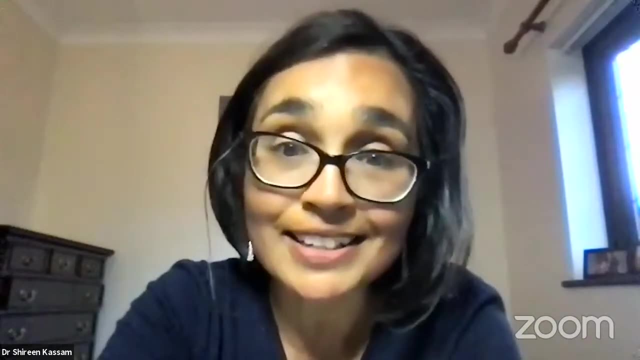 we're working really hard to try and, you know, bring all this knowledge and you know information to the UK public and, you know, spread the message for us and share our resources. We've got some amazing fact sheets and articles and webinars and all sorts on our website. 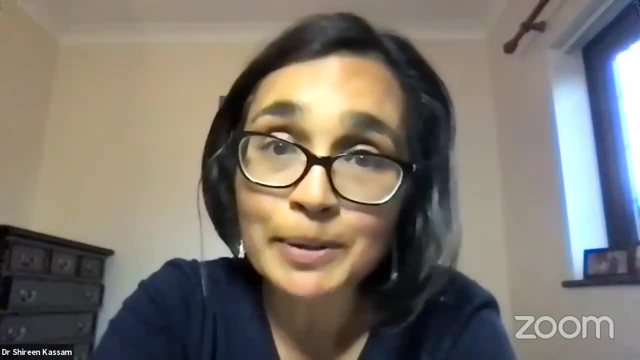 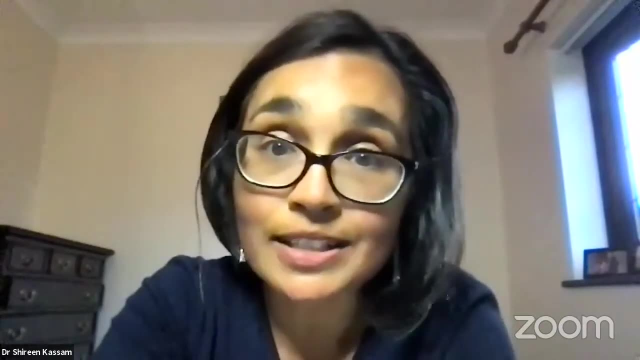 that are mostly free to access. And if you come across people in the UK who are looking to connect, to then connect with like-minded health professionals, then then we're here And then, of course, all your audience are welcome to take the course. And if they've got patients, 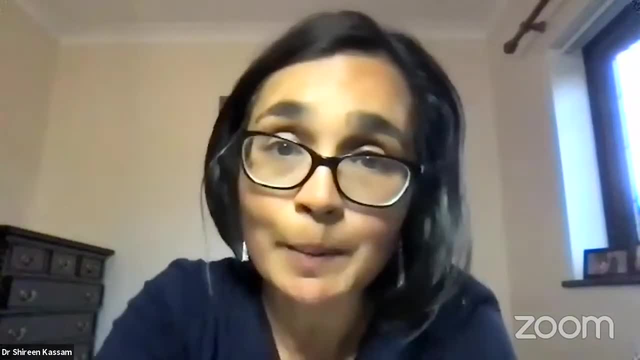 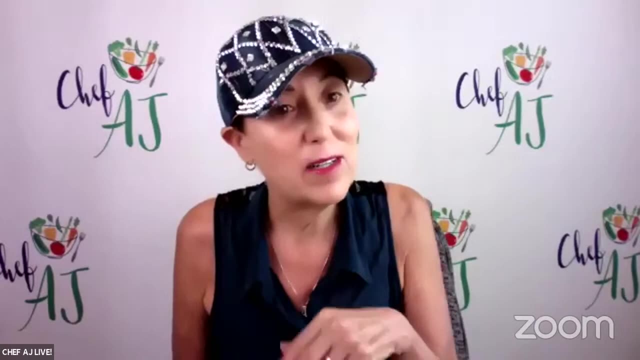 clients or friends or family who need a bit of extra help. we've got plant-based health online as well. That's accessible, That's terrific, And all the links are in the show notes, So people can everything. we talked about the course, the telehealth and the. there was three things, and